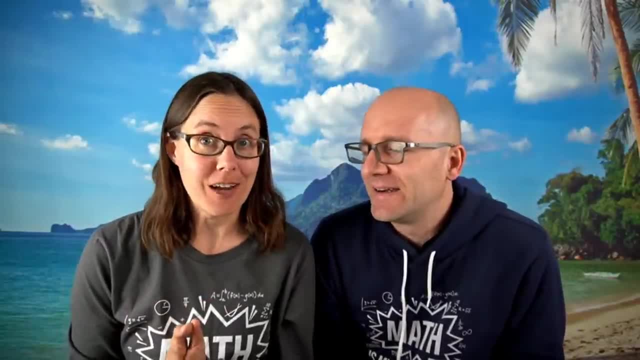 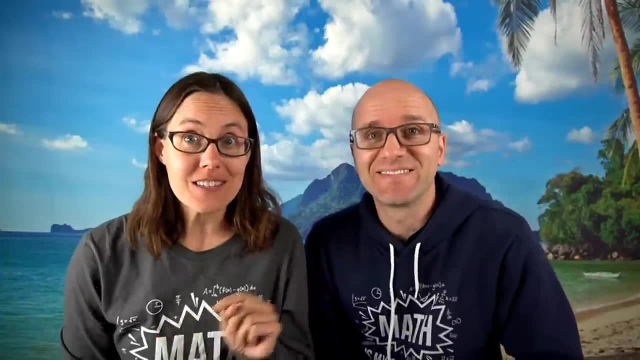 as well. There are a couple important tools that will help you identifying rocks. One is to recognize how hard the rock is. We'll talk about mineral hardness in a minute. The other is to be able to look closely- and a magnifying glass can help- and see. are there visible crystals? 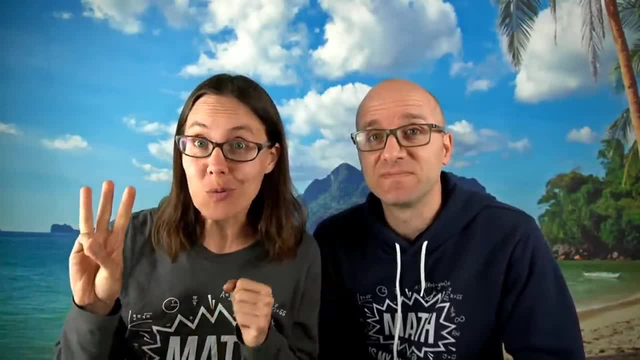 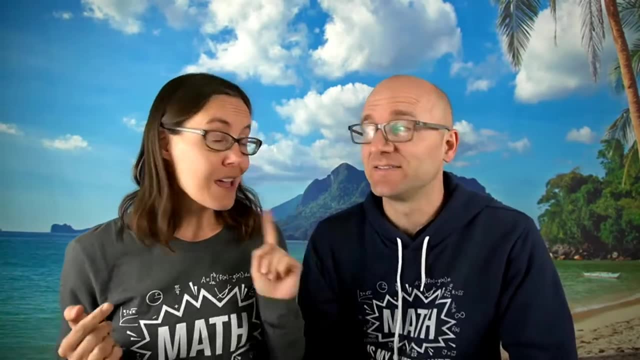 Are there layers? Those three things are clues that can really help you identify a rock. And then the fourth one, which is also very important, is: where did the rock come from? Because location can be really helpful. But before we dive into those processes, let's 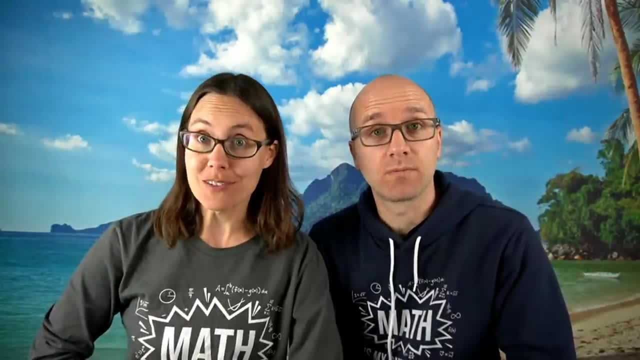 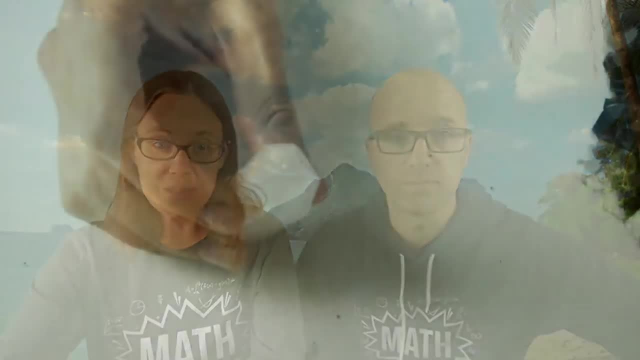 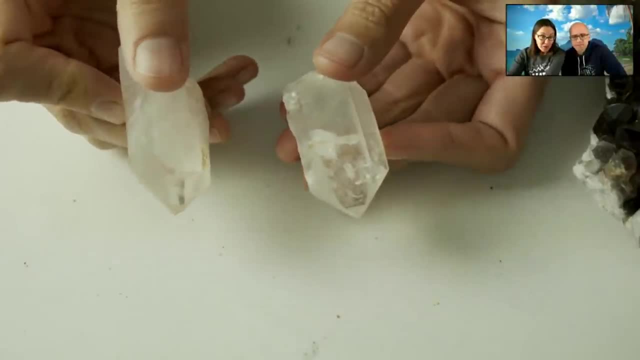 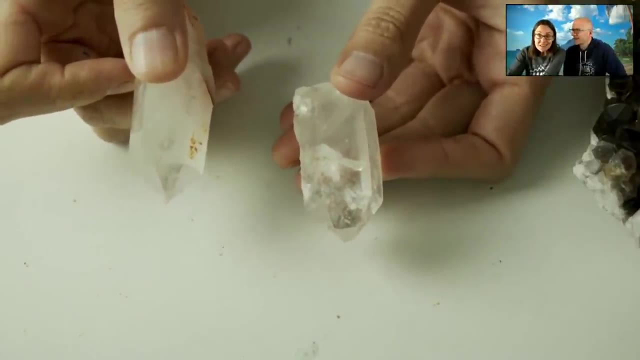 Wow, Kind of like. It's like a crystal, It's a crystal, It's a crystal And it was not carved like this. This quartz crystal grew into this shape all on its own, because it is a crystal, Whoa. 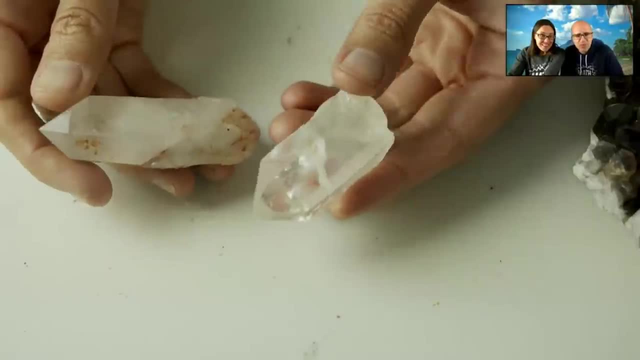 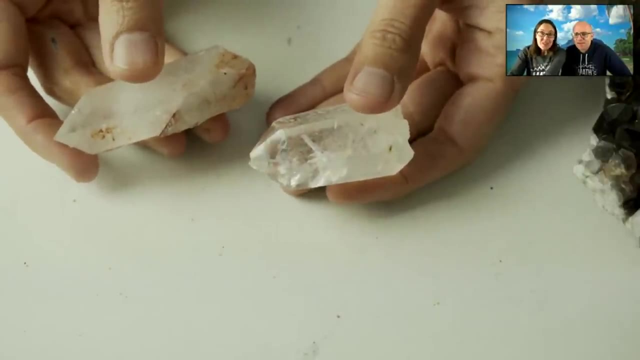 It looks like glass. It's so clear- almost No way, So that's naturally occurring. This is naturally occurring. This is natural quartz and it grew like this. Now, a crystal is something that has a regular repeating pattern And there's a really common crystal. 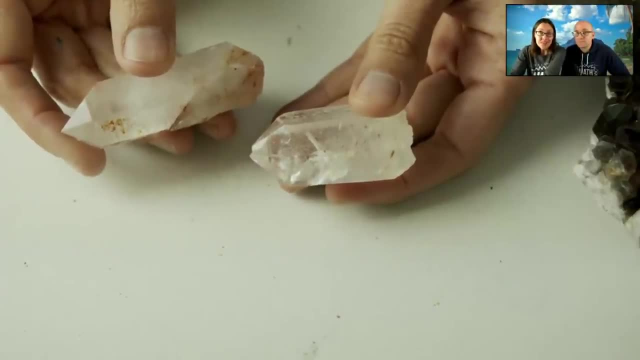 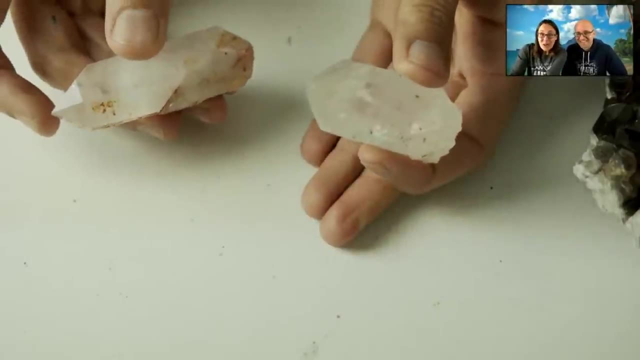 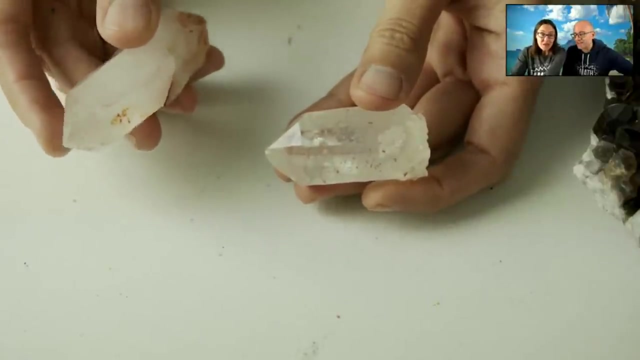 probably in your fridge right now it's called ice. oh, because when water in a freezer, for sure in your freezer, that's what i meant. because water, when it freezes, it likes to lock into a pattern, into a crystal pattern. and quartz, which is made out of silicon and oxygen, quartz does the same. 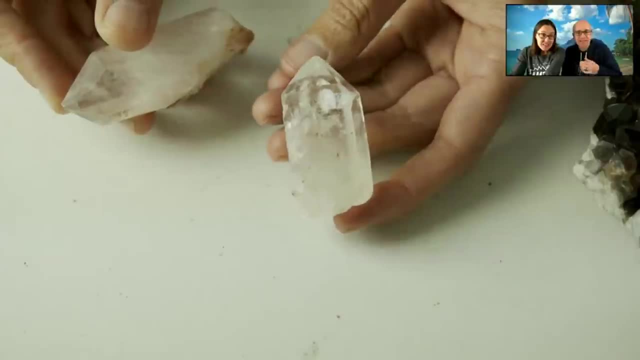 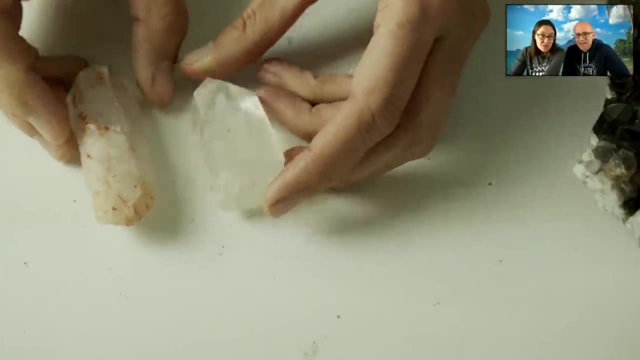 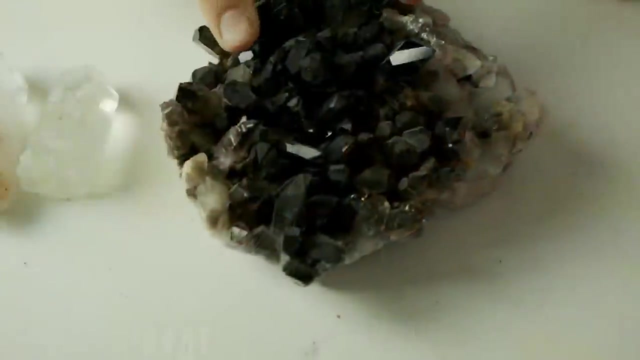 thing, so like in a cave, or how does that? or underground, underground, underground. so yeah, it forms underground as um. as igneous rocks are cooling down really slowly, you will get quartz forming. now this is quartz, but this is also quartz. this is smoky quartz, if you can zoom us out just a. 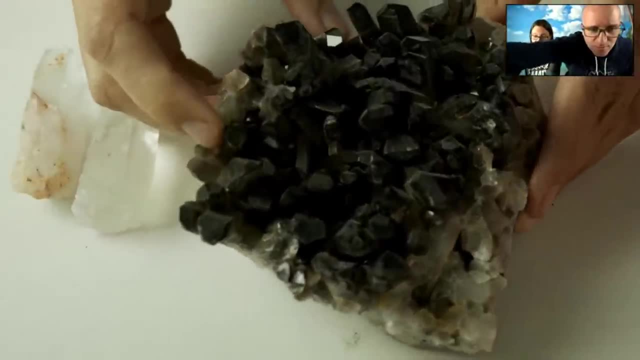 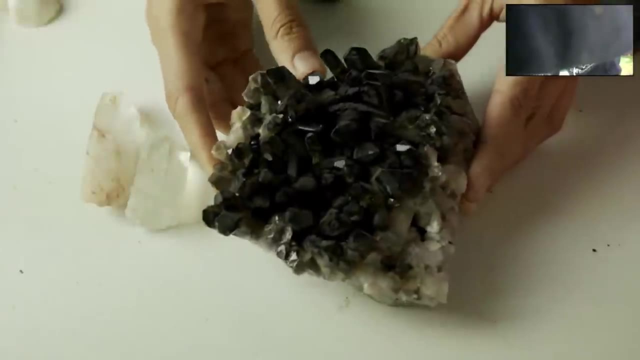 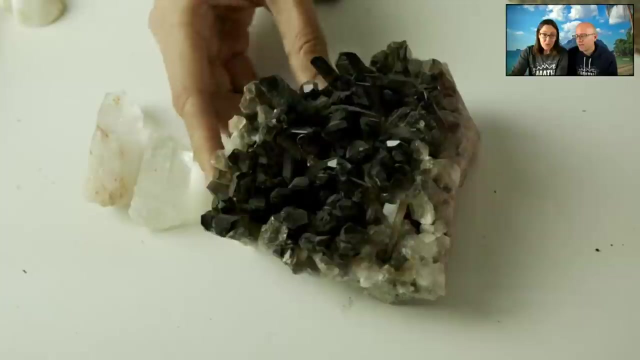 tiny bit math, dad, so they can see that just a little bit better. look how cool these crystals are. they're all growing up and again. this is naturally forming, but the color is completely different. so color of a rock turns out to not be the most useful thing in determining what a rock is. because this is quartz, this is. 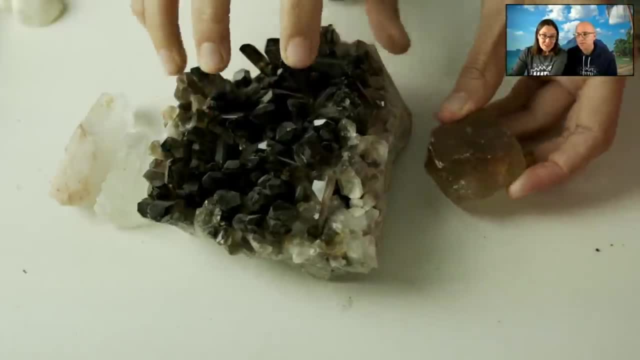 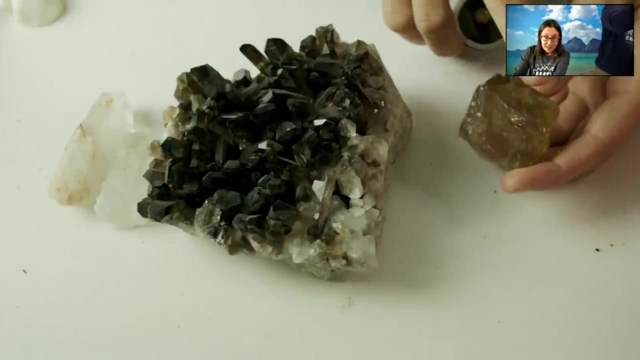 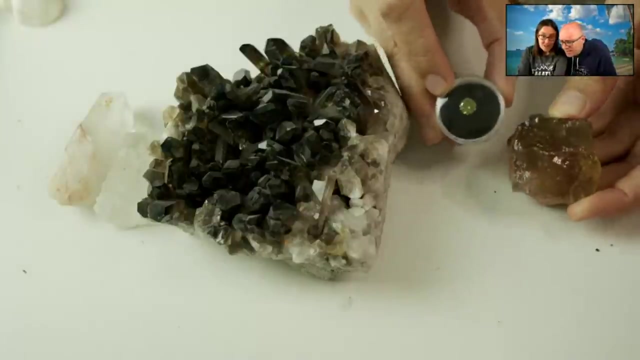 quartz, and this is quartz too. now it's a little hard to see with our light here, but this is actually yellow, and if this is polished and cut to be a gemstone, then it looks like this: this is citrine, raw citrine, and then polished and cut citrine. it is also quartz. it's a yellow. 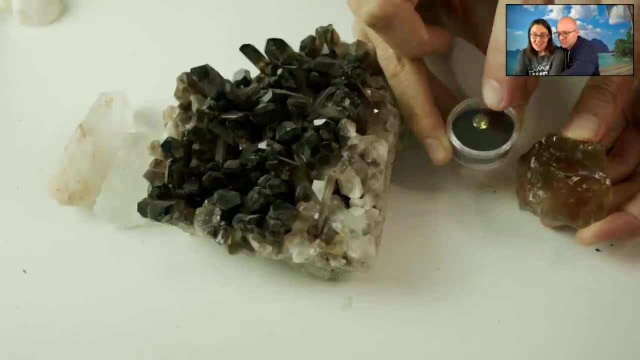 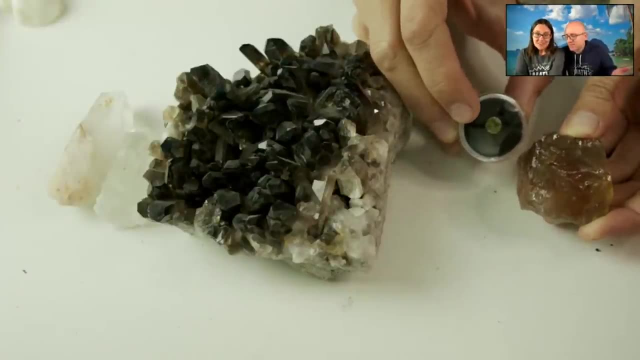 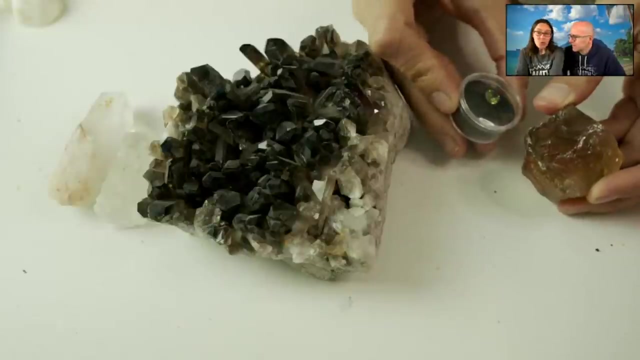 variety of quartz. no way, i mean. this one looks like a gemstone. it is in a ring. yes, yeah, those are all quartz. these are all quartz. that makes almost no sense. so what is causing the difference in the colors? tiny amounts of other elements or other atoms. so quartz is mostly made of silicon and oxygen, silicon oxide, but there are other. 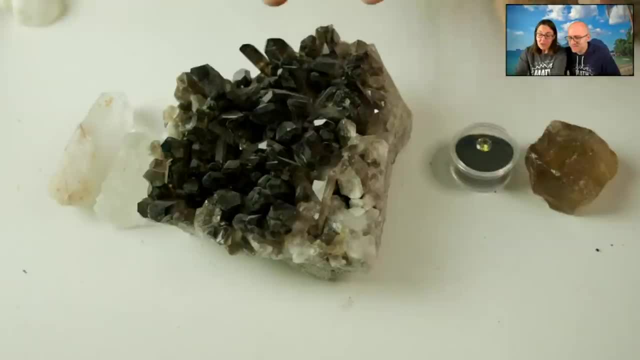 little elements that can get in there, and just a little bit of a certain element can cause a huge difference in color, and we see this especially with corundum. have you ever heard of corundum math, dad? i have? that's a pretty hard one, right, it is a pretty hard. it is a gemstone, a mineral. 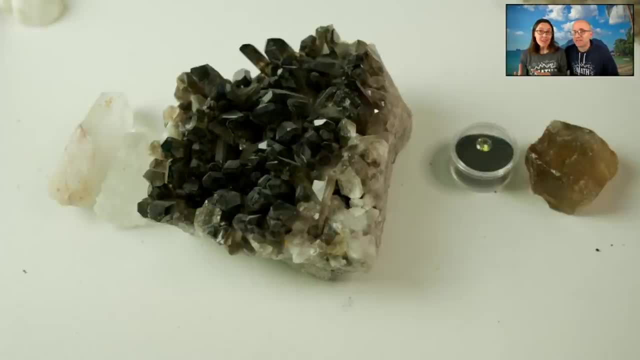 and depending on which variety you have, it will be different colors, and it could be. do you remember the two? it's ruby. it could be a ruby if it's red or sapphire, or a sapphire if it's blue. and then there are colors that are sort of in between that spectrum as well, but they're the same thing, they're. 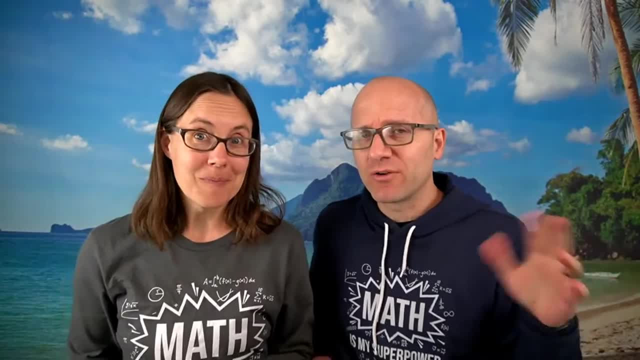 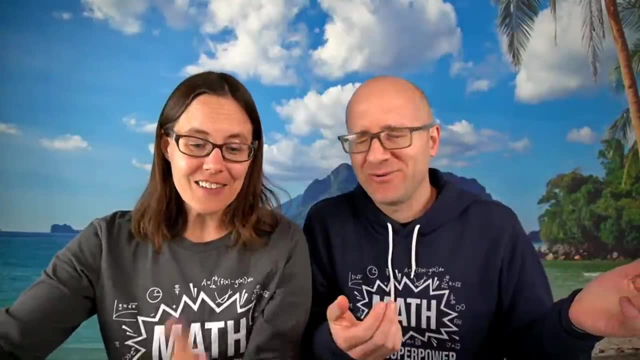 both corundum, so just other impurities or other elements are somehow in there and they're different, and that's where we get the difference in color. that is where we get the difference in color. let's talk just a little bit about gemstones, because when some people hear mineral they think 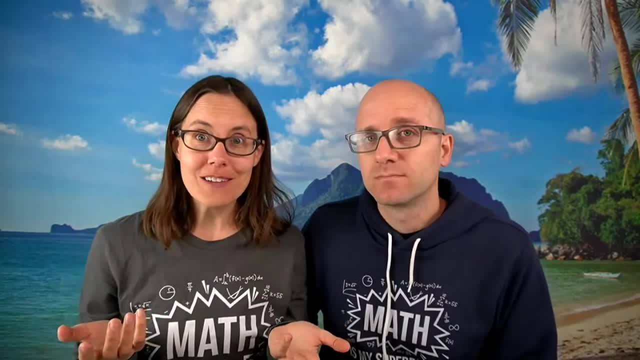 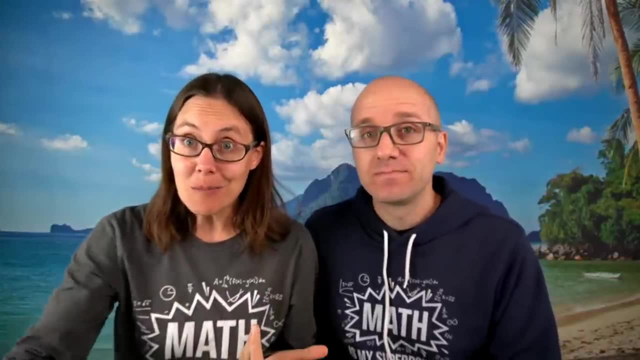 oh, like diamond and quartz. so we're just talking about things that we would put in in you know someone's crown, right, we're just talking about jewelry. well, no, we're not just talking about jewelry, but gemstones are a very valuable to us human beings because they are so hard and 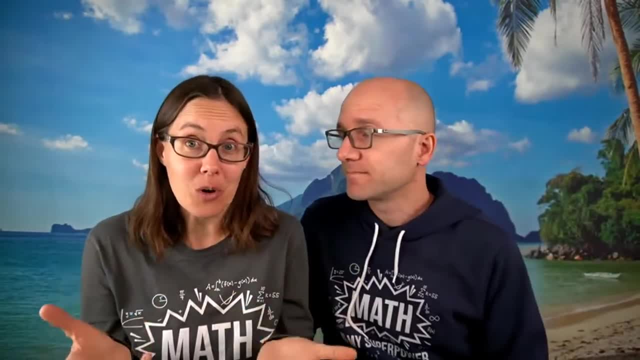 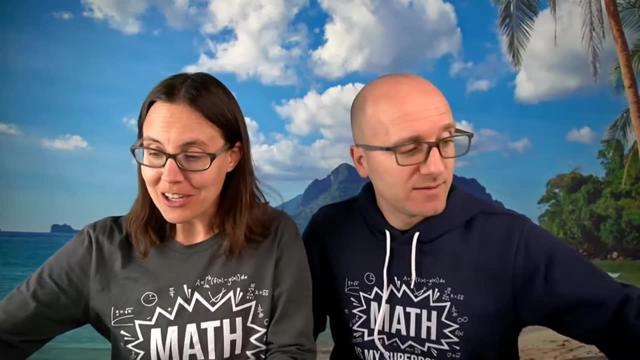 beautiful and you can cut them into these expensive and gorgeous pieces of jewelry. and there's a shapes, and so we like gemstones as as a species. but there are a lot of variety with our gemstones. let's take a look at some some cool examples. so this is not necessarily a gemstone, it's a rock. 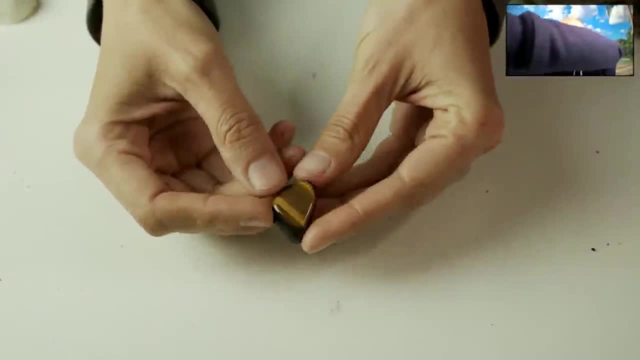 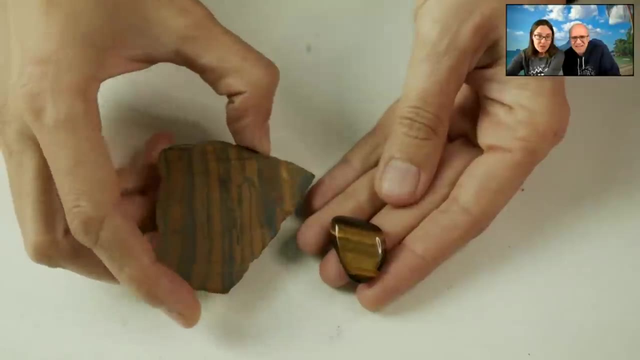 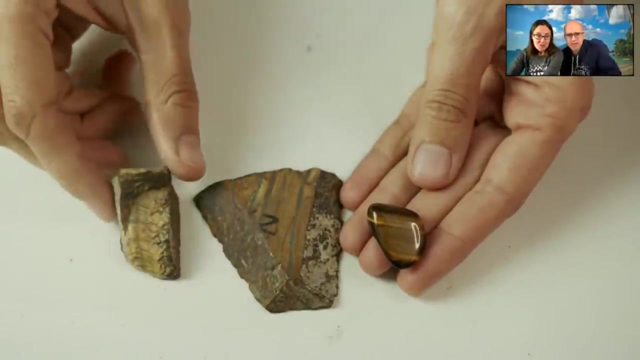 it's called tiger's eye and it's usually polished to look like this, and I brought this just as an example to see how different something can look when it's raw versus polished, because here is tiger's eye before being polished. okay, so what does one do to polish a rock? you've got to tumble. 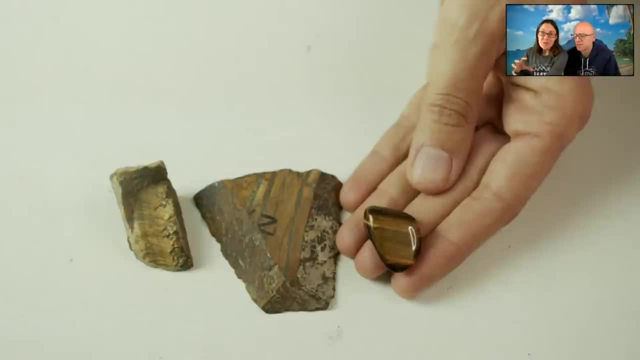 it. so people will have rock tumblers, which basically is just a big barrel with some rough stuff in it like sand, and you just tumble it around and around and around, kind of like what would happen naturally in a river. okay, so that kind of breaks off any corners and it smooths. 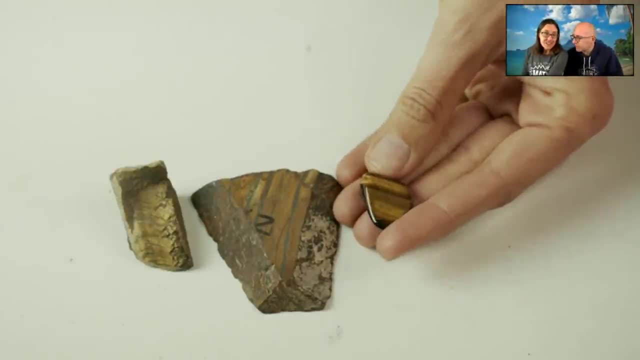 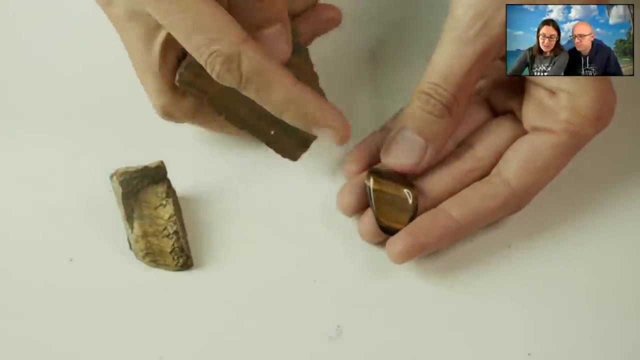 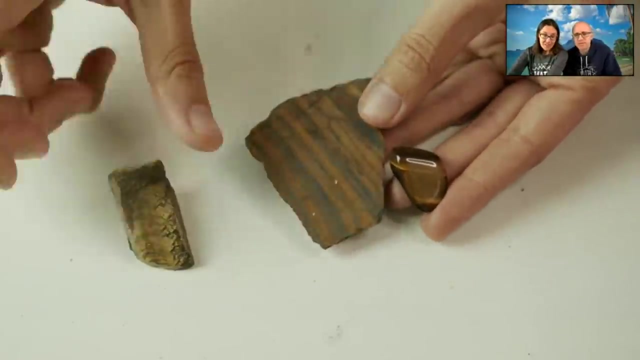 it out. but but how does it make it shiny? does the tumbler make it shiny? yeah, just getting it smooth. so this this surface here. if we polish it and get it really smooth, it would also look similar. but this has been cut but not polished as smooth as this one has. so these are all tiger's eye. this is raw tiger's eye. that hasn't. 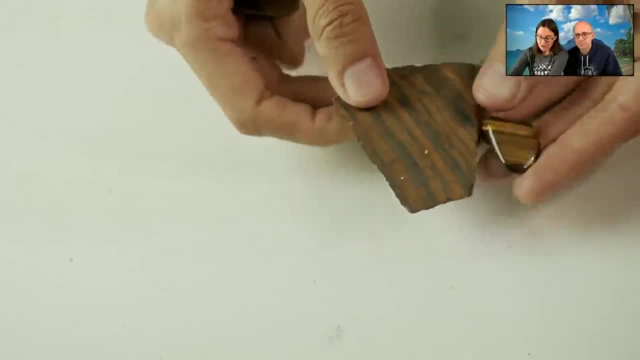 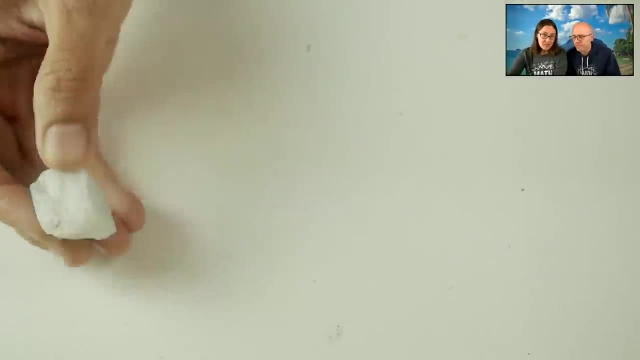 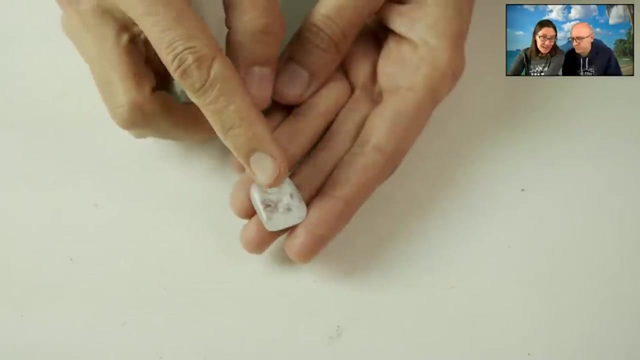 been tumbled or polished. yet this one has been cut but not polished. and then here is one more example. this is aquamarine, another gemstone. this is raw, so it's slightly bluish cast to it. is that where the name aquamarine? yep, and this one is polished. and if it was cut and polished? 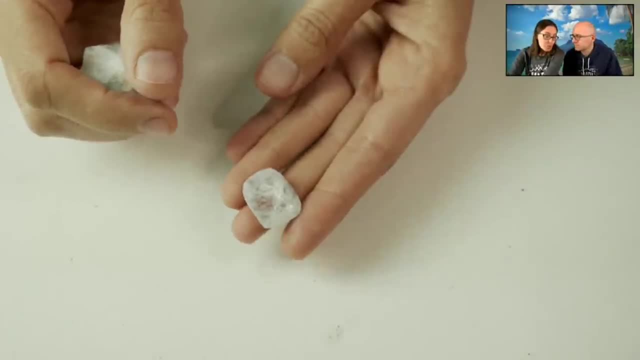 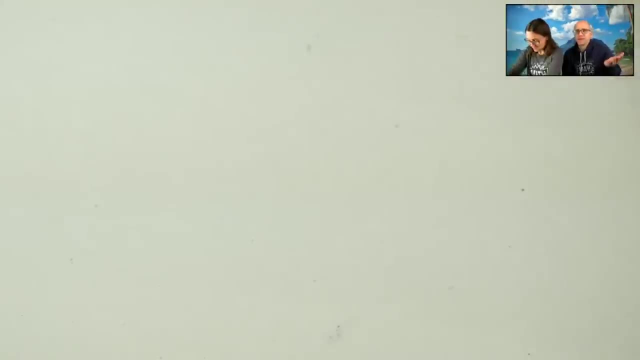 to look like a gemstone, then it would look sort of like a bluish diamond. only this is not as hard as a diamond. well, that's way cool. i mean, i, i couldn't recognize a diamond. i, even if i had a magnifying glass, i wouldn't know what to look for, although professionals do know what professionals 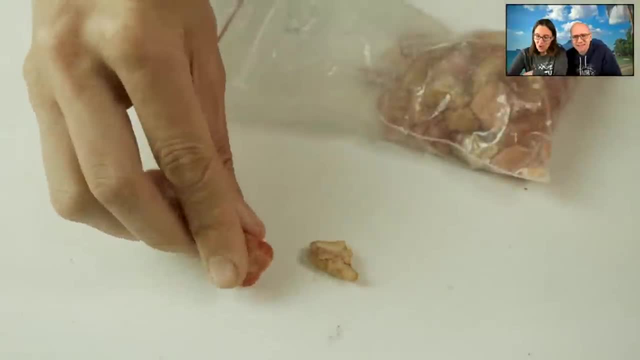 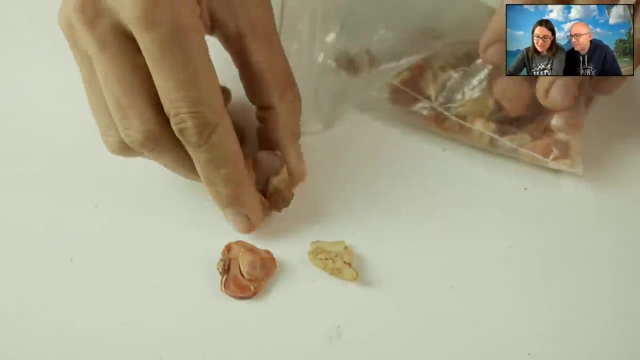 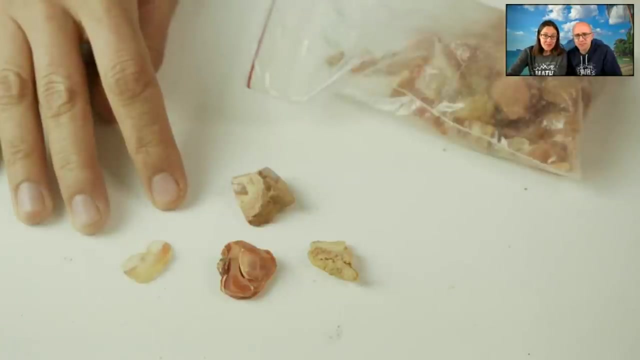 do. and then this right here: this is opal, common opal, you can see. it has a beautiful color, and if we were to polish it and cut it a little bit more nicely, this could be. this is used as a gemstone as well, but this is not a mineral. wait, what's a mineral then? because, remember, a mineral is. 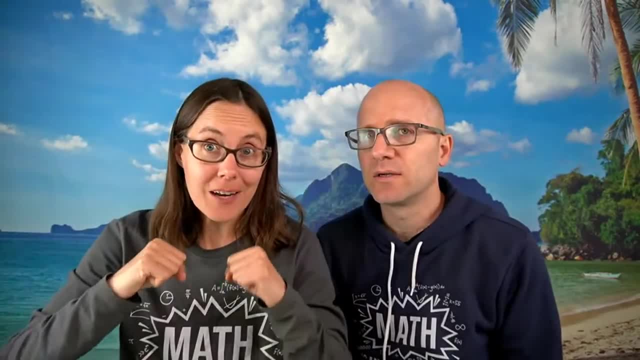 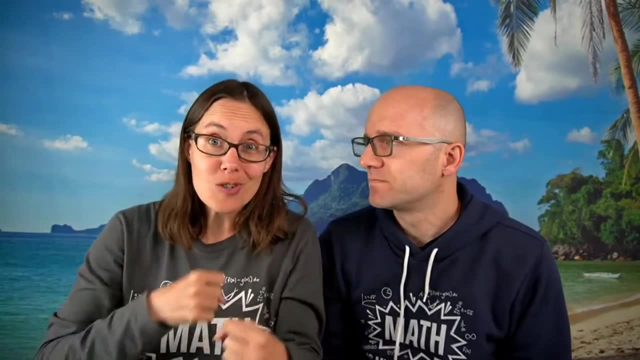 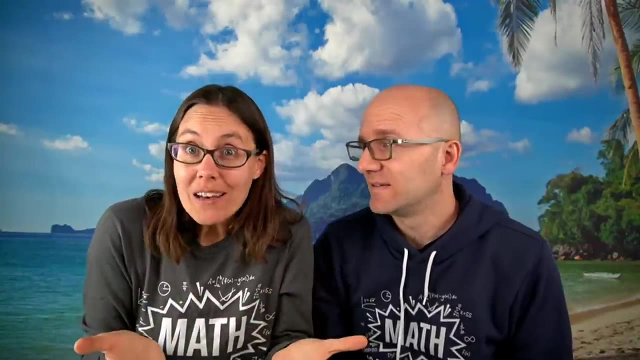 something that has a regular crystal structure where the atoms are stacked and arranged in a really organized way. and if the atoms are not arranged in an organized way, if they're just kind of, you know, all over the place, then it is not a mineral and we can call it a mineraloid, like it's. 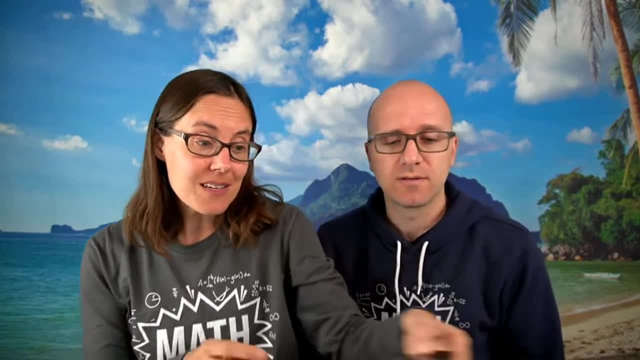 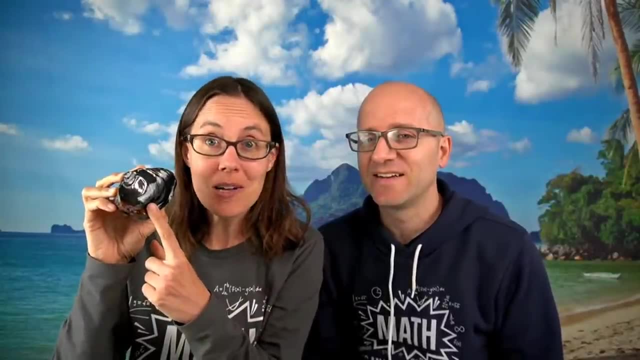 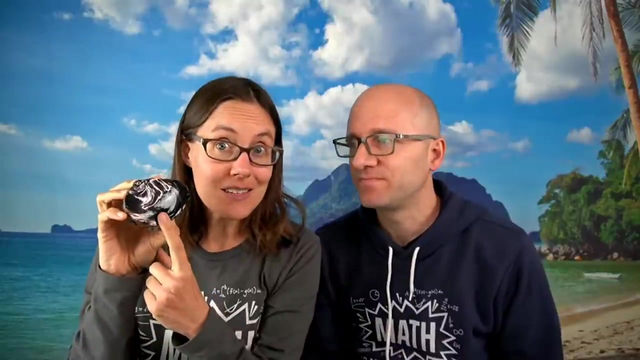 similar to a mineral, and obsidian is a great example. obsidian is volcanic glass. it's an igneous rock that cooled down really quickly the atoms here. because it cooled down so quickly they did not have time to organize themselves and get all into a crystal structure, and so this is what we call amorphous. that means the atoms are not. 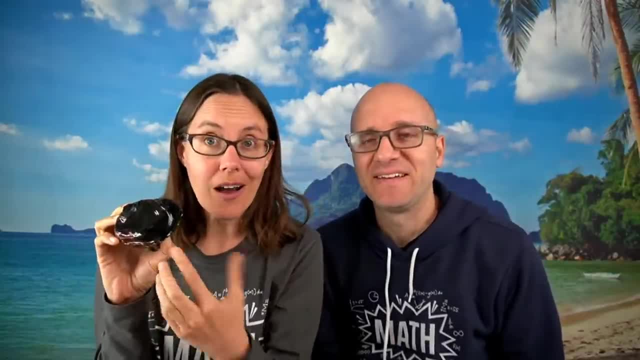 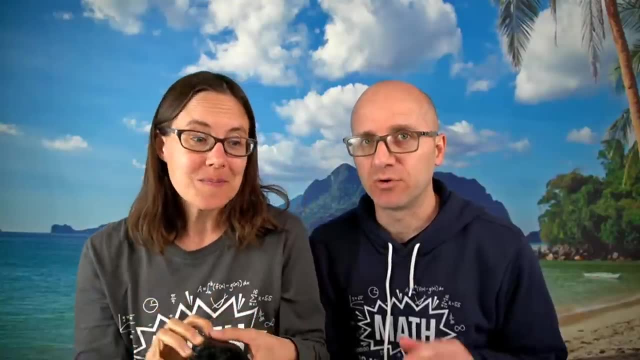 lined up, so this is obsidian. if we were to cut it and maybe make it look like some sort of a black gemstone, it would not be a mineral. it's a big mineraloid, mineraloid, mineraloid. and there are several things that are not minerals, that we call precious gems. let's take 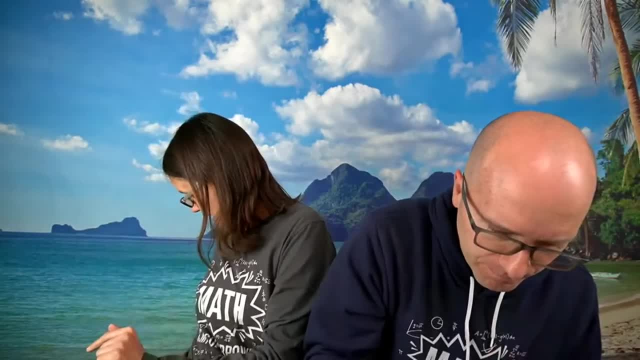 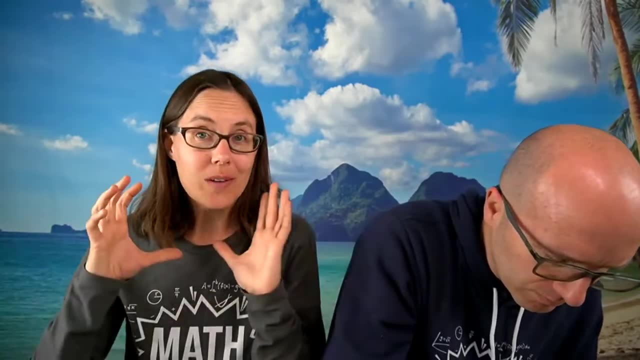 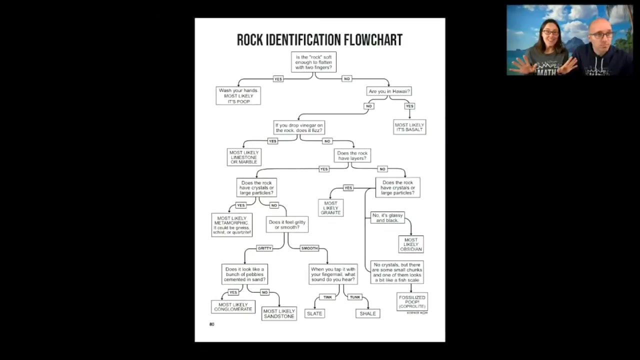 a look at our notes real quick. we're going to be on page 81 and i have a little venn diagram to help kind of separate it out: what's a mineral, what's a mineraloid and what is a precious gem or a gemstone, because they're not all the same thing. so we'll come to back to this one in just a minute. 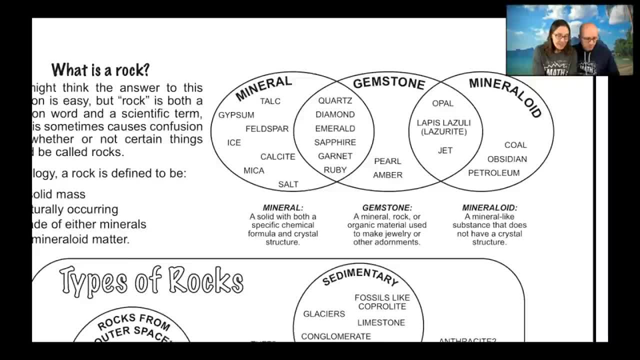 here we are, on page 81, all right now, an opal, the stems, the stones that we were just looking at. these are gemstones. they're often used in jewelry, but they are not minerals. they don't have a crystal structure. pearls come from oysters. they're actually made by a living thing and they are beautiful, but they're not a rock. 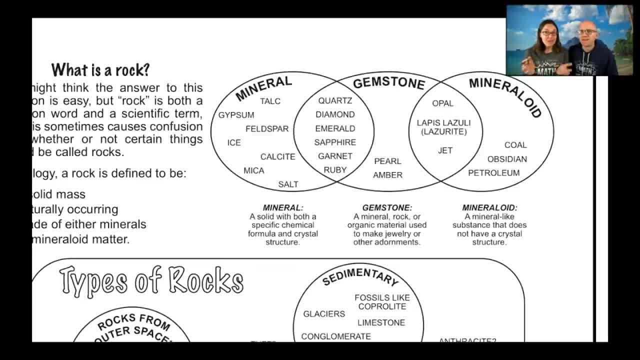 they're not even a mineral, because they are made by a living organism. oh, and that's part of that definition. yes, same thing with amber. so amber is fossilized tree sap and it's made from a living animal, not of any kind. so if it's a living having a real life, it looks really beautiful and sometimes 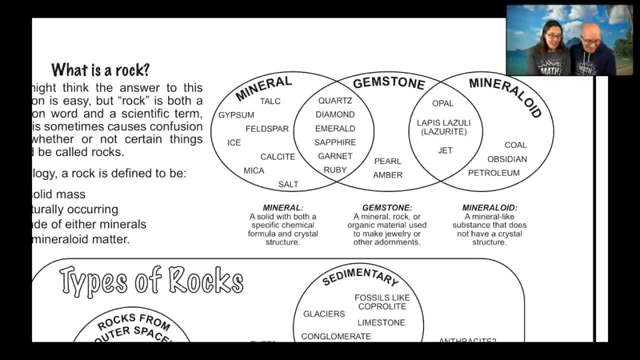 can be used as a gemstone, but it is not a mineral and not a mineraloid either. it's kind of a separate thing interesting. and then coal can actually be cut and into a gemstone if it's hard enough, and that's called jet. so here is a piece of coal. this is actually a hard enough piece of coal if we 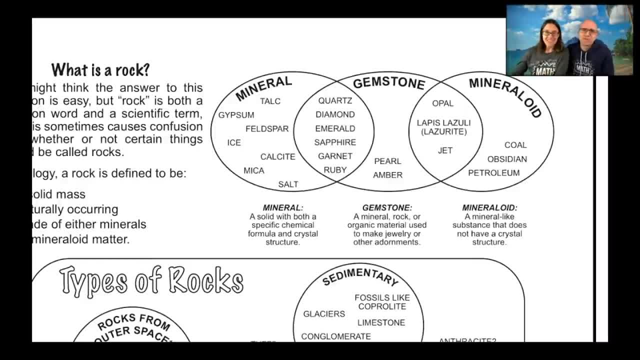 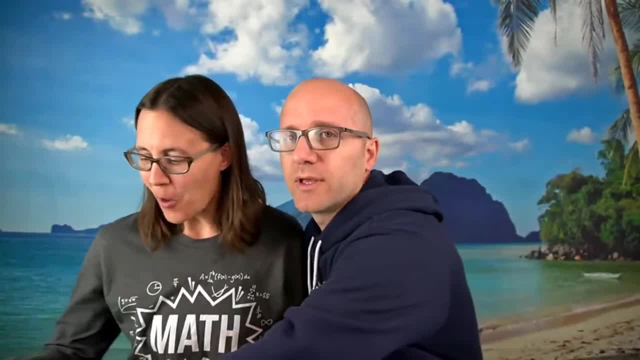 wanted to polish this, we could, and it would be a gemstone called JET Jet. okay, that's a cool name for a gemstone. it is a cool name for a gemstone, agree on that. oh no, i'm sorry, we hold up the coal. we were in the small picture mode. there we go that. 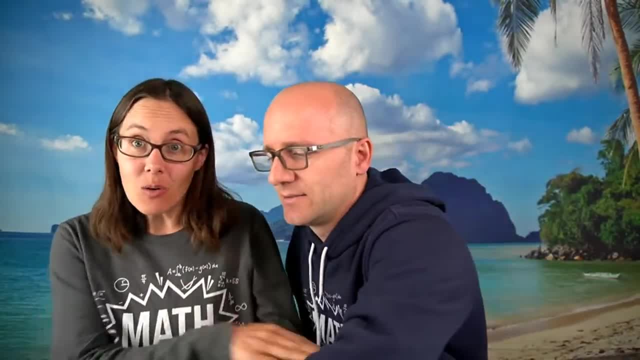 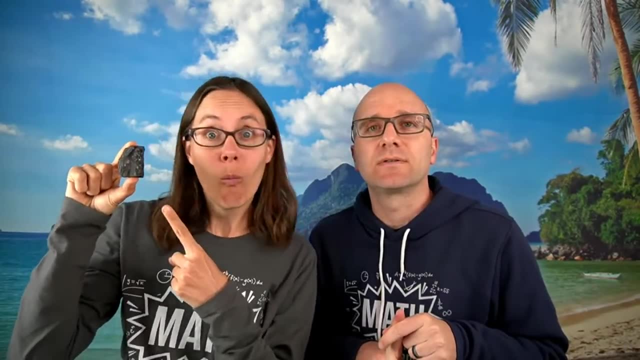 is a piece of coal, crazy. so is coal a mineral? math, dad, don't look at the flow chart. oh man, no hints from the chat. so it's yeah. is it a mineral? does it have a crystalline structure? so, yes, it's a mineral. it is not a mineral. it does not have a crystal structure. oh, it doesn't. have the crystal. it doesn't have a crystal structure. are you going to find coal with little crystals of coal growing out? no, because it is not a mineral. all of the atoms are kind of smushed in and they are not organized. but there are lots of different types of minerals and one 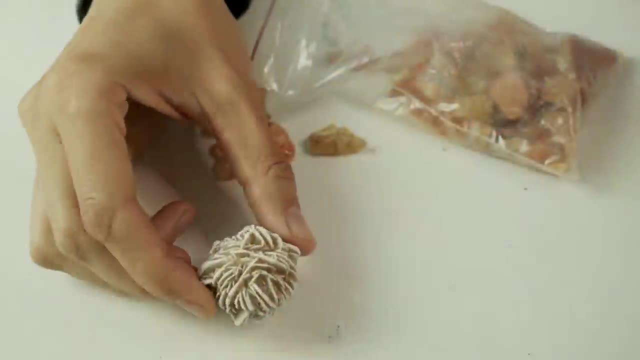 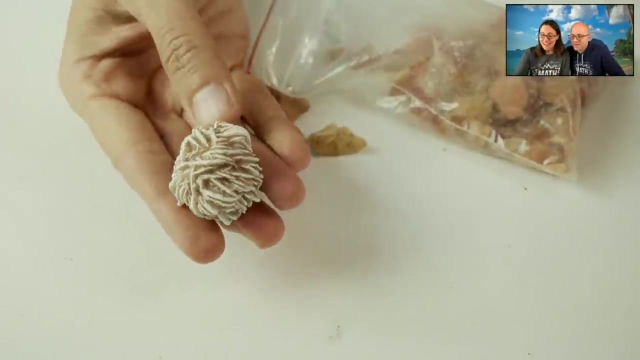 of my favorites is called selenite. take a look at this. this is sometimes called desert rose. shout out to ibrahim from canada, who identified that correctly from the thumbnail- and it is naturally forming. it forms like this all on its own, and these little ribs that come out that are 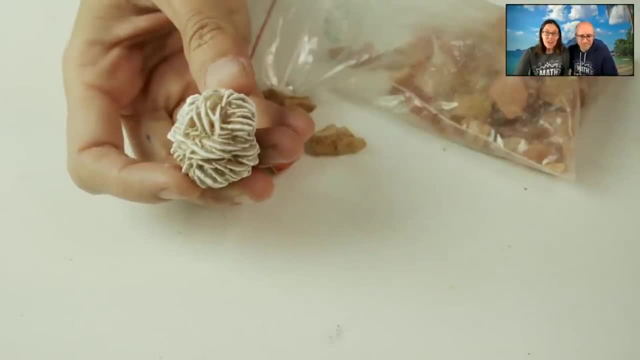 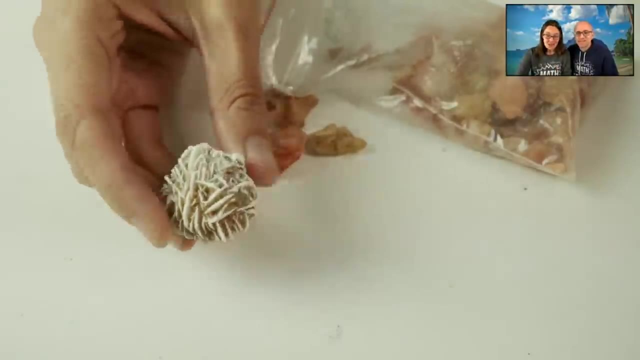 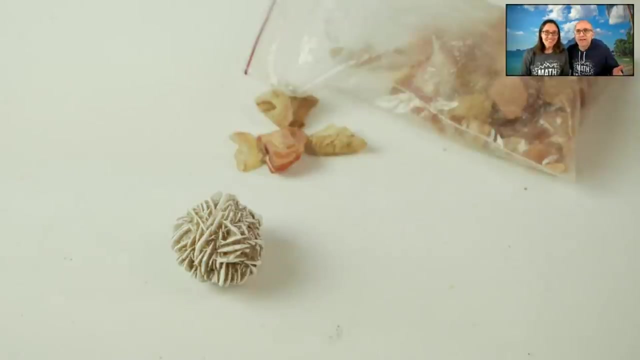 dusted white. that happens because it is a mineral and those atoms want to line up in an organized way. they want to be all lined up and this forms naturally, just like those quartz crystals did. that's, that's neat. i saw that the chat. everybody was getting the question right that i got wrong. so coal is. 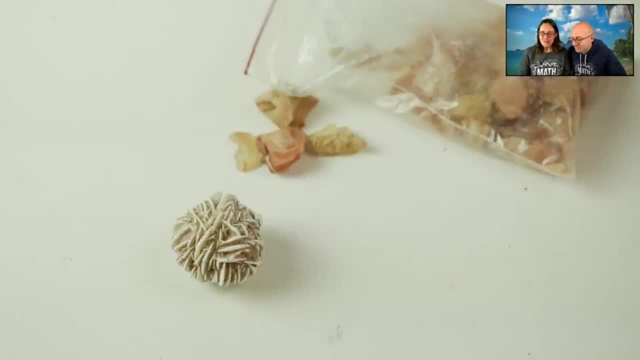 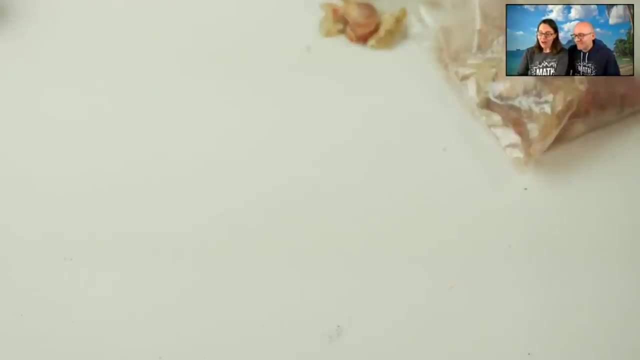 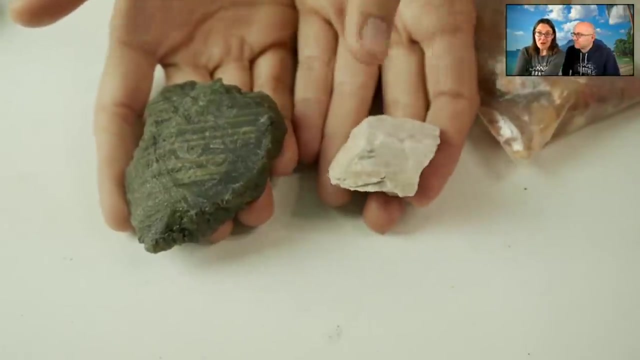 not a mineral. i'm gonna remember that one from now on. good job, unbeatable science kids. i want to show another example. that color is not a very good thing to use when you're identifying rocks. that's because this and this are both feldspar. what feldspar is one of the most common minerals on our 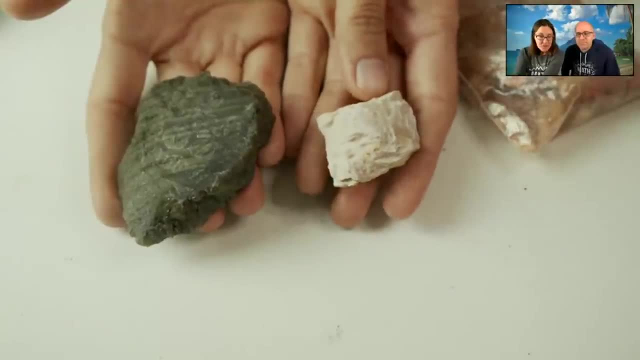 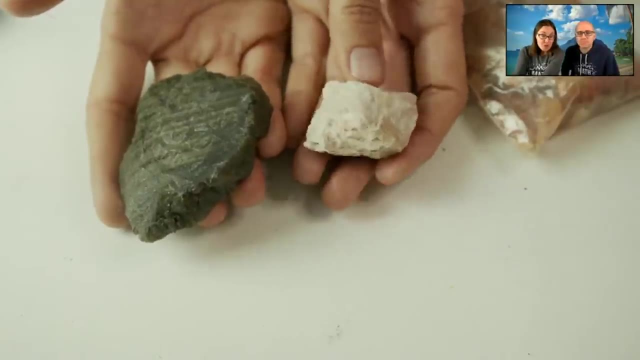 planet. a lot of rocks have feldspar in them and it's it's not a mineral that you're going to see growing into crystals, um, like you do, quartz, where they're a really pretty glassy structure, but if you look under a microscope and you look at the structure, there is organized, an organized lattice. 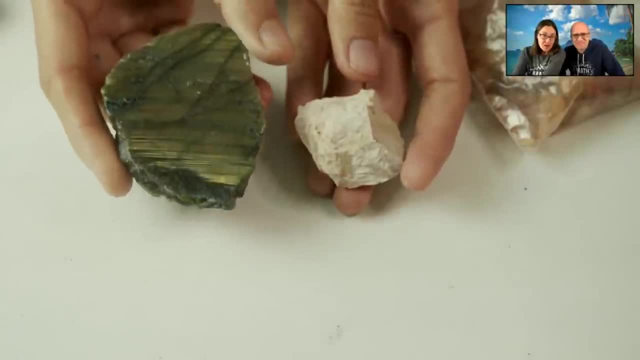 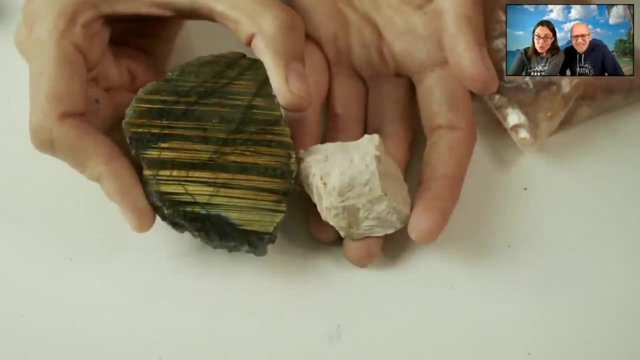 to this, to this mineral and certain types of feldspar, will actually form layers. this is labradite feldspar. isn't that beautiful? yeah it is, but you don't see it unless you polish it. without being polished, it looks like. it looks like this. you can kind of see that there's some 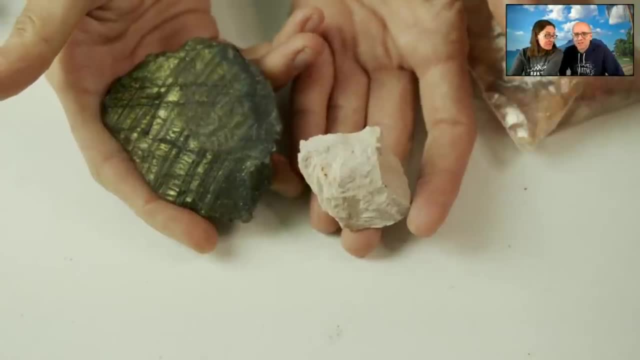 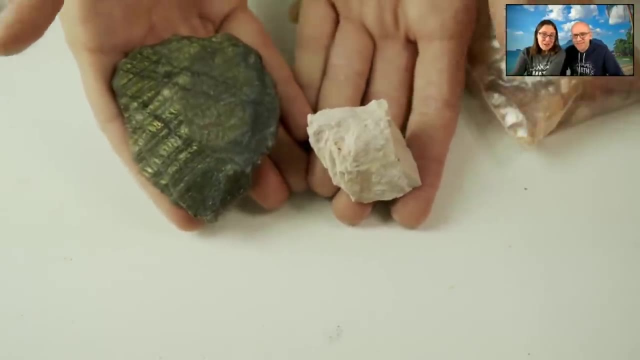 striping there, but it's not nearly as obvious, and this makes me want to polish some rocks. yep, gotta get a rock tumbler. but both of these are feldspar. do they look the same? not at all. i would never guess that those were the same mineral. very, very different appearances. 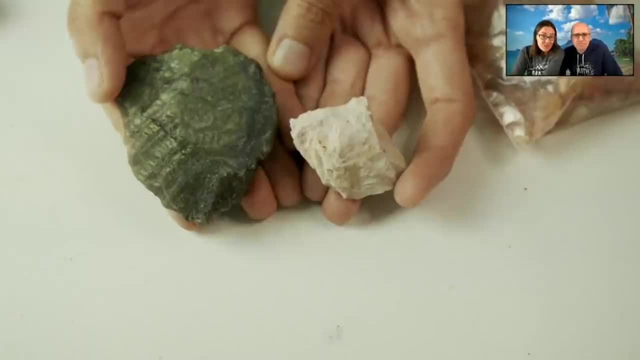 and they're different, a lot of different varieties of feldspar. but if you look at what the atoms are and what they're made of and how it's formed, they're not the same minerals, they're not the the crystal forms. they're pretty similar even though they have totally different colors. 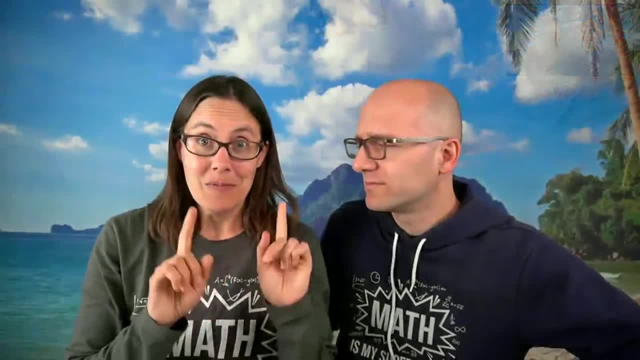 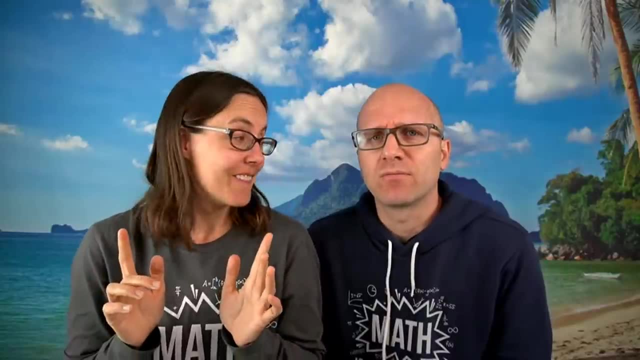 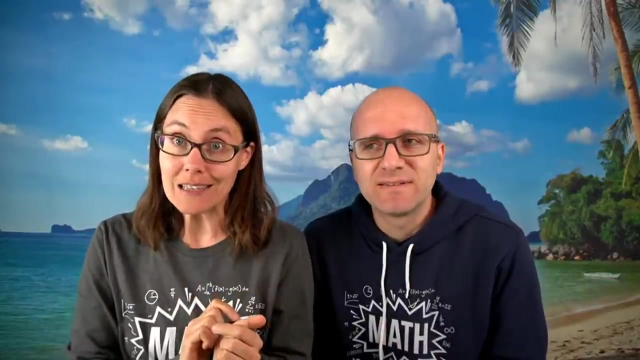 okay, next way cool. there's one more mineral i want to talk about that you actually have in your kitchen right now. you're talking about our granite countertop. nope, nope, not the granite countertop- although the granite countertop might have some quartz crystals in it- but granite itself. 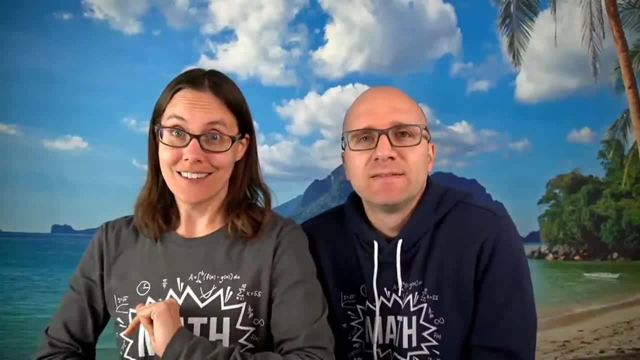 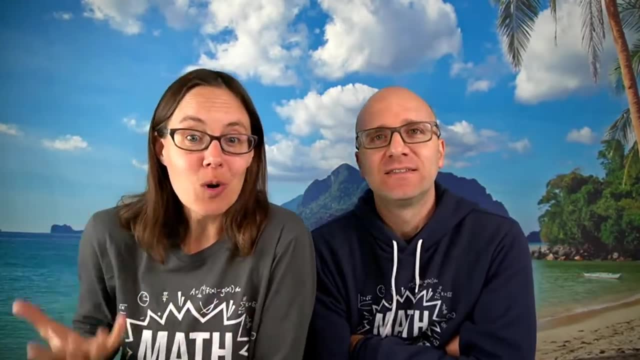 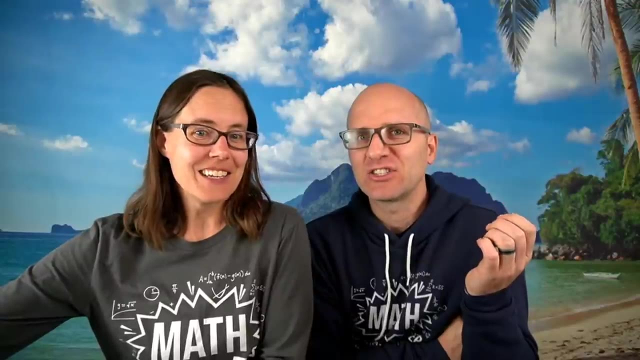 isn't a mineral. i'm talking about a mineral that you eat- and if you're watching the replay, see if you can guess the answer before math dad- a mineral that you eat, that is in your kitchen, that can form a rock. okay, i've got, i've got a theory. it's got to be the milk, like the calcium, the calcite. 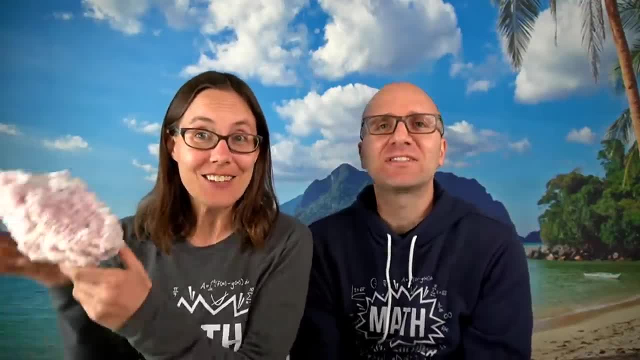 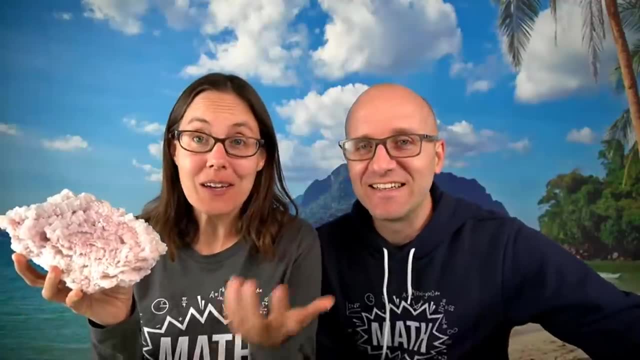 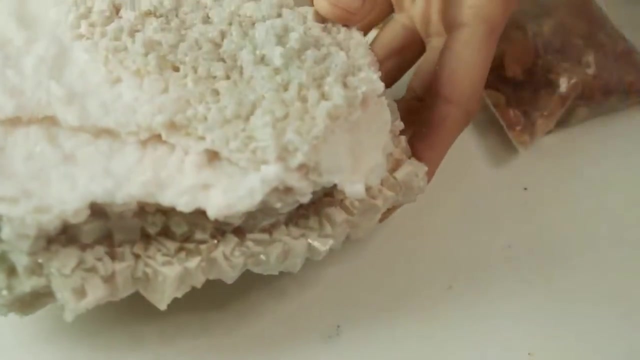 amy's got it, dexter's got it, rachel's got it. i love what it is salt. this is halite, or rock salt, and we call it rock salt because it literally does form rocks. so this forms on the top of a lake bed and when they went and harvested it it looks like this and you would reach underneath and then break. 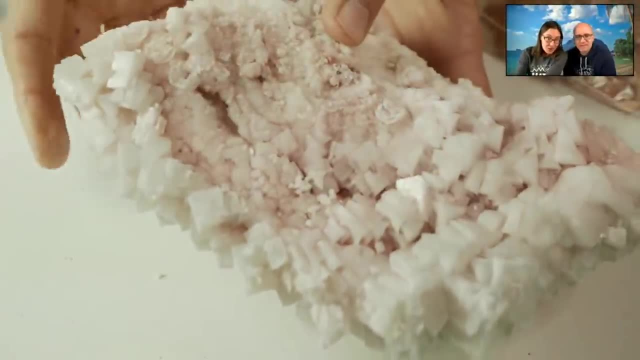 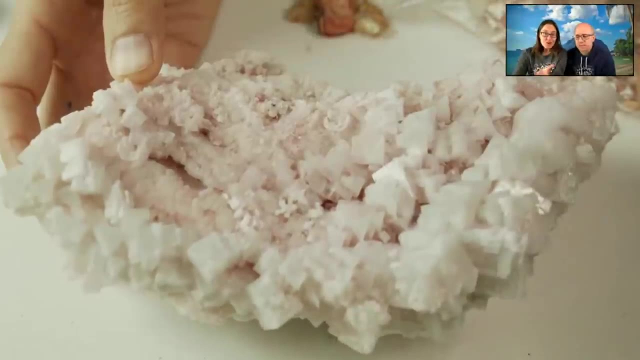 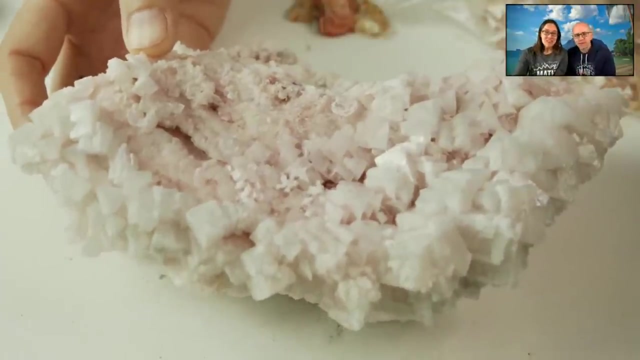 it up and when you turn it over, you see these incredible crystals. those are huge. they are huge and they have a square shape because salt forms a cubic crystal. they meet at right angles. yeah, it really is. isn't like a pointy diamond? no, so math dad, is this a rock? well, it's a. 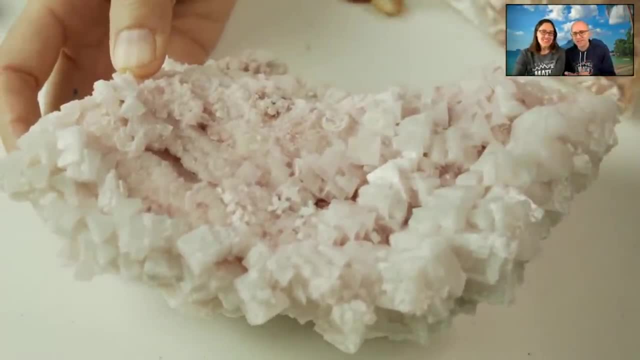 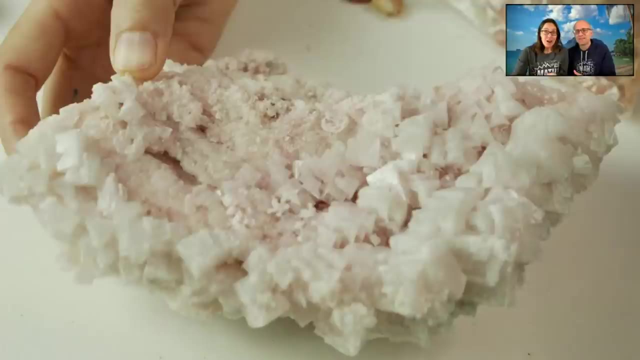 mineral rocks, because i i yes, it's got to be a rock, it's natural. it's got a crystal it formation and, yeah, it's a rock. yes, it all depends on how you define rock and sometimes people will get in arguments. even fellow geologists can get in big arguments about whether or not something is a rock. 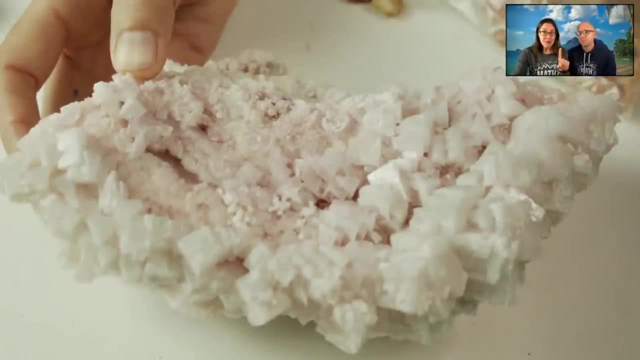 but if we define a rock as being naturally occurring- that means it's not man-made or animal-made and that it is made of minerals or mineraloid matter and that it is solid- then this is a rock and it's made of salt. but this rock here, if you dropped it in a bunch of water, it would. 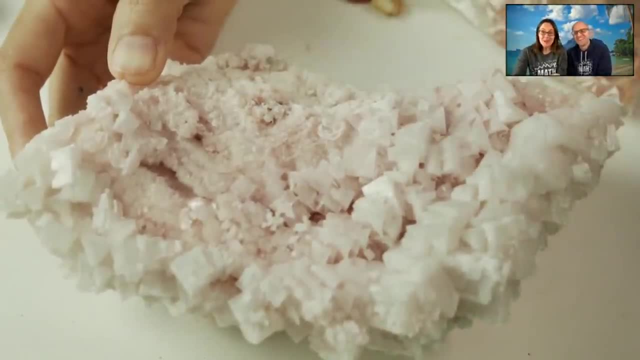 eventually dissolve because it's it's made of of salt, it is rock salt. it's kind of weird to think of a rock dissolving, and if this rock is put under a lot of pressure, there are certain rock salt deposits that would not dissolve very easily because they are so compacted, but this one was 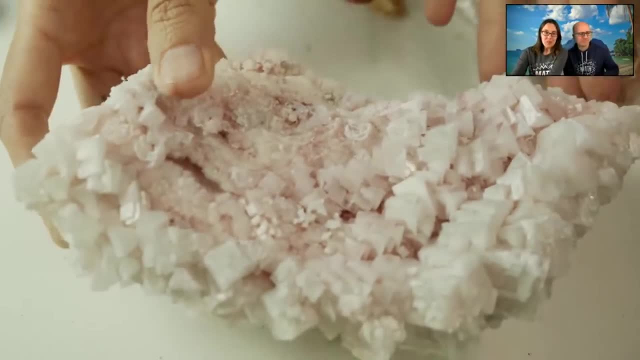 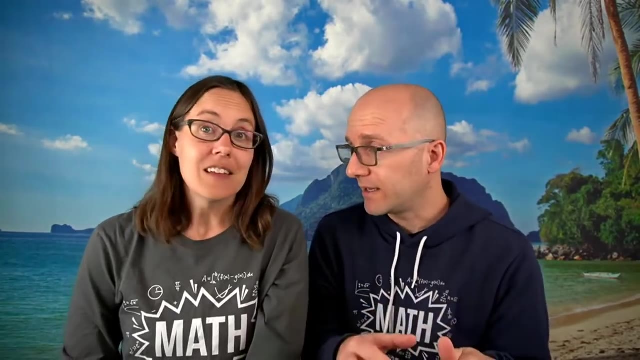 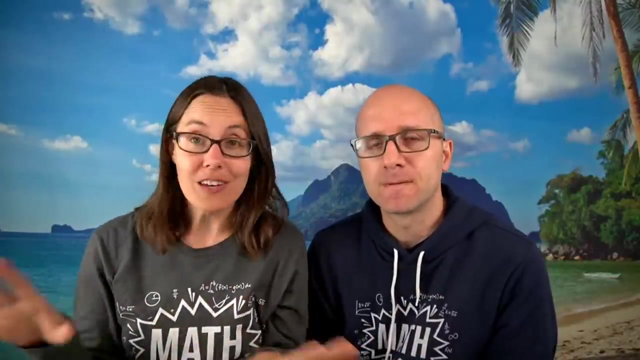 formed on the top of a lake and it would dissolve. so that's why we're not getting it wet. so something is not a rock because it was man-made, that's right. if an animal helped to create it, then we don't call it a rock, because rocks are naturally occurring out in the natural world without 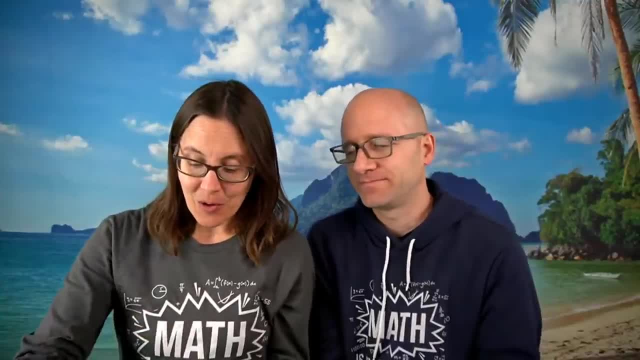 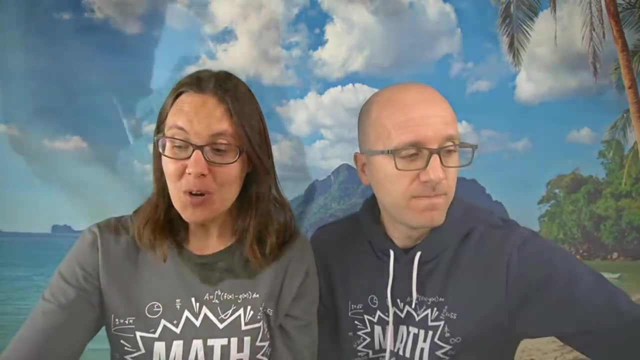 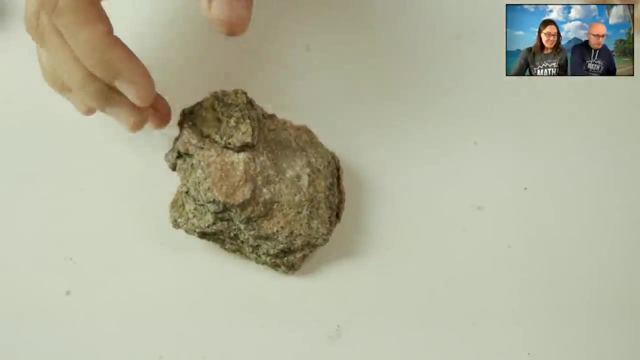 some animal, making them we cool. now we are ready, i think, math dad, to try identifying a rock. okay, i have a rock right here and we are going to go through our little flow chart and see if we can figure out what this rock is. oh so, this is the flow chart in the notes on page 80. 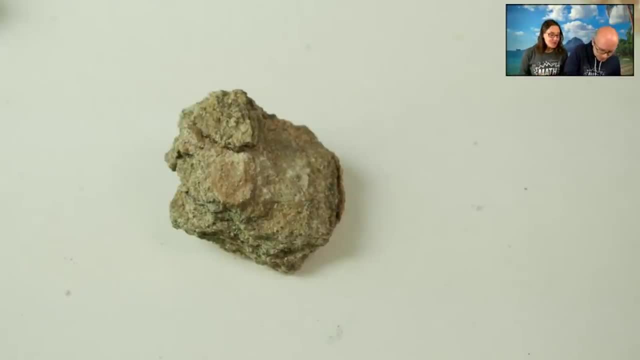 which you refer. that is right, and this first question on our flow chart has to do with where you are and when you're identifying rocks and trying to figure out what a rock is. the best question to ask first is: where did the rock come from? because there are geographic, not 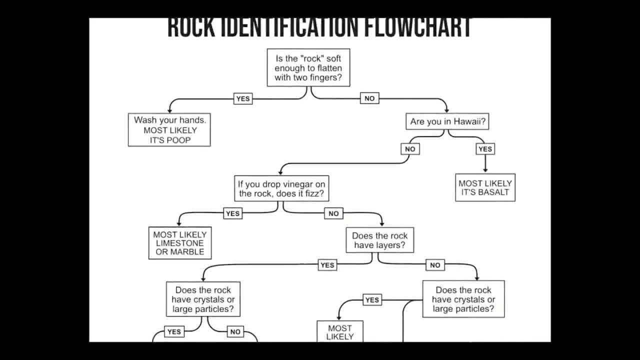 geographic, geologic maps that will show you what type of rocks occur where, and that can be really helpful as you try and figure it out. so first question: is the rock soft enough to flatten with two fingers? this is a fairly important one, because sometimes you'll pick up what you think looks like a cool 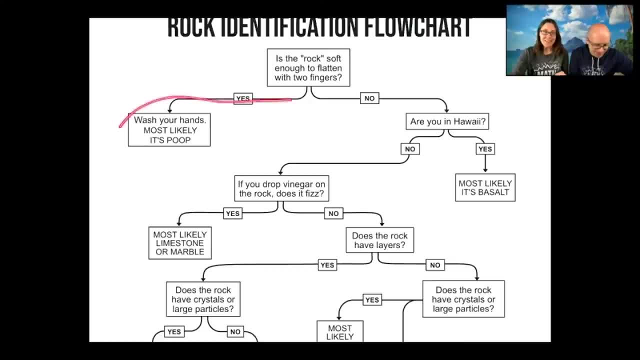 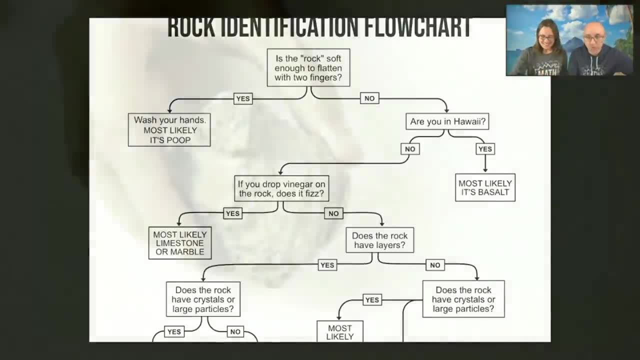 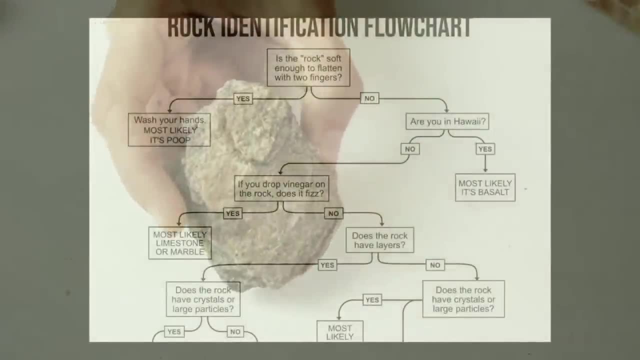 rock, but it actually might be something like deer poop, and if it's squishy, then go wash your hands because that was not a rock, all right. so the answer is no in this case. so looking at this particular rock, all right. so look at that, two for one. are we in hawaii? did this rock come from hawaii? 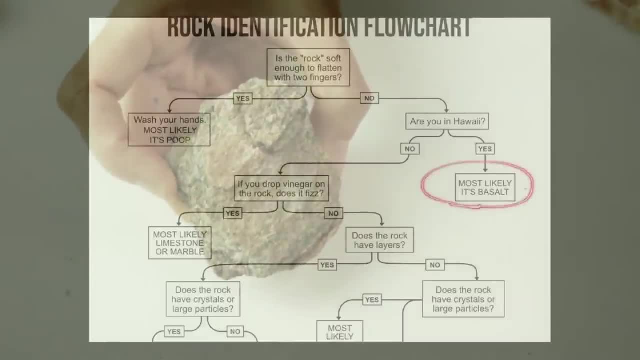 no, if it did come from hawaii, then most likely it was basalt. yeah, okay, so no, we were looking at this about 15 minutes ago to make sure we clear up. let's go, we back up to our main view. yeah, so the method i use here is to balance the Tennessean. 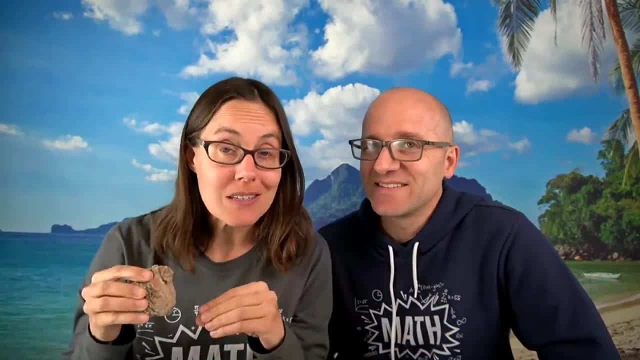 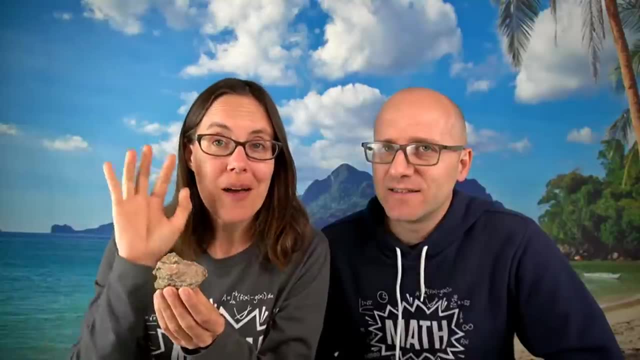 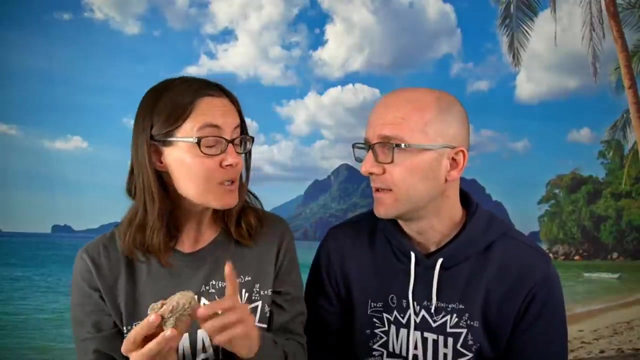 the brown disease is just getting the bran and fat, all right. so that means that you can have five years break and you create the rock that you're saying. it's in that monbinary rock stage, uh, as in the sickle. we found that already in the power stage, especially if you hit the rock and it either 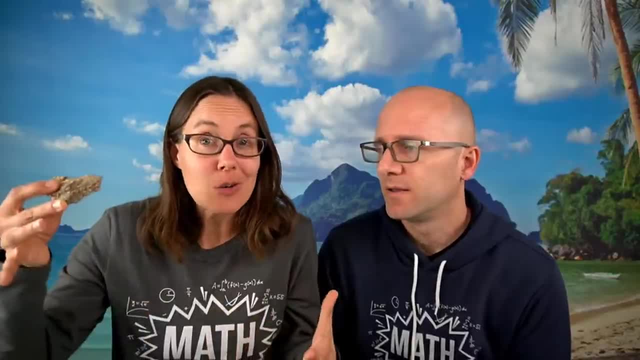 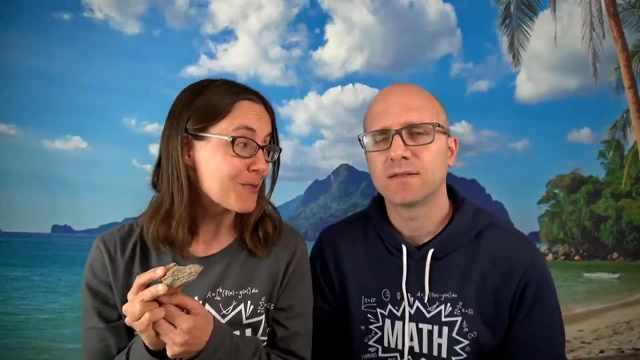 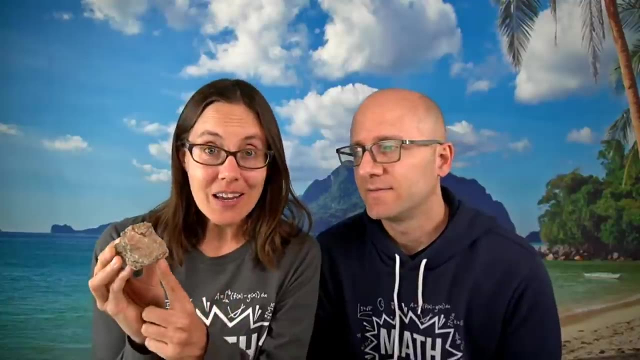 or marble, but sometimes you have sedimentary rocks that are cemented together with calcium carbonate. so rock identification can be a mystery. it can be a puzzle. is calcium carbonate like baking soda? it's. it's very similar to baking soda. yes, now this rock here. it does not fizz. 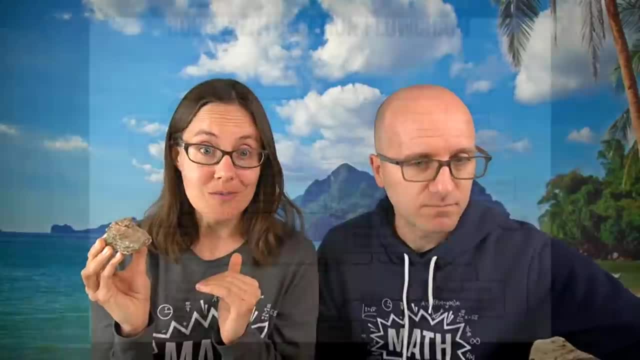 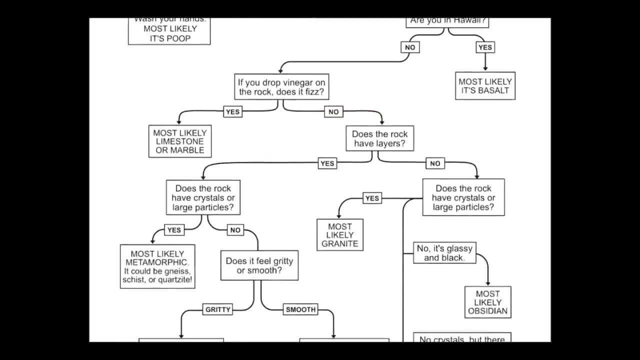 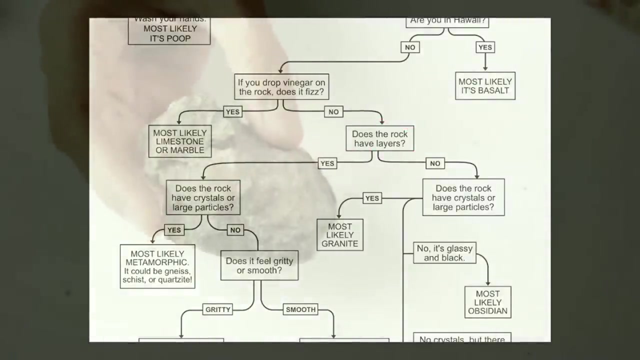 so we're going to go to our next branch in our little trail. all right, so you said the answer was no, so we're following it along this way. does the rock have layers? does the rock have layers? and this one can be a little bit tricky to answer. when i look at this rock, i do not see layers. so 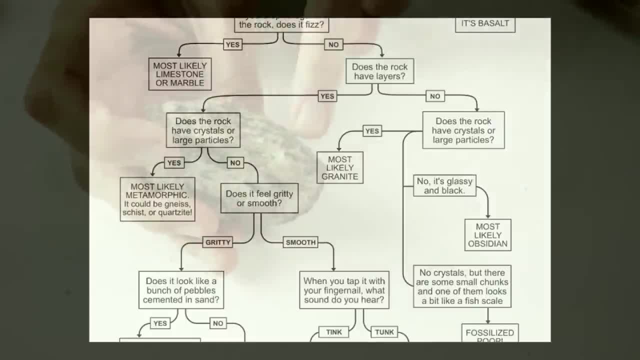 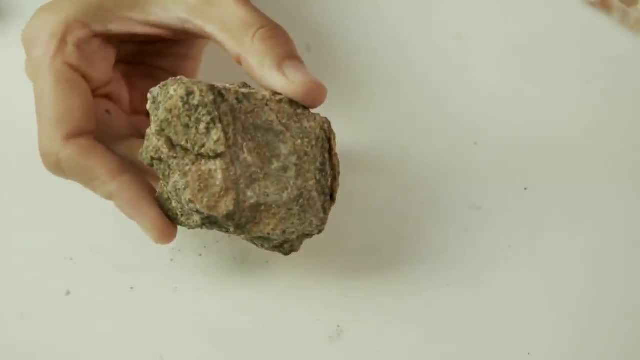 but you know what, if i look at it sideways, i do see some layers. do you see that stripe of black? and then there's a stripe of ground. so at first, if i look at the top, i'm going to say no layers. but then if i look sideways, say wait a second. 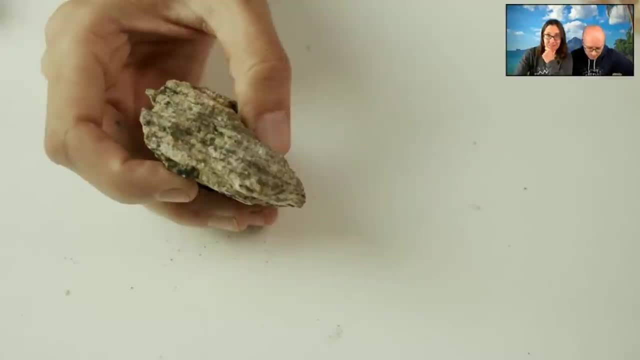 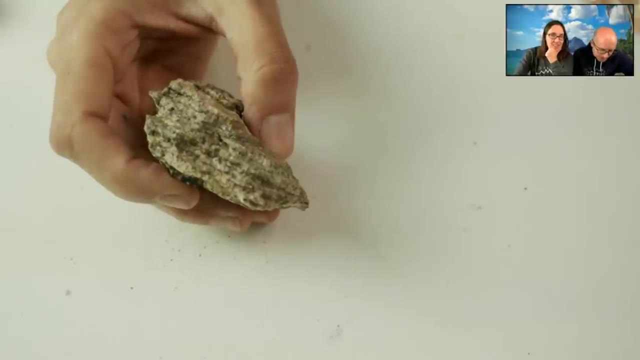 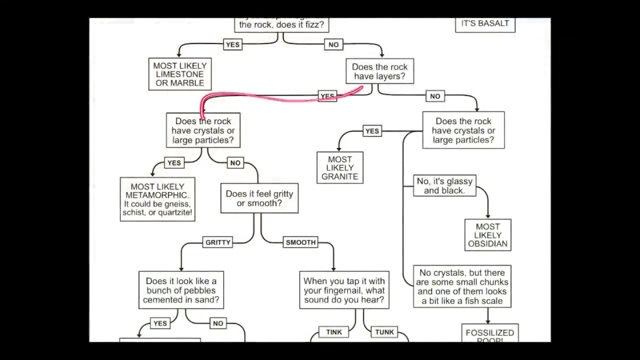 there are some layers. so let's say, yes, all right, it does have layers. all right, we are right here. oh, does there? oh, i'm sorry, did i jump down too far? all right? so, yes, all right, we're headed over to here. does the rock have crystals, i'm sorry? or large particles? so are there crystals on that rock? 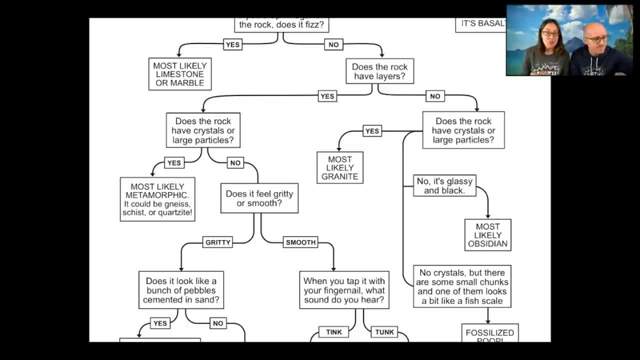 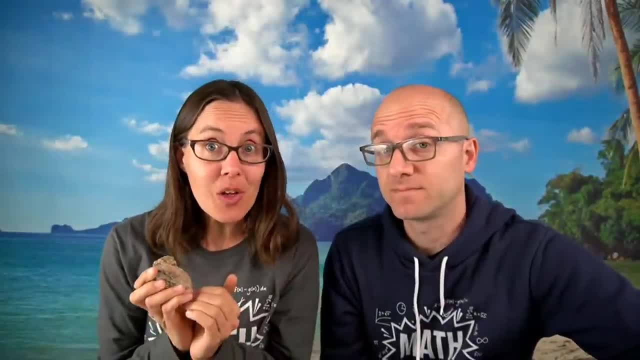 this is another question that can be kind of tricky to answer. let's go up to our big view just real quick and talk about why would we care about crystals? and it's because of the, because if the rock has crystals that are visible, that really helps us to identify. if it's a 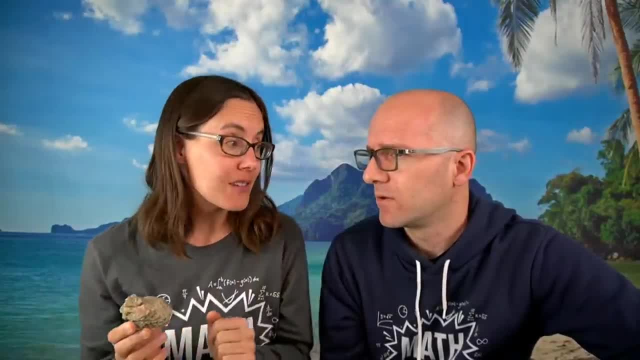 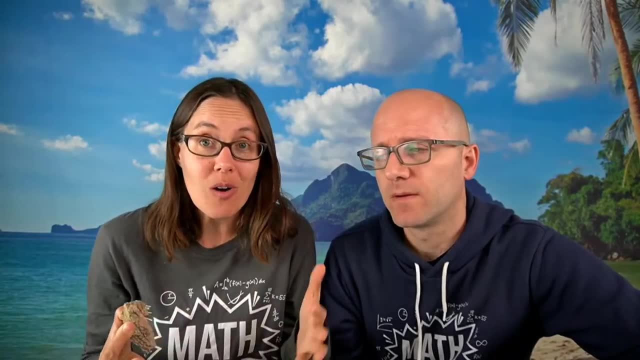 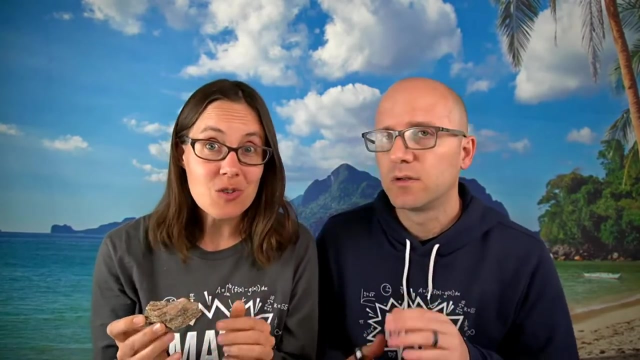 sedimentary rock or a metamorphic rock, because crystals form when you have a rock cooling down very slowly, or with a metamorphic rock. sometimes if the rock gets hot enough, pressure you can get crystals forming. but sedimentary rocks, sedimentary rocks, you're. you're going to see grains, you're not. 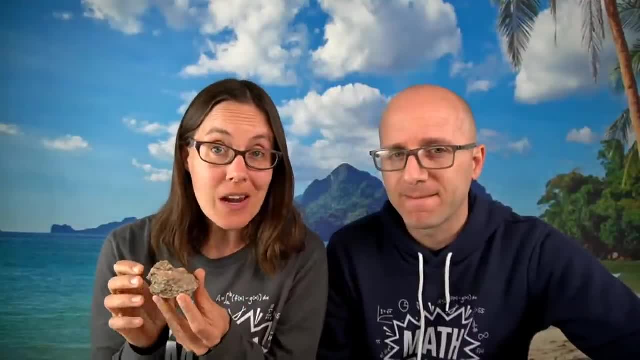 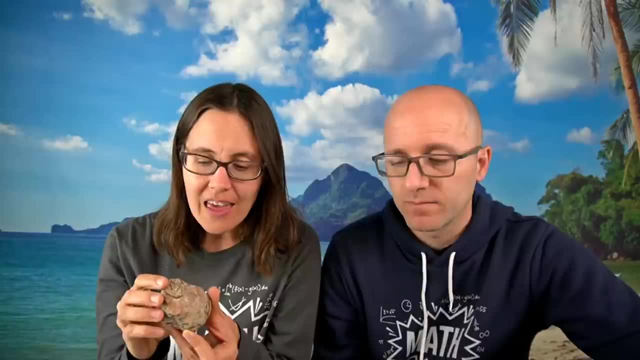 going to see. you're not going to see crystals. so for this step you actually need a pretty good magnifying glass, and you're going to need a pretty good magnifying glass and you're going to need a glass or a little pocket telescope to look and see: are there crystals and on this particular rock? 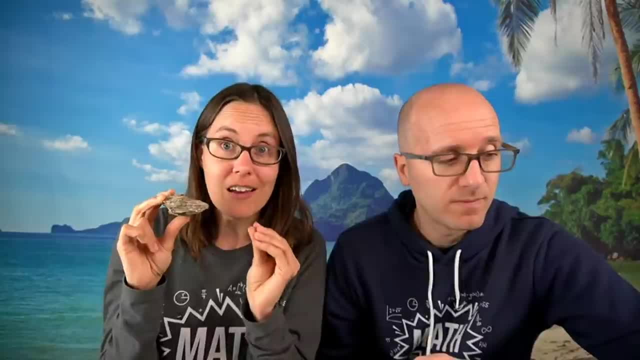 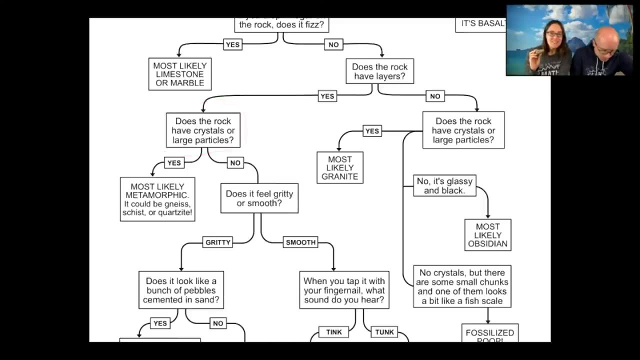 here i could see just some really, really fine crystals. so the answer is yes, all right, so does it have crystals? so the answer was yes, and it turns out this is a piece of nice, spelled g-n-e-i-s-s. it's a nice rock. i love it. 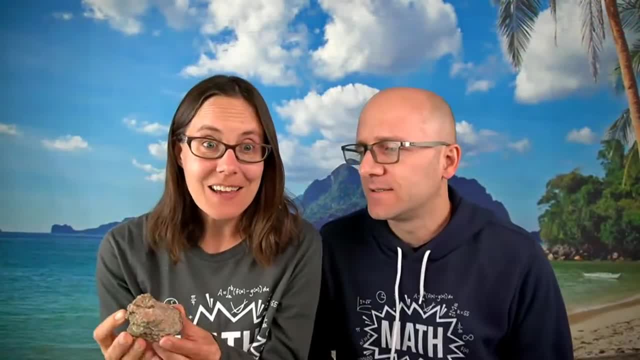 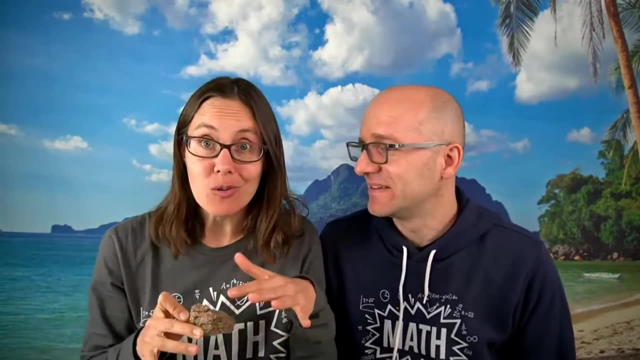 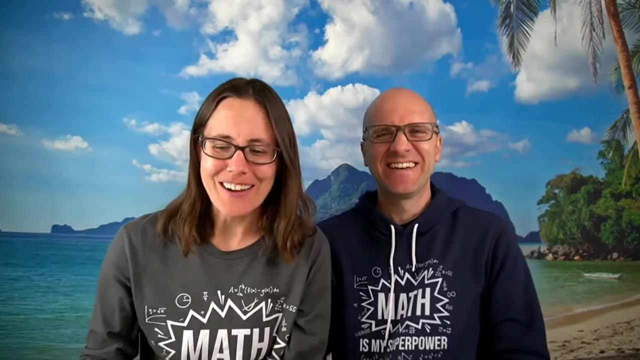 nice is a metamorphic rock and that's kind of where it gets its crystals from. this is actually granite. nice, it was a piece of granite that was then pushed deeper underground and reheated again and kind of kind of moved. so nice nice, a nice rock. that's pretty cool. so i mean this flow chart. 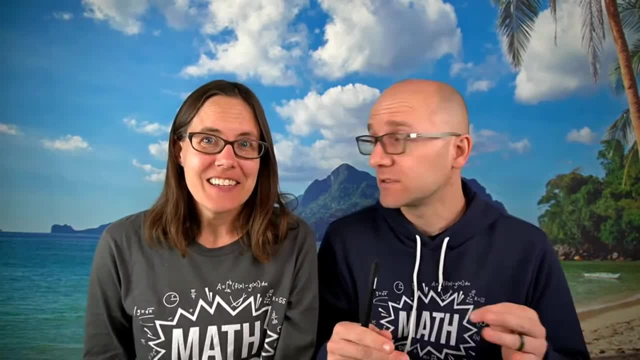 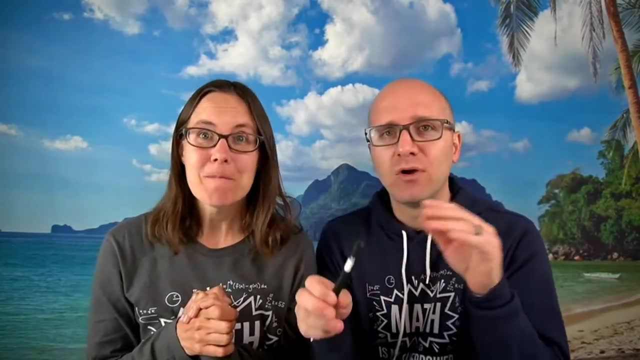 isn't comprehensive, it's not going to be perfect, but it's going to give us, it will give you- some good ideas. it will give you some good ideas. so when you get a rock, you can just follow that flow chart from one answer, one question to the next and hopefully you'll be able to identify what rock. 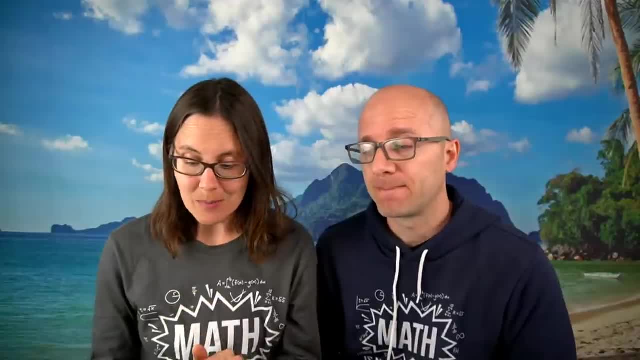 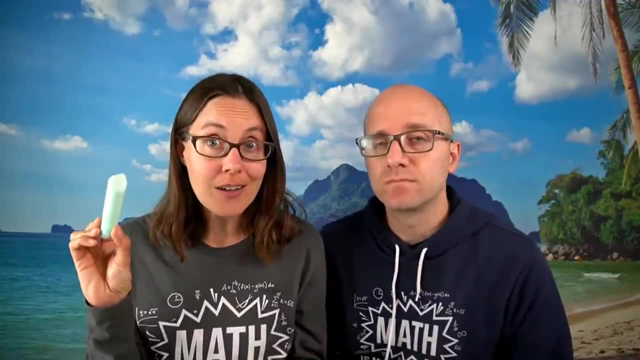 you have. i want to talk a little bit more about mineral hardness because i have here a piece of chalk and we had a couple good questions in the in the chat where people were actually asking: is chalk a mineral? and it is this green sidewalk chalk that i have right here. i would not call. 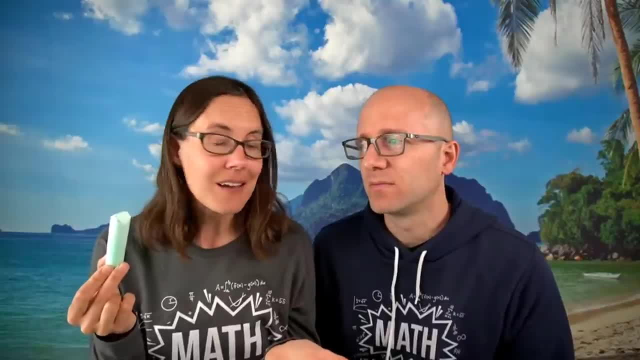 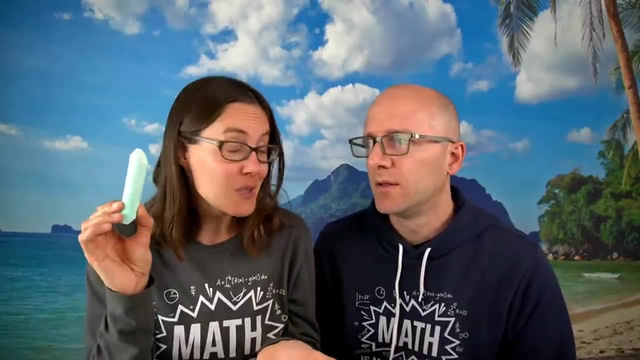 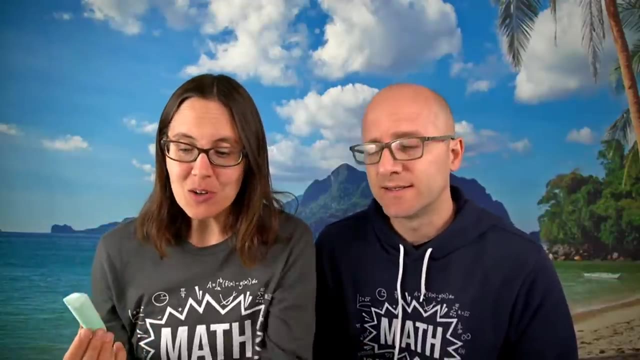 a naturally occurring mineral, because it was obviously produced and made, you know, by people. but there are natural deposits where this is really. this is the mineral: talc. that's what this is. oh, talc, is that the softest? that is the softest of all the minerals. so if i take this piece of chalk and i scratch it, 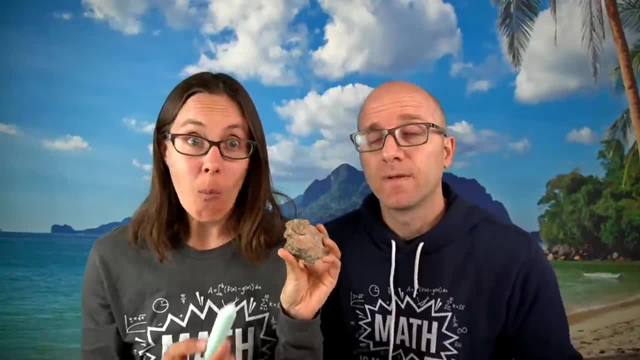 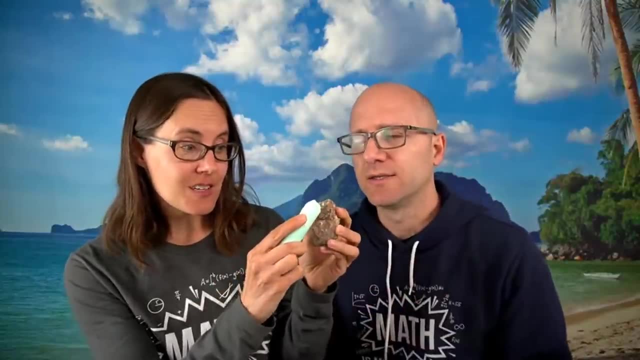 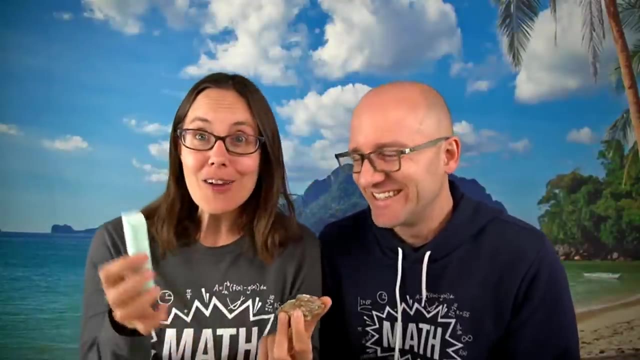 along my piece of nice. what's going to happen? the nice is going to not get dirty, but this will actually rub off. this will rub off the chalk, it's right. so i just made a streak of chalk across my nice rock. what if i do the reverse? i have my piece of chalk here. what if i scratch the nice? 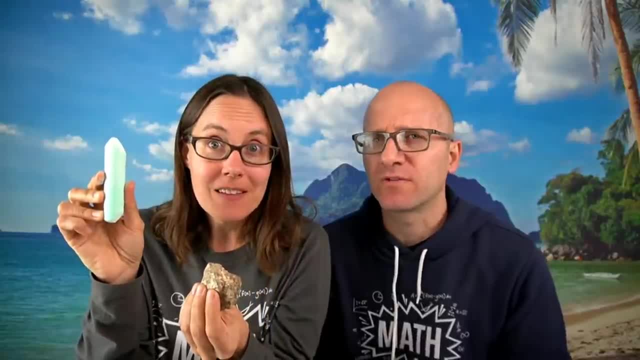 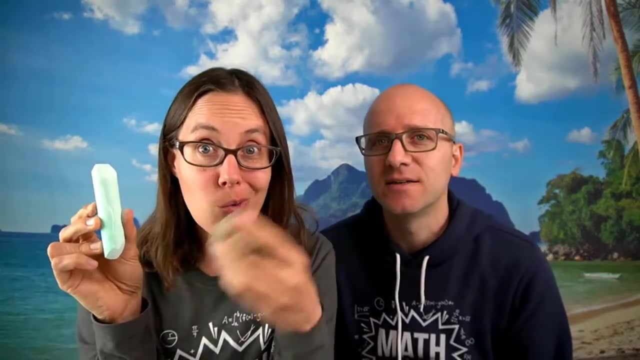 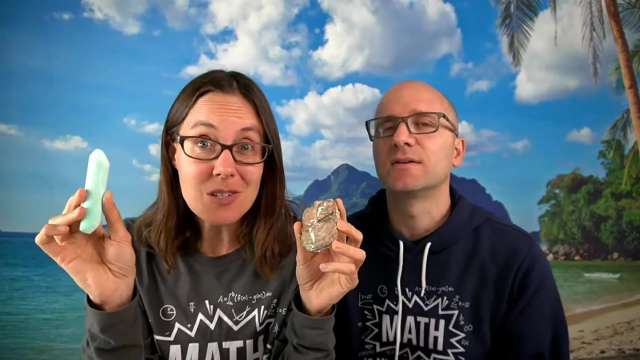 what if i scratch this rock on the chalk? well, once the same thing roughly will happen. well, it's going to make, it's going to make a scratch. oh, that see. so did i get pieces of my rock that rubbed off onto the chalk? no, i made a scratch, but if i take this, i make a streak. that means that pieces of 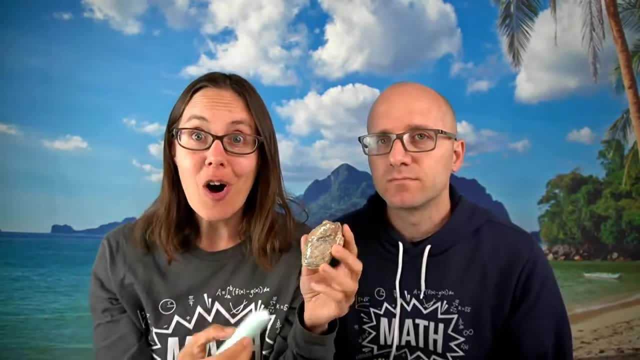 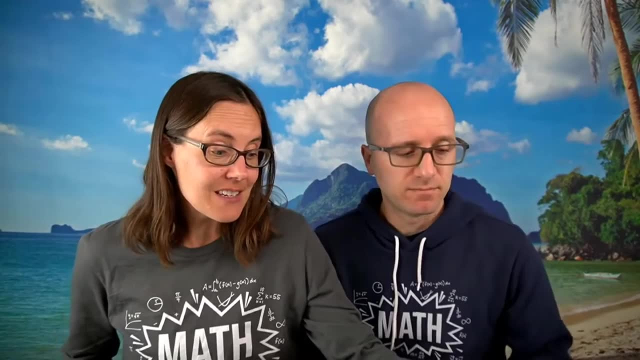 this rock because it's softer, have actually rubbed off onto my rock, and this is what i'm going to do. this is exactly how the mineral hardness scale works. there was a scientist way back when who made the mo's mineral hardness scale and he took lots of different minerals and 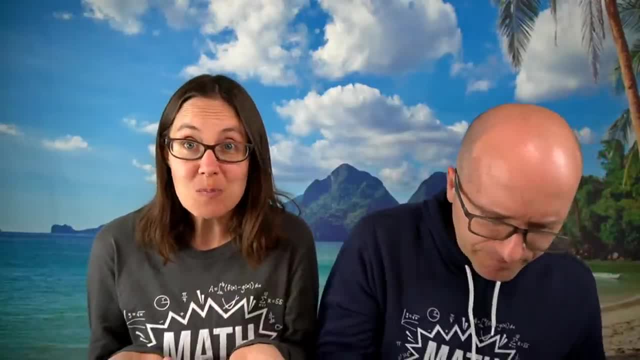 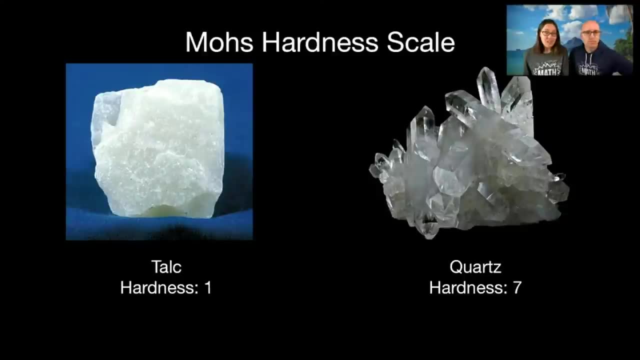 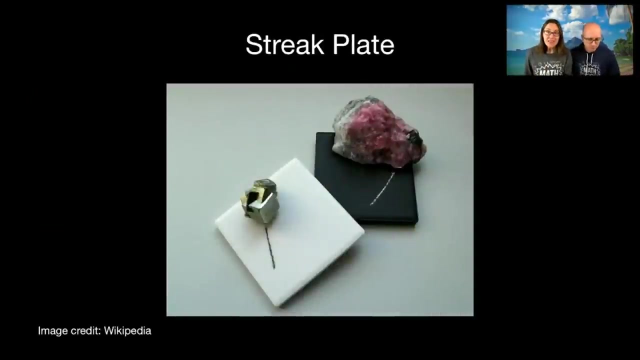 he said: you know what? we can really tell a lot about these minerals just based on how hard or soft they are. so quartz, on the mo's hardness scale, has a hardness of seven, talc the softest has a hardness of one. and our fingernail and a streak plate is super useful in. 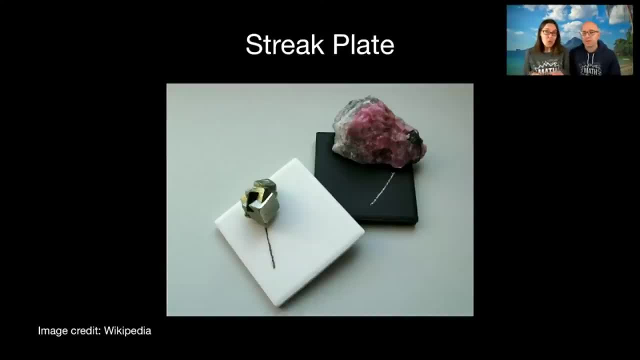 telling where you are on that scale. if you take a piece of porcelain, you can even take the bottom of a porcelain bowl. if you have a porcelain bowl at home, use that as a streak plate. if the rock leaves a streak, then it is less than seven in hardness. if it scratches your porcelain, then it's. 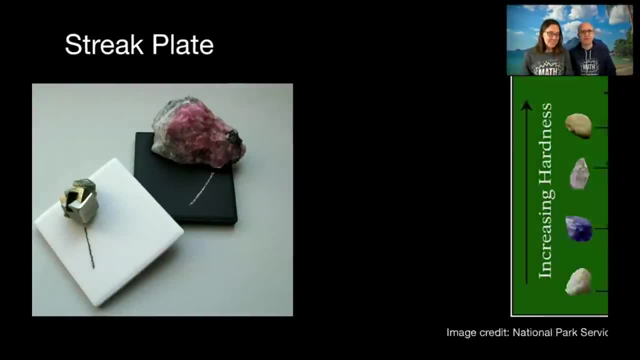 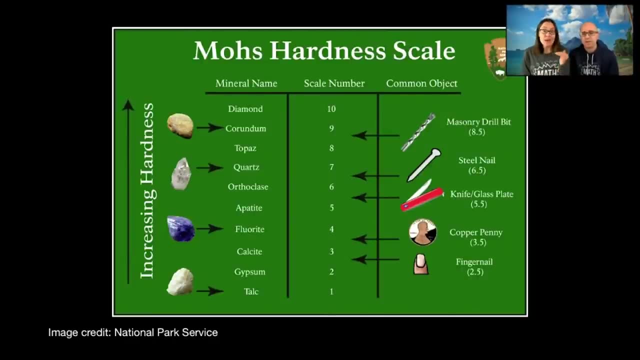 higher than seven. well, that's pretty cool. that's a really good guide right there. so let's take a look at the whole mo's hardness scale. give diamond is at the very top. that is the hardest mineral of all, and we think diamonds are valuable because we have a tradition of putting them in jewelry. 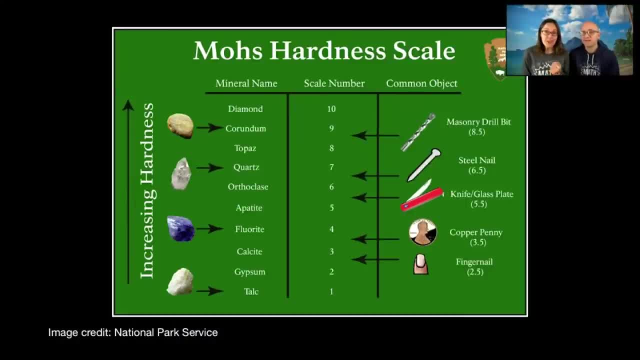 but really the most valuable use for a diamond is cutting things in industry, with machine shops and all sorts of production lines. diamond drills are used to cut things because they are the hardest thing we have to cut with pretty much. that makes a lot of sense. yeah, and your fingernail actually. 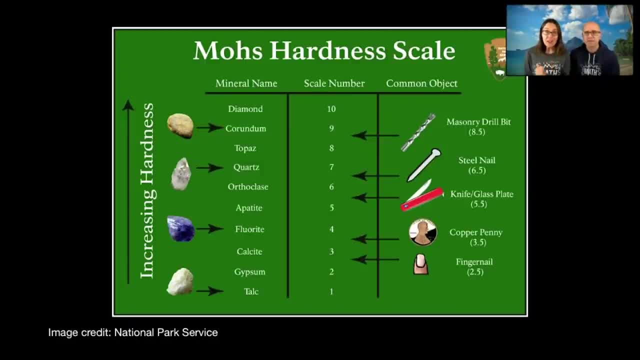 has a hardness of about two, which means that your fingernail is hard enough to scratch certain types of minerals. so that's a really good guide right there. so let's take a look at the whole mo's hardness of rock like the talc, like the talc and like gypsum. so i have a piece of gypsum here and this. 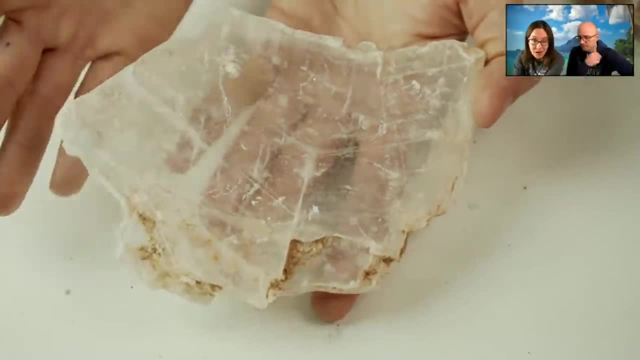 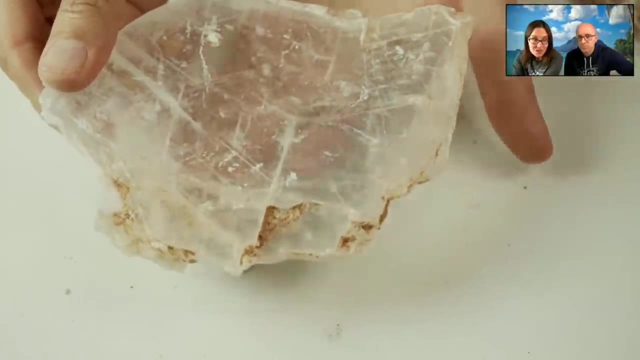 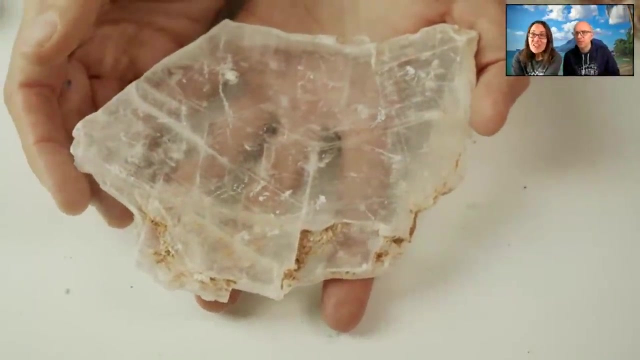 piece of gypsum actually came from near lake mead, which is right next to where i live. it is a mineral. it has a clear crystal structure and its crystal structure is so ordered you can actually see through. it, isn't that amazing? so it's so ordered. so then they're lined up in such a way that light 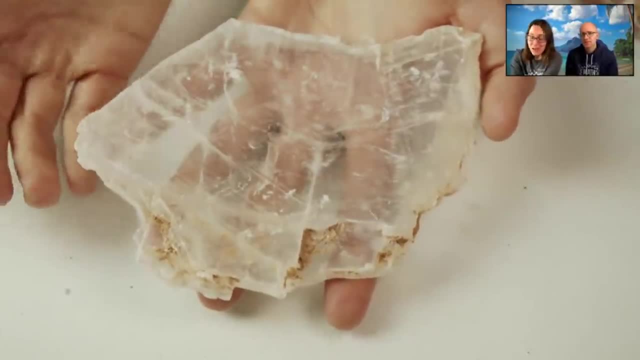 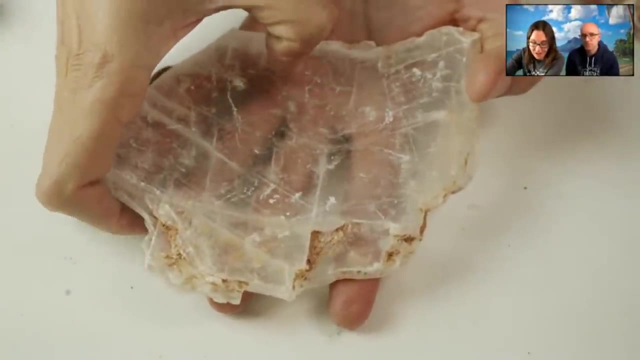 can pass. yes, the atoms are lined up so nicely that light can just pass right through. and this plate right here, if i just take my fingernail. my fingernails aren't too long, but they're long enough. if i push down i can scratch. don't do it. i can scratch the surface of this because it is so. 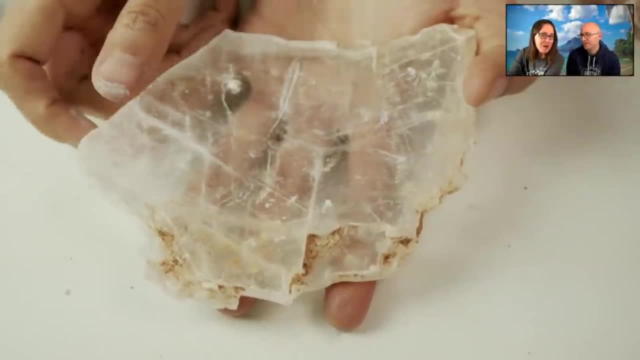 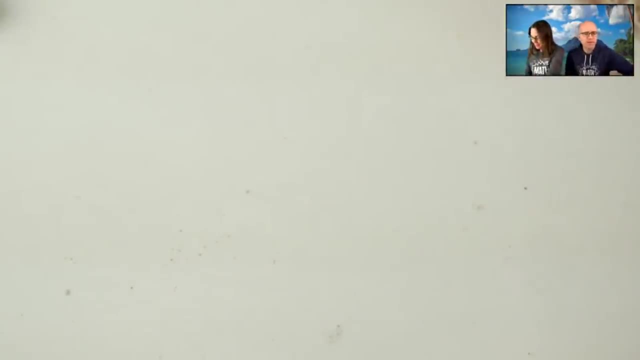 soft and, don't worry, matt, then we can. we can polish that off later if we want to. all right, all right. he said this one was called what this is, gypsum. oh, that's gypsum. oh, that's interesting, because when i think of gypsum i usually think of like sheet rock. so in most people have walls. 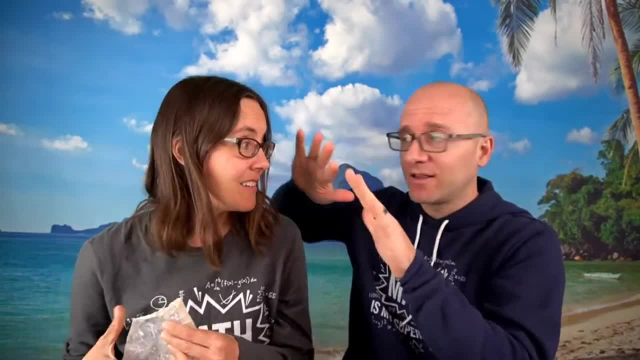 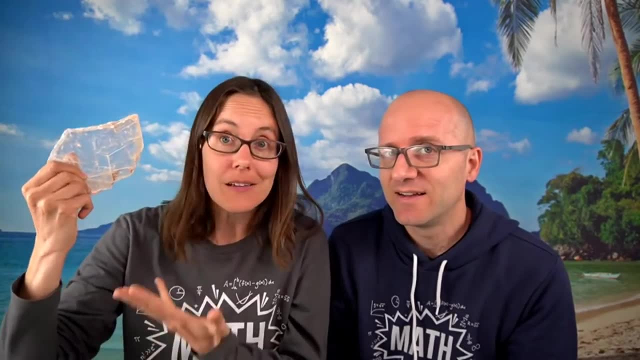 with sheet rock behind the paint, and that sheet rock is made of gypsum, and it's it's made of material, just like this. so gypsum occurs naturally out in nature. it is deposited and we go and we harvest it and mine it and then grind it up and use it to make sheet rock. so that's probably the 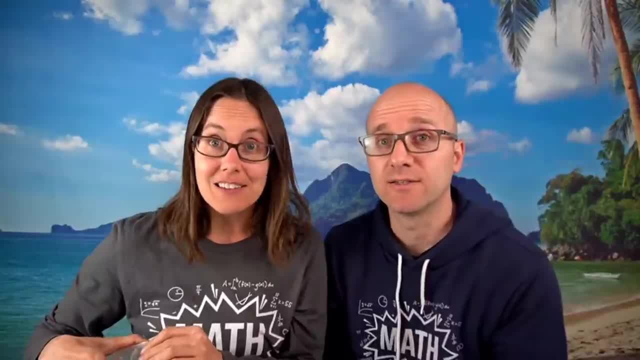 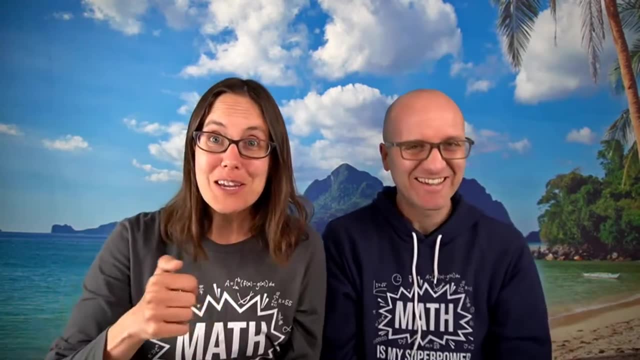 strongest thing that our nails can scratch on that most hardness. yes, yes, all the other rocks. if you try and scratch them with your fingernails, you'll end up filing your fingernails instead, you'll leave. you'll leave a little streak of fingernail on the rock, because the rock is strong and it's. 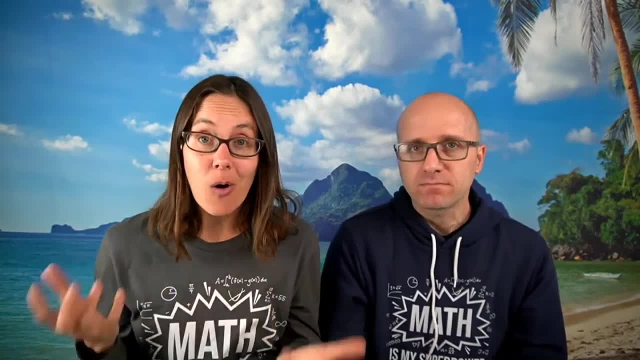 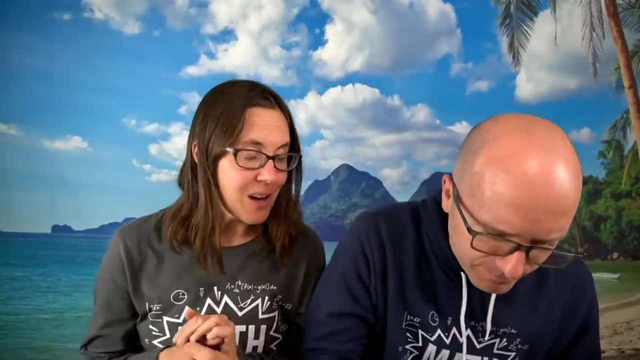 stronger. so a streak plate is super useful in telling how hard a mineral is and then, of course, looking to see: are there crystals? now let's, let's go, look back. i want to talk about four minerals and then we'll have our where in the world question and we'll go to our questions for you. 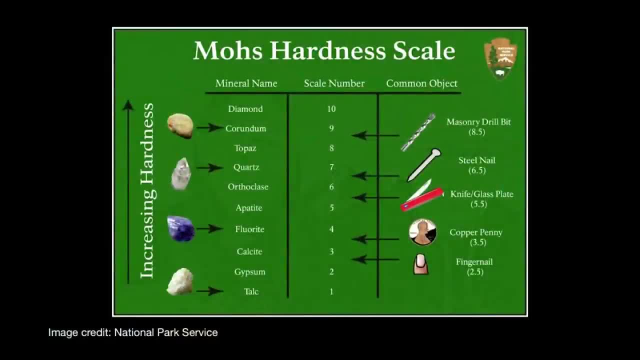 guys. so if we can go back to the notes real fast, okay, oh, do you want to say? i just wanted to take take another look at this because i think this is so cool. so yeah, we've got talc, gypsum, calcite, apatite, orthoclase- i've never heard of that. quartz topaz corundum- that's the emerald and ruby. 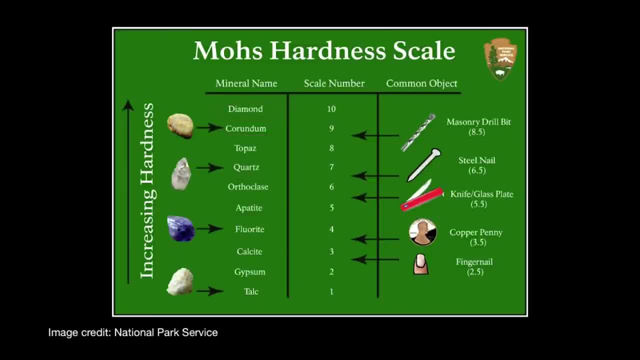 yeah, yeah, and then diamond ruby- sorry, i said that wrong. oh, yes, yeah, it makes me wonder where emeralds or other gemstones fall in here, things like pearls, but um yeah, so steel nails fall in here somewhere. a glass plate somewhere between a five and a six, a copper penny somewhere between 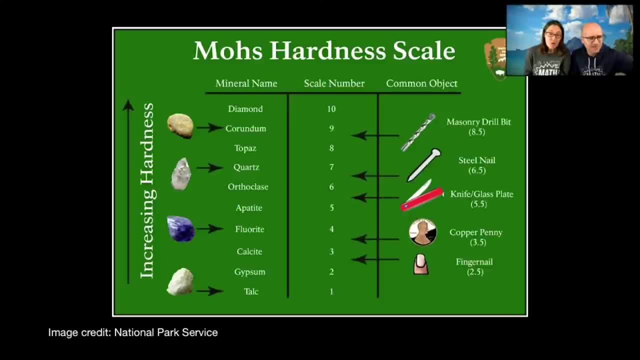 a three and a four, so a copper penny is actually somewhat soft compared to the other items on this list. yeah, i usually think of coins as really strong, but all depends on all depends on the coin. yeah, all right, let's pull up the notes. we're gonna just 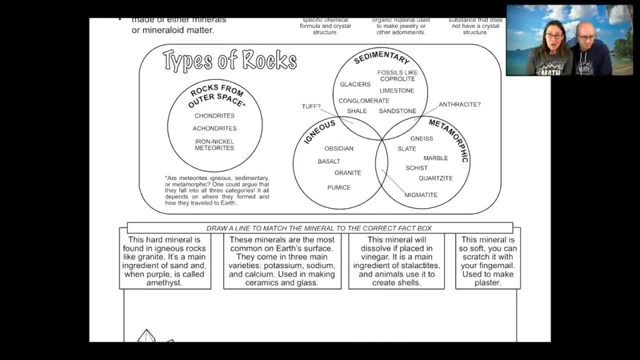 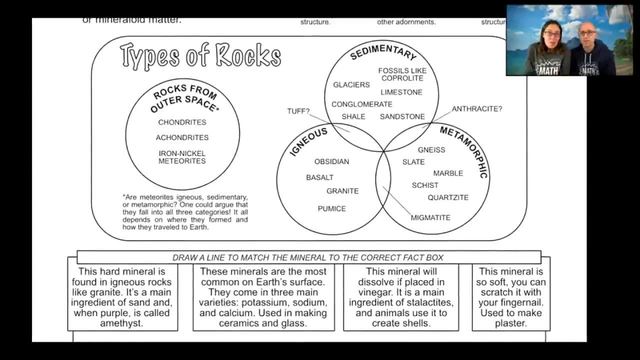 come down here real quick on this page 81, because sometimes we think of rocks as just being in neat categories like that. all rocks are either sedimentary, metamorphic or igneous, but some rocks kind of fall in between. so coal is a sedimentary rock made by, you know, ancient. 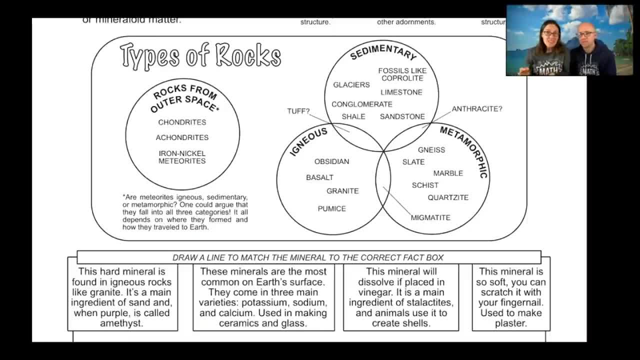 material that got squashed down to a layer. but if that coal is heated enough that it really becomes compact, you could argue that it's a little bit in between sedimentary and metamorphic. not every rock fits into each category, and this rock that i have right here, this is a small rock, but math 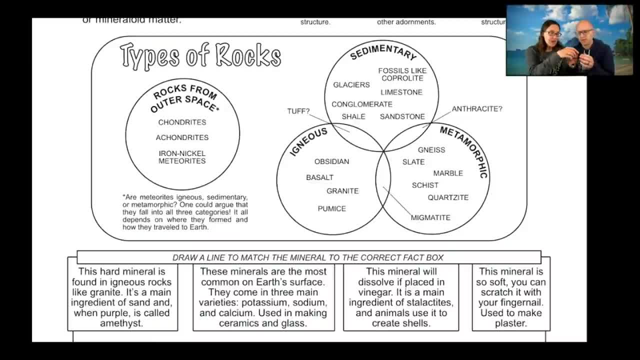 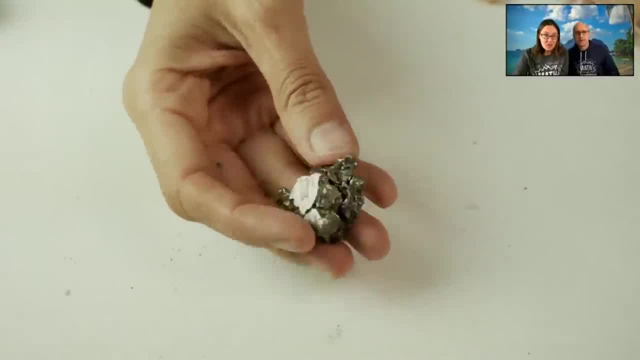 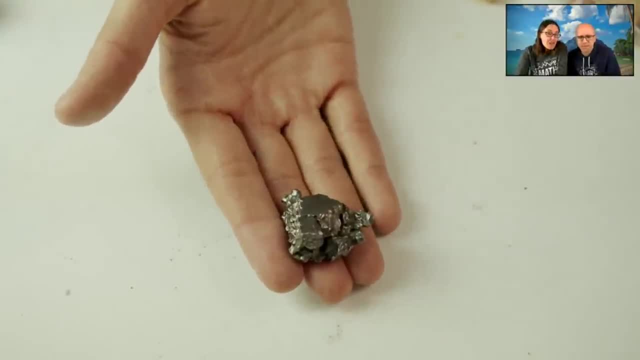 that i want you to hold it real fast. that's kind of heavy, it's really heavy. and then let's, let's look at this close view so i can show this one off. this is an iron nickel meteorite, a small piece that it fills way heavier than any natural rock and a meteorite. is that a sedimentary metamorphic or? 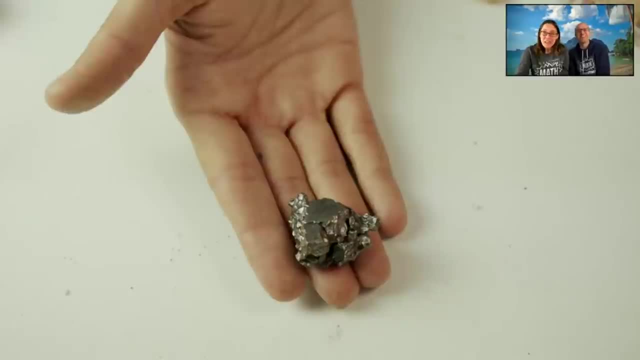 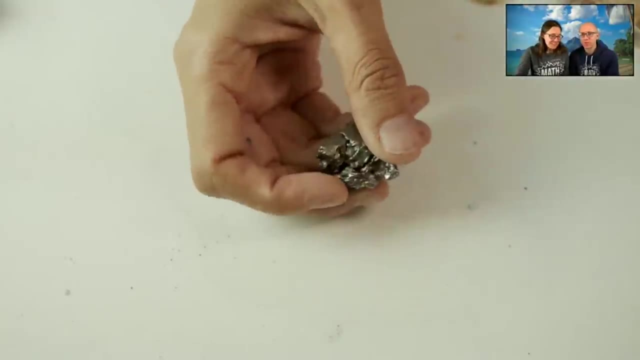 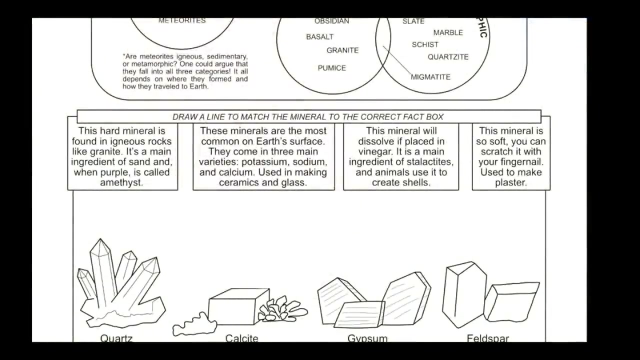 igneous rock? well, it all, it all depends. you could actually make an argument that it's any one of those, depending on where it came from and what type of meteorite it was. wait, what about moon rocks? moon rocks are all going to be igneous pretty much there. we don't have the sedimentary you. 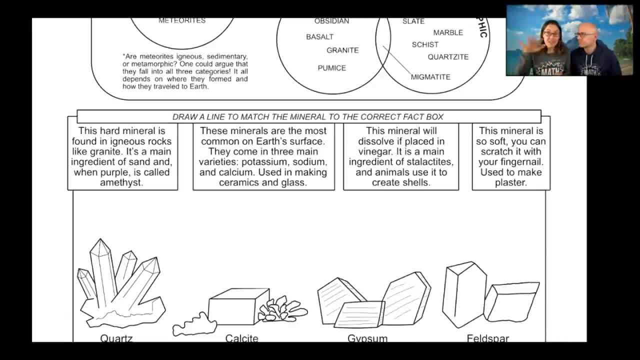 know you don't have sediment on the moon that is cycling in layers and compacting, you don't have water moving through to cement sedimentary rocks together and you don't have plate tectonics to heat up metamorphic rocks. so all the rocks on the moon are igneous. but 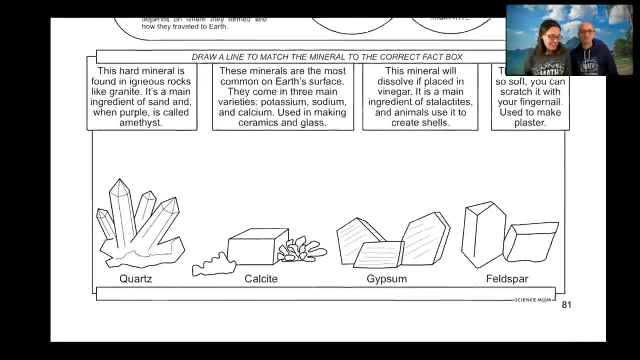 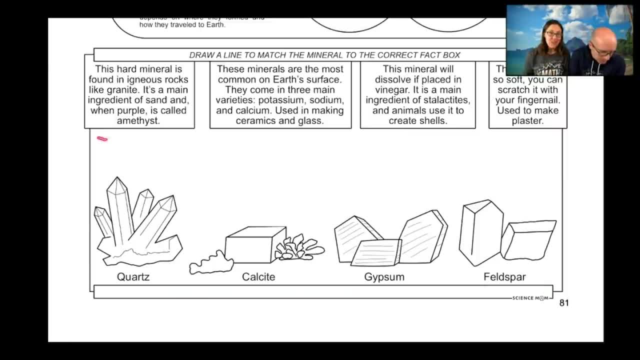 they've been cooled down for a long, long time. let's look at four minerals real fast and then we are going to get back to our where, the world mystery and our questions. all right, so this hard minerals found in igneous rocks like granite. it's a main ingredient of sand and when purple, it's 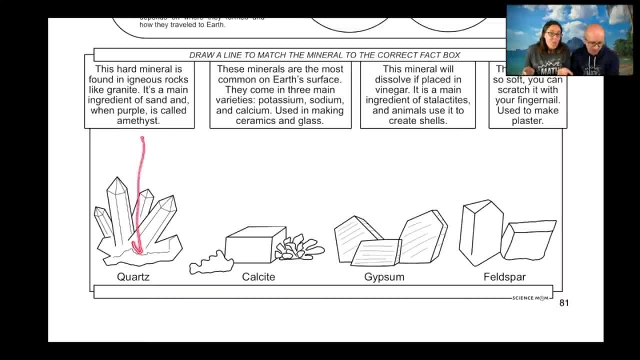 called amethyst. oh, that's just going to be straight down to quartz. right, that is quartz. and adaline asks: why is quartz so common? it is one of the most common minerals and it's because it is so resistant to erosion. it just stays around because it's so hard. it's a seven on the hardness scale, which actually means 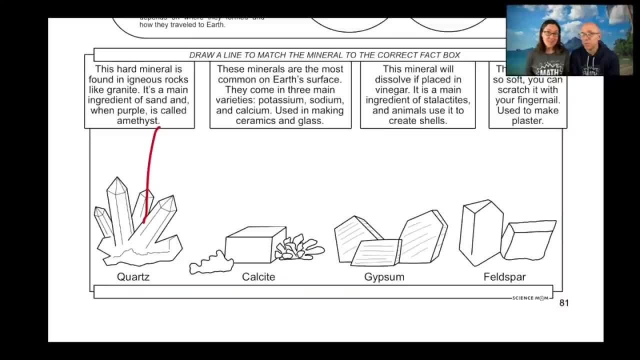 it's a hundred times harder than talc is right, all right. these minerals are the most common on earth's surface. they come in three main varieties: potassium, sodium and calcium used in making- and i have a hint right here- oh, these two varieties that i showed earlier. this is feldspar. yes. 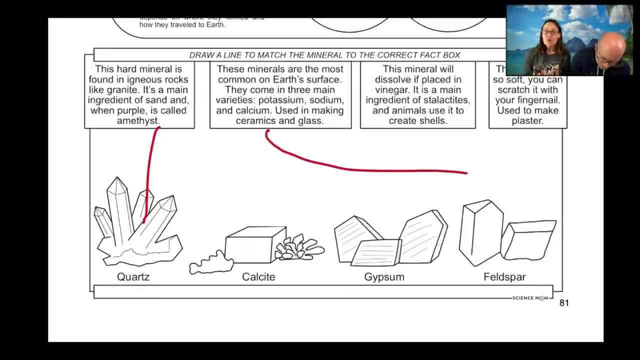 feldspar is actually the most common mineral on earth. there are so many different varieties of feldspar and, like you saw, from looking at these two- the labrador feldspar and the other one- it can look really different depending on what it is. that's. that's really interesting. i'm curious. let 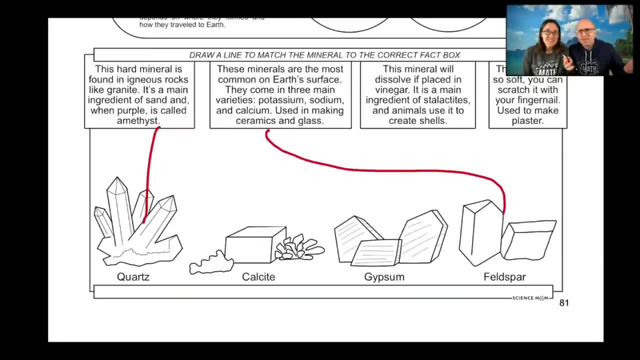 me know in the chat, have you even heard of feldspar before? that's? that's not a very commonly used term. up next, this mineral will dissolve if placed in vinegar. okay, so that was calcite, that is calcite. and then, last but not least, we have the mineral that i scratched and that your sheet rock is made. 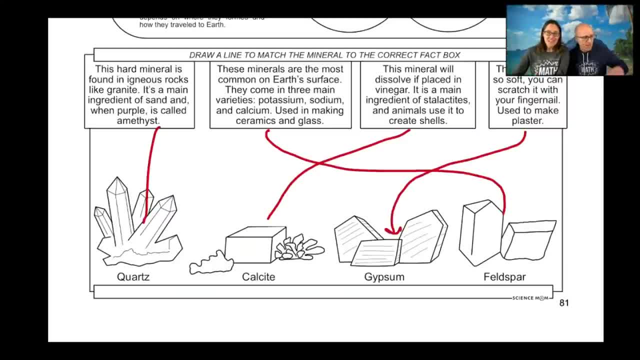 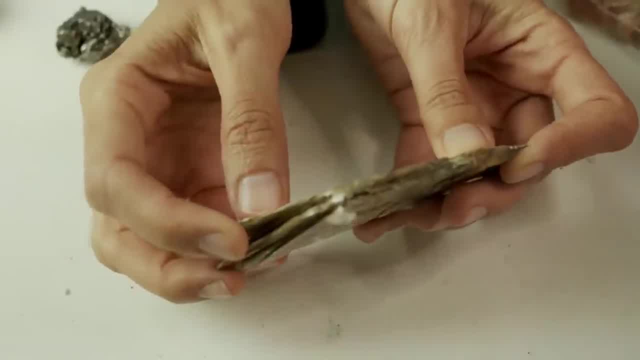 out of so soft you can scratch it with your fingernail. that's right. gypsum. and last little one i want to show you. this is mica and it has such such dramatic layers that flake off so easily. there was a mica mine in nevada. 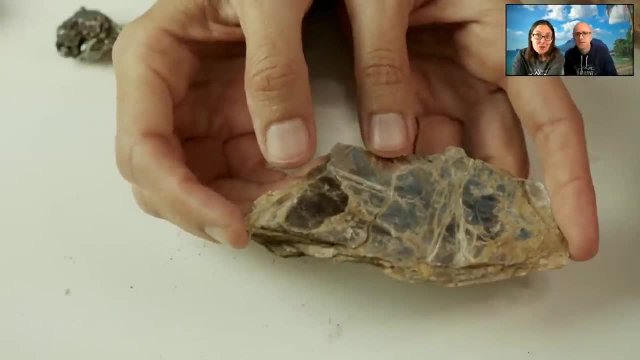 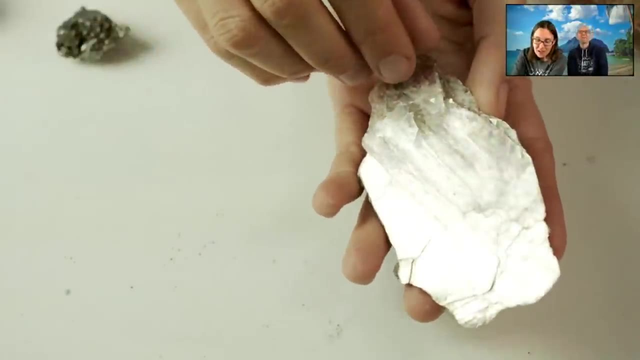 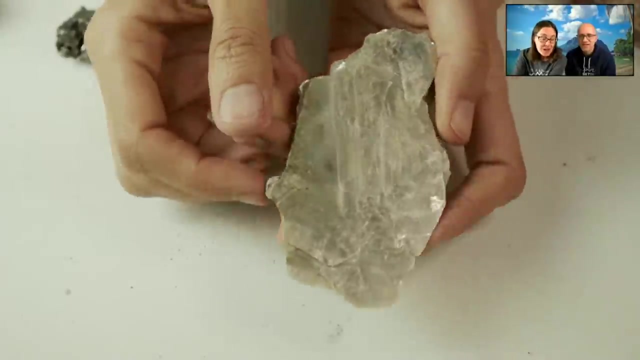 that was located several hours drive from here, and in the early 1930s, at this mica mind, people made windows out of mica. they would take a large piece of mica and they would carefully peel off one of these pieces and if they got it small enough, it was translucent. light would pass through. 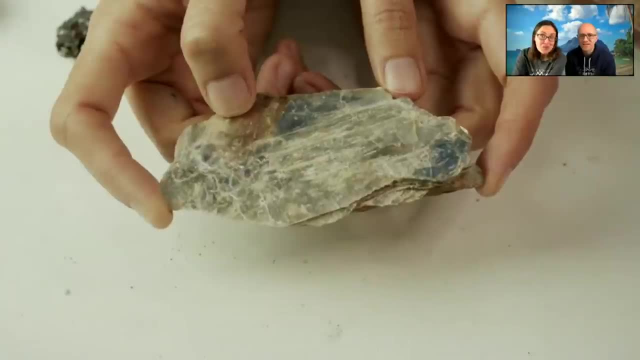 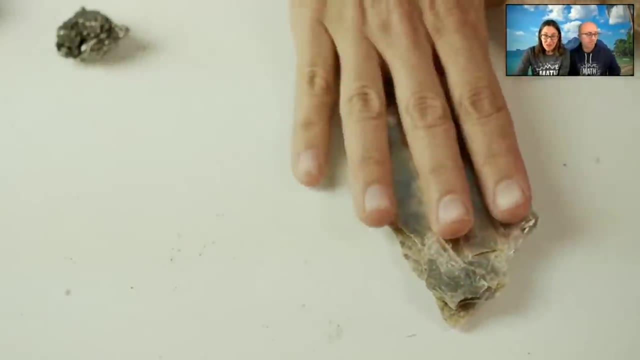 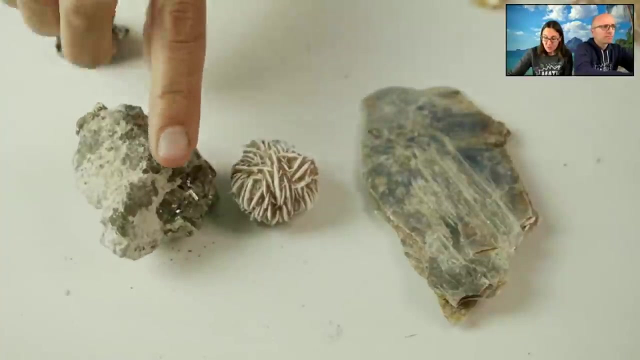 and that's what the miners used to make windows in their in their homes. whoa kind of crazy right? yeah, it is so. there are so many different cool types of minerals, from mica, which comes in sheets, to selenite, which has this beautiful rose-like pattern, to pyrite, also known as fool's gold, and on and on. 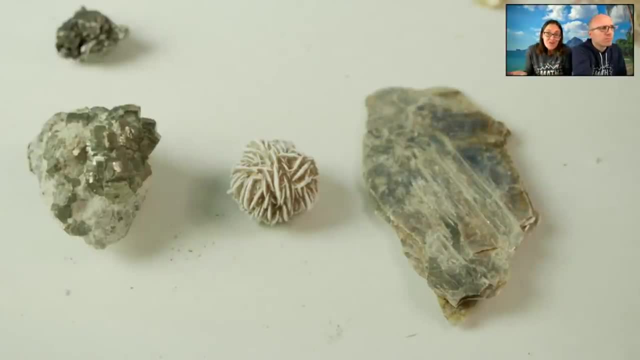 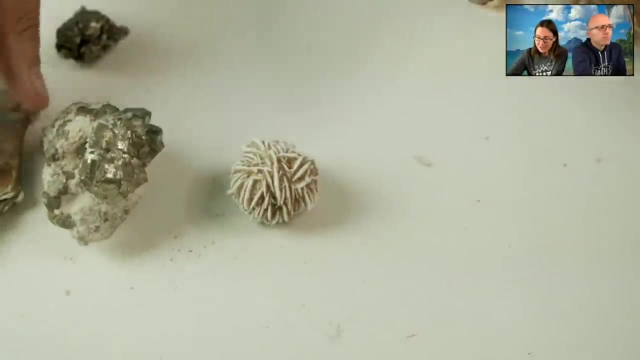 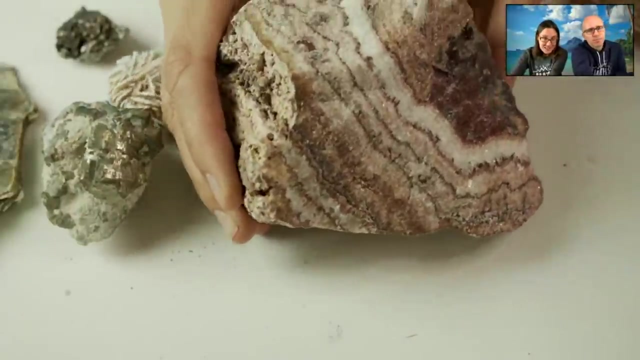 i hope this just gives you kind of a fun taste for how, how much variety there is with rocks and that you enjoy exploring and learning more about them. and one last little example: calcite has so much variety. this is a piece of banded calcite that our friend, who's a geologist, lent to me, isn't that? 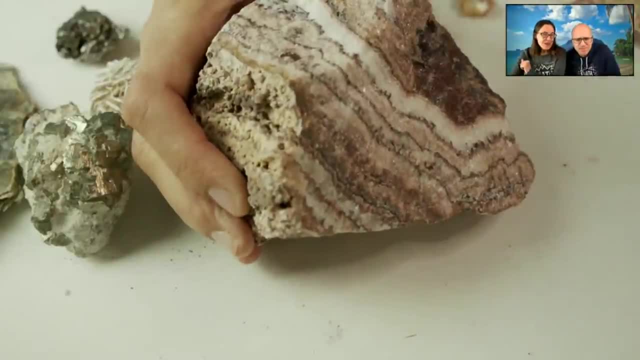 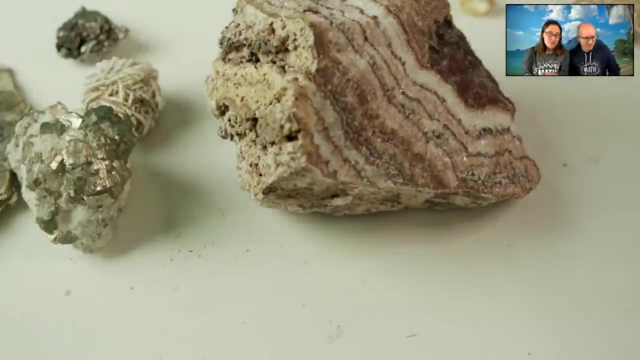 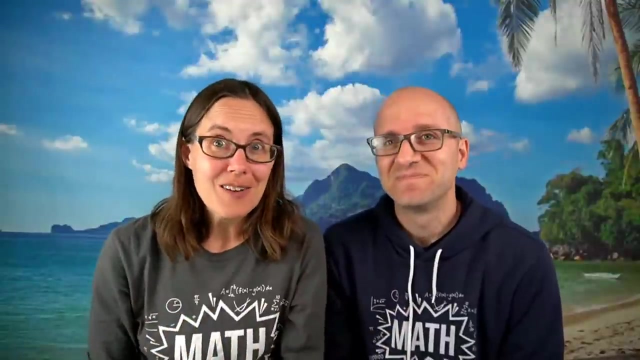 beautiful. oh yeah, it's gorgeous, but this is kind of a rare specimen. most calcite looks completely different from this and the little drawing that i showed. we saw that sometimes it can be kind of cube shapes. sometimes it can form beautiful little um structures. calcite has a lot of variety, all right. 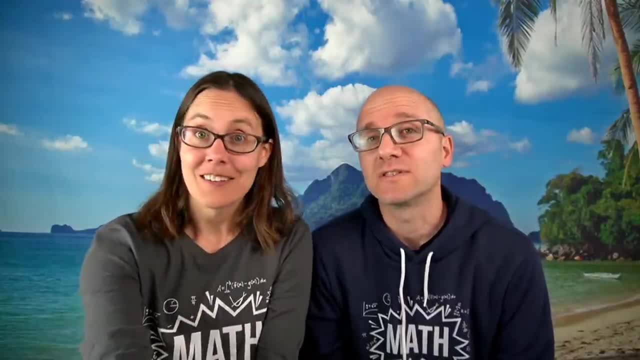 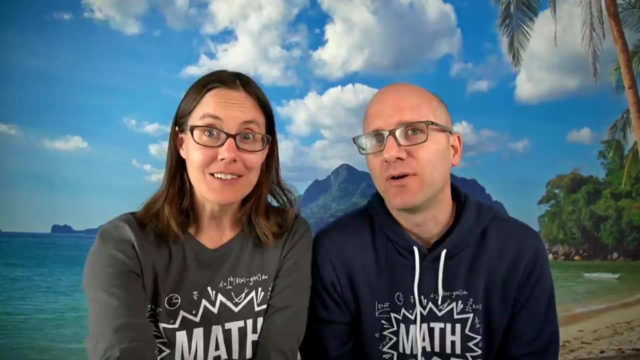 one question for you, science mom, before we even get to the poll questions. there was one type of mineral that gets used in baby powder, or at least was at one point talk talc. that's right, i do. i do talc, talcum powder. yep, all right, you ready for the? where in the 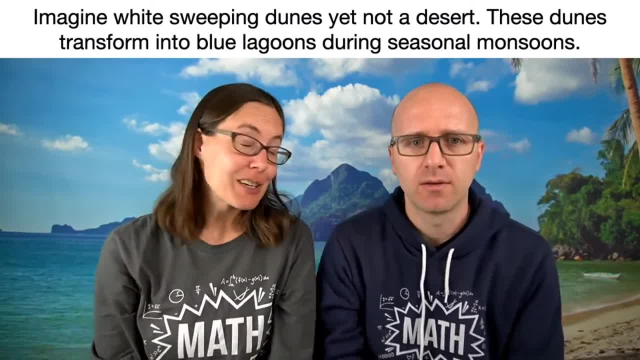 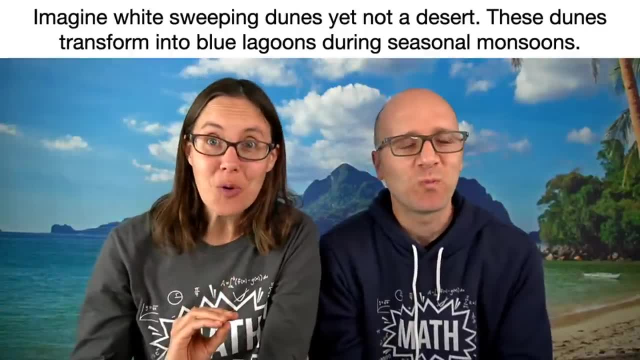 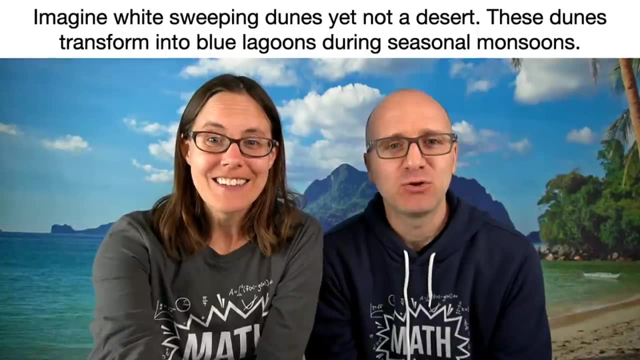 world mystery math dad. oh yeah, i'm ready. this one's a tough one. i don't think you're gonna get it. okay, imagine sweeping white sand dunes, but this isn't a desert. these dunes transform into blue lagoons during seasonal monsoons. do you have any ideas? lagoons? let's see the monsoons. okay, so 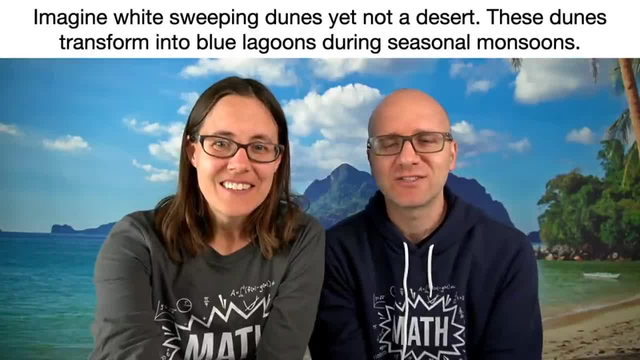 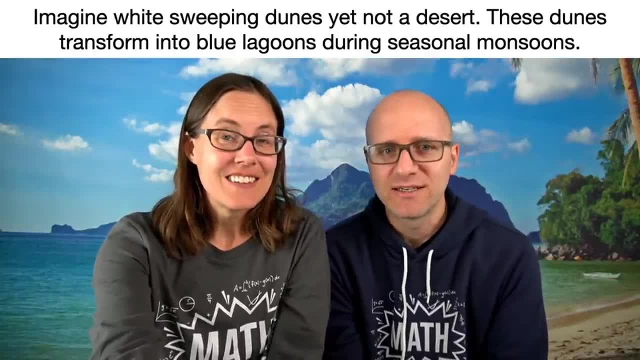 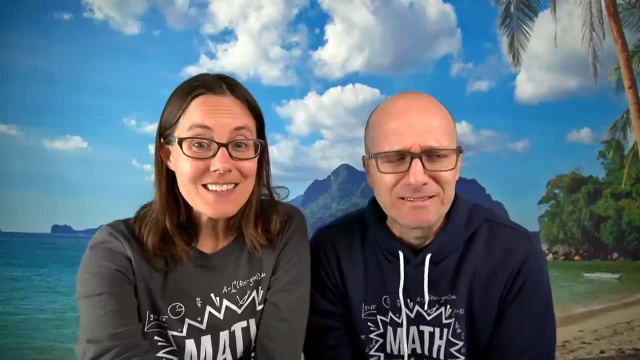 it's somewhere with sweeping dunes, so somewhere extra sandy, but it's not a desert. it's not a desert. it'd have to be a beach, and you're talking about blue lagoons, so that makes sense. is it right behind me? it is not right behind you, um, so this is a national park in brazil. 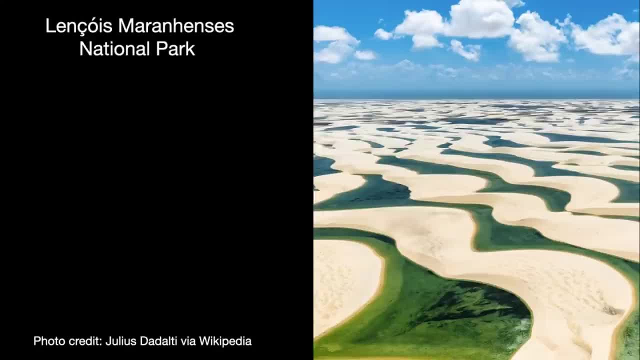 called um and it's a little difficult to pronounce. i wrote myself a tip. l'inspoir marines national park- okay, i have never heard of that. that. it is beautiful, beautiful, and the reason why it looks so amazing is because there are sand dunes and then underneath that. 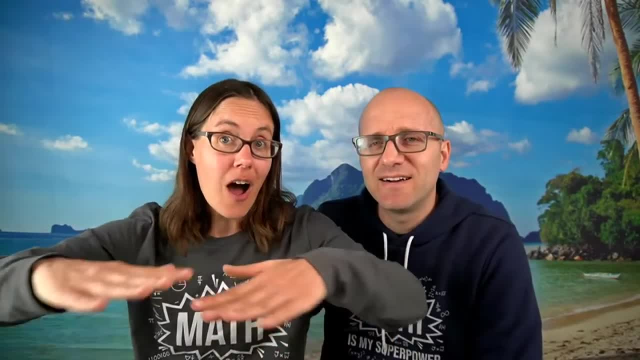 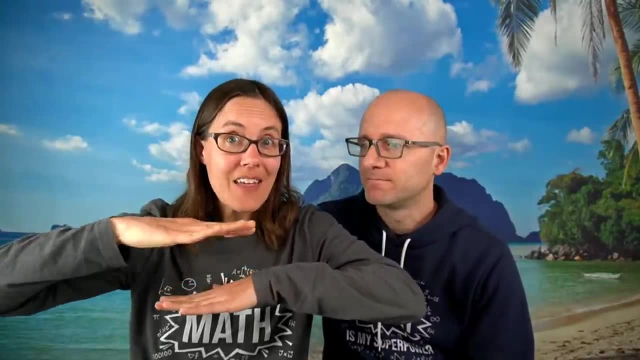 layer of sand, you have igneous rock that is not permeable. that means the water can't go through it, and so when it rains, the rain goes and kind of hits those sand dunes and then just stays there and it takes a while before it either soaks into the sand or evaporates or slowly runs to the ocean. 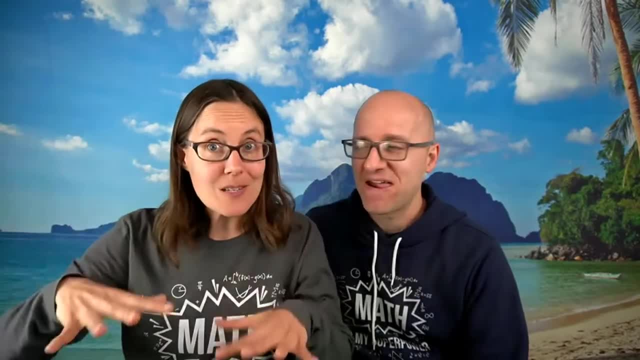 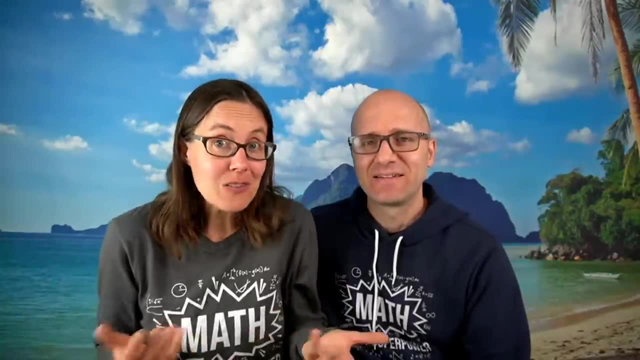 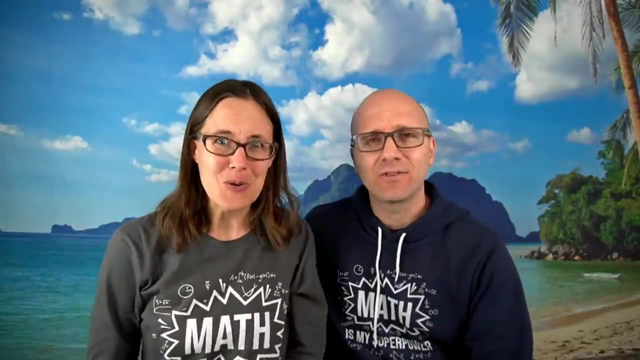 and it doesn't get very much rain. just once a year they'll get these monsoon rains that dump a lot of water, and then the rest of the year it's dry. a really cool environment and caused in large part by the geology, by the sand and then underneath a layer of rock that is not permeable. yeah, i don't know, i don't. 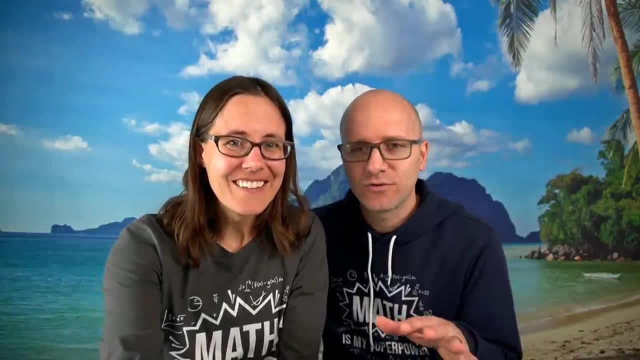 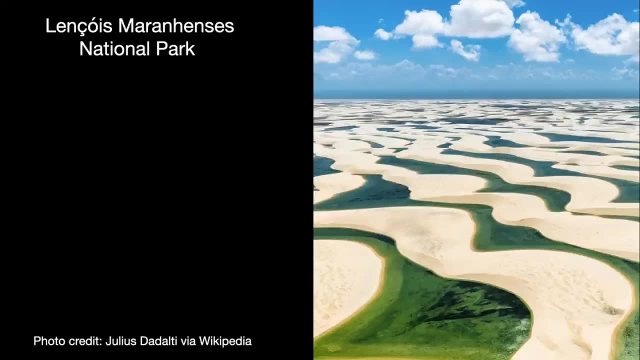 even remember seeing pictures of that before, but that was really neat. yeah, you throw it one more time. yes, i'll grab it one more time. there it is l'inspoir marines national park. it is in brazil, up near the sort of the top of brazil, nice. and now we're ready for poll. questions go to. 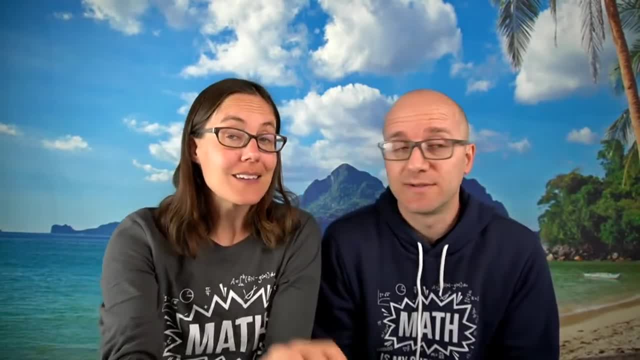 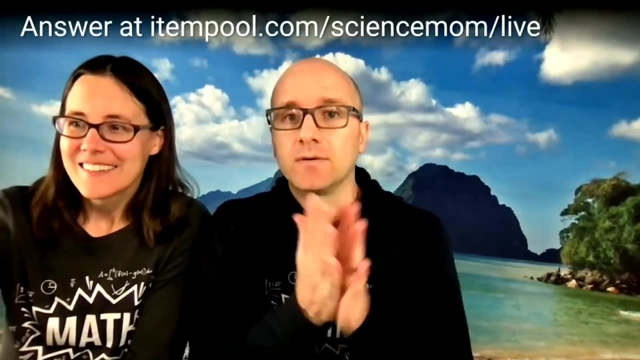 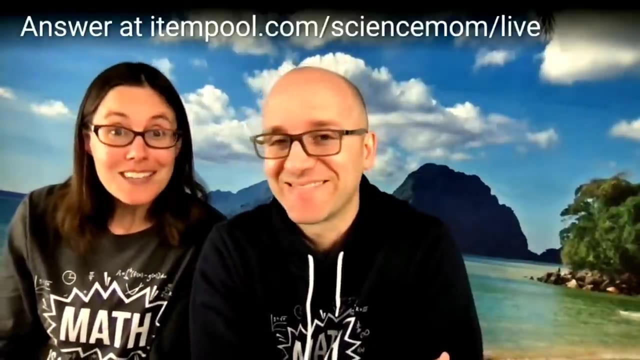 itempoolcom science mom, or if you're watching the replay at sciencemom, you can click right below the thumbnail and it will bring up the poll questions. all right, do we have some birthday shout outs today? we do have some birthday shout outs. a very happy birthday to katya, who turns 12 today. happy birthday, katya. 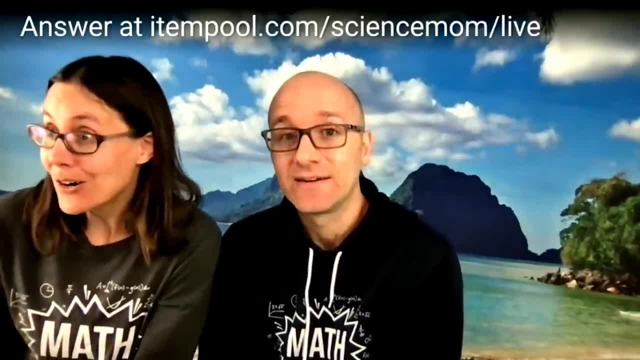 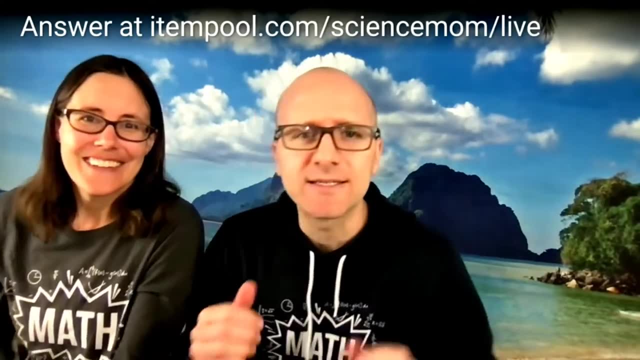 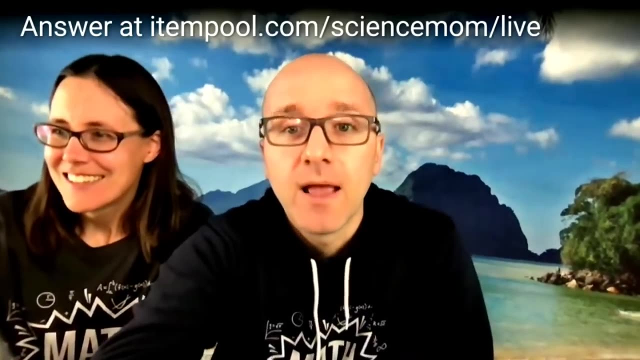 and a happy birthday to emriah tomorrow. woohoo, and lila from colorado turns 10 today. happy birthday, lila, or lila, i'm not quite sure how to say your name, but happy birthday, all right. was i looking at the wrong camera? math dad, right right? whoops, we're here. so 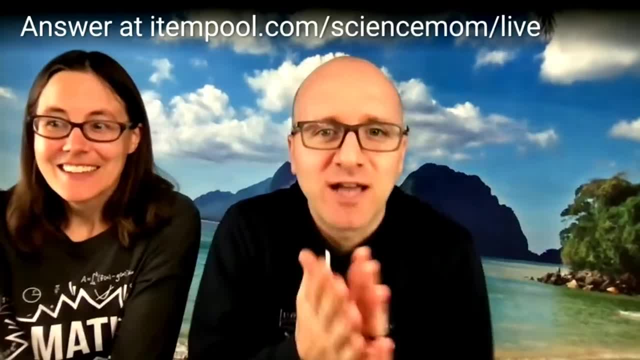 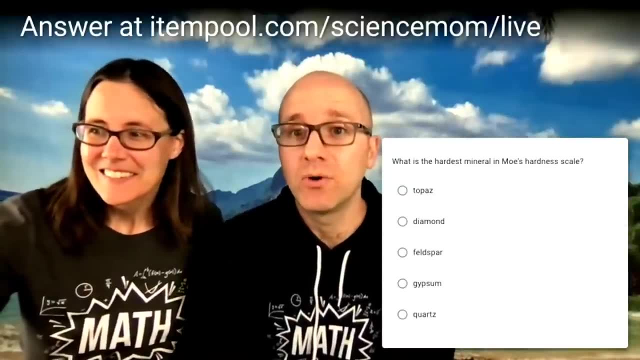 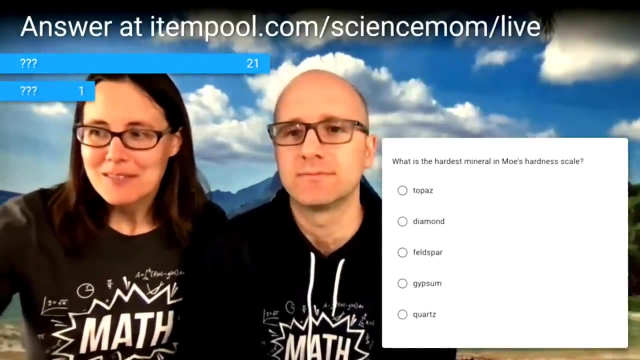 that's a birthday present. i'm gonna crush you guys. that's what math dad thinks, but i don't think so. all right, first question: what is the hardest mineral in mo's hardness scale? and i totally spelled mo wrong, didn't i? m-o-h-s. that's okay, math dad, the unbeatable science, kids are very. 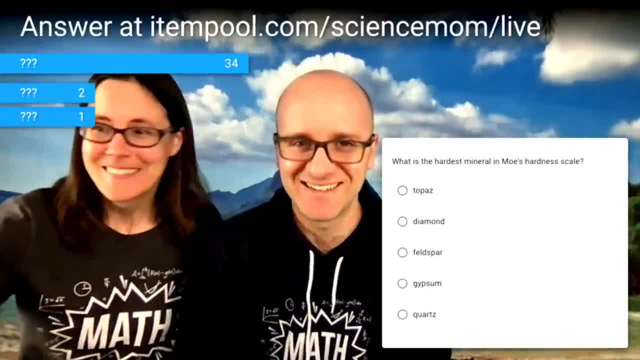 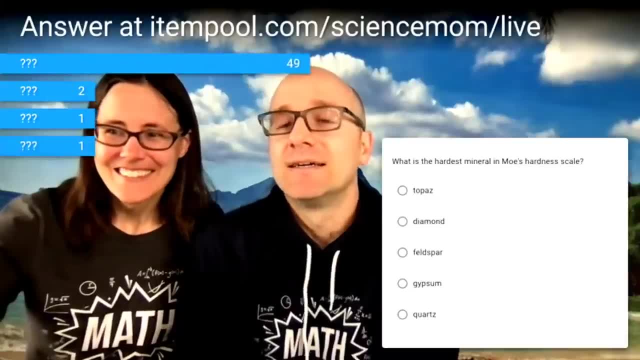 forgiving because they, they win every time. all right, and i didn't mean i would crush you on this question. i know you're going to get this one right- most of you. but what is the hardest mineral? and when we say it's the hardest, the most mineral scale it. 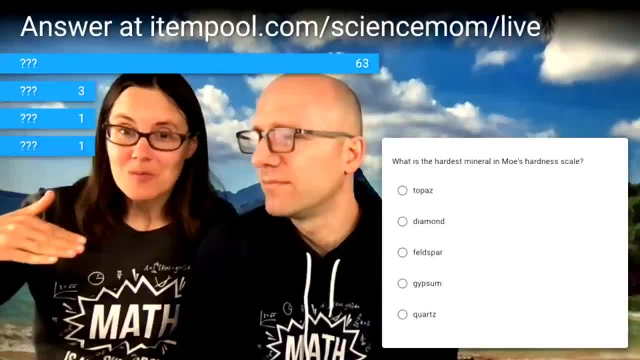 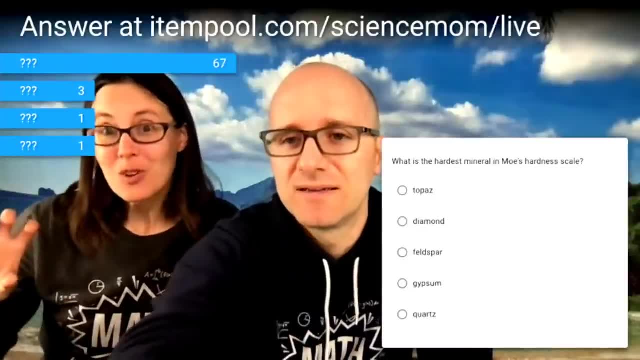 doesn't go like. a two is twice, you know, is a little bit harder than a one, and a three is a little bit harder than two. each time it just about doubles. oh wow, so the hardest mineral is actually one thousand five hundred times as hard as the softest. that's pretty cool, all right. and the 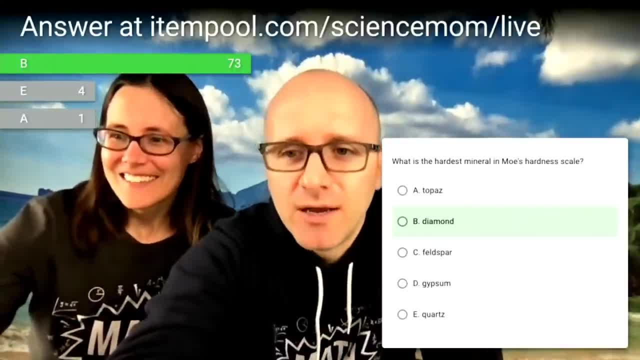 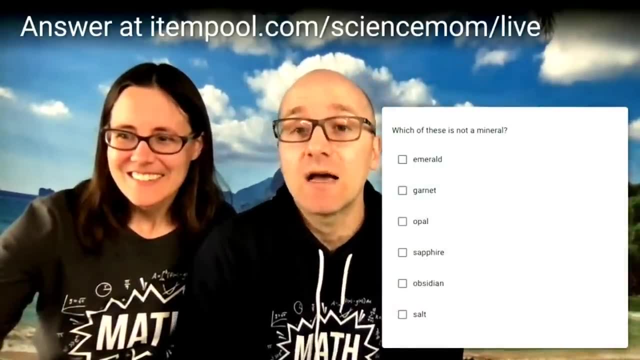 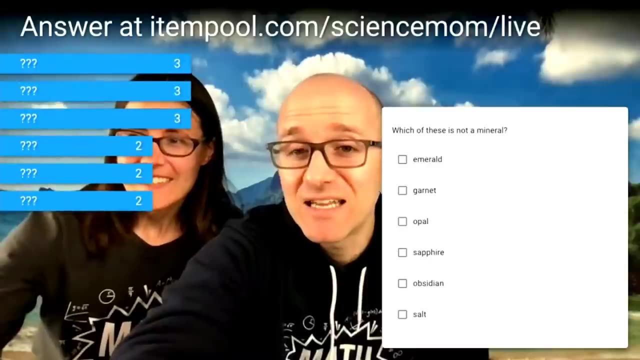 second one is a diamond. all right, nicely done. many people on that one. all right, gotta build you up before i crush you. question two: which of these is not a mineral? so select all that apply. we've got emerald, garnet, opal, sapphire, obsidian salt. select any of those that are not minerals. 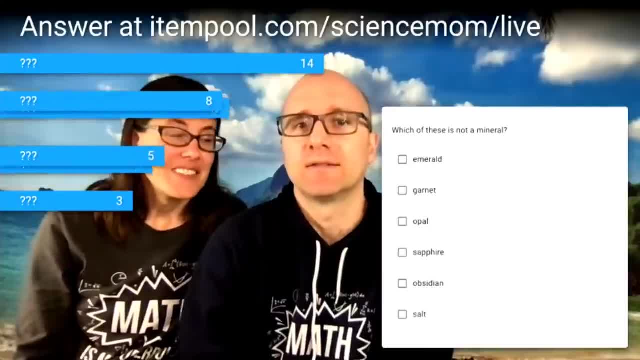 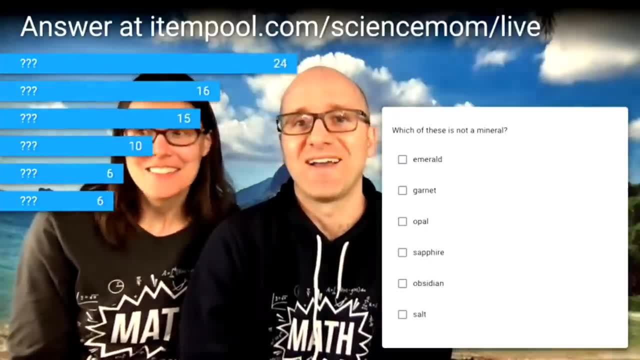 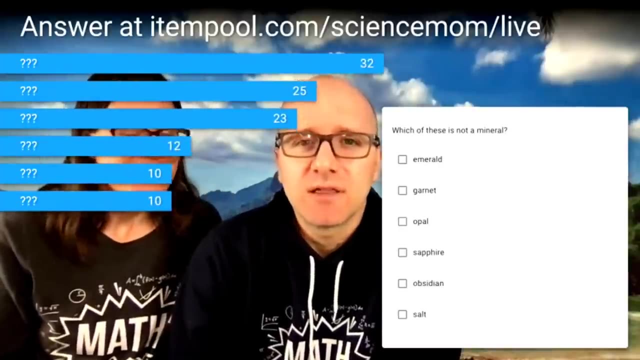 and don't select the ones that are minerals, as you were taught earlier. i just thought that was a good one. i know it's from the moderators. we also have a birthday to natalia. happy birthday today. hey, yeah, creative koala. great, lots of birthdays. all right, i'm seeing three categories get a lot of votes. 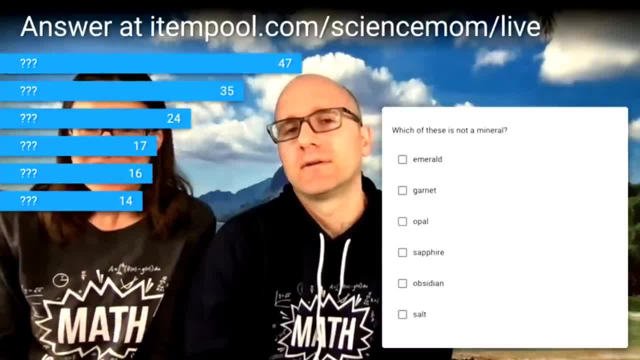 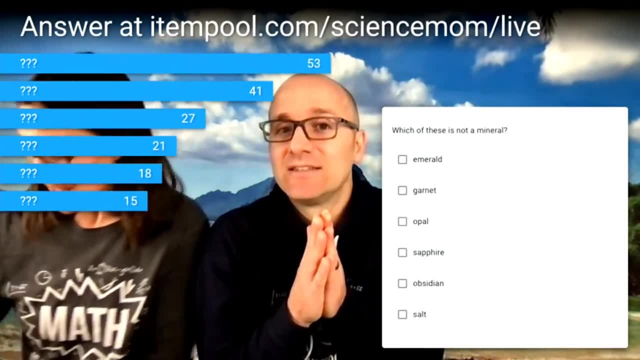 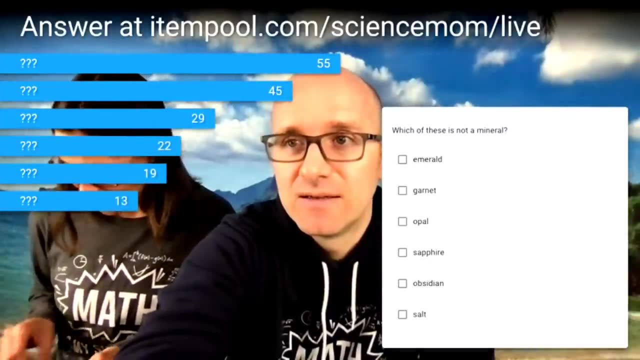 one- one's in the lead, i'm not sure- interesting. hmm, so we have- maybe are they all- minerals, emeralds, garnets, opal, sapphire, obsidian, most sand made out of quartz, but I actually have here a sample of sand that is made out of garnets. 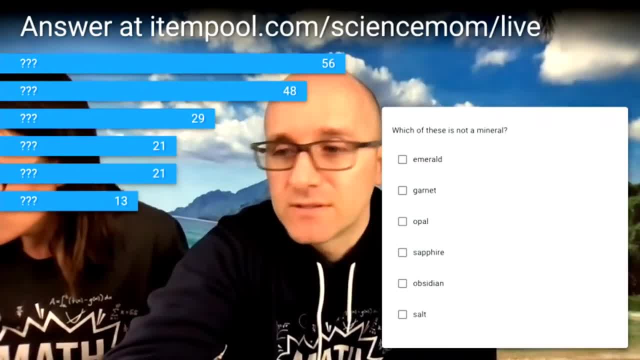 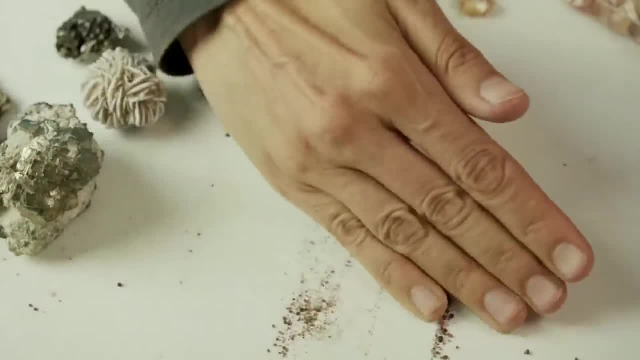 Sorry, All right, I'm doing this. Oh, you want me to show that? Yeah, real fast. So this sand- oops, I put it too far. This sand is from near Washington and Oregon. A geologist friend of mine collected it. 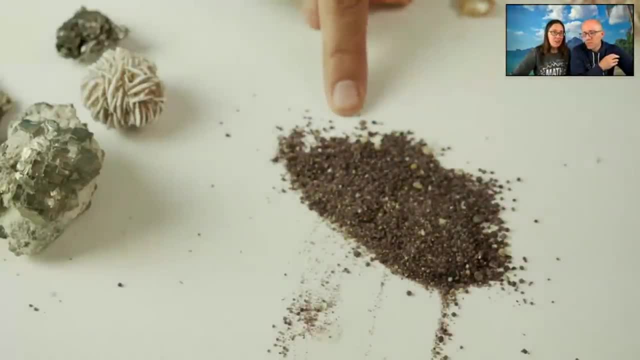 and all of that. each of that is garnet, But- and garnet is a precious gem, but these pieces are so small you couldn't cut them into a gemstone. No, Isn't that neat though? No, that is neat. 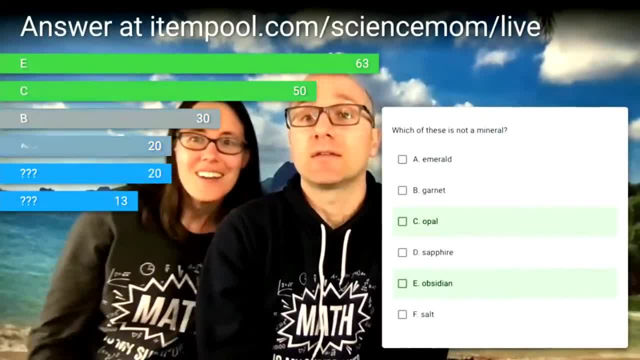 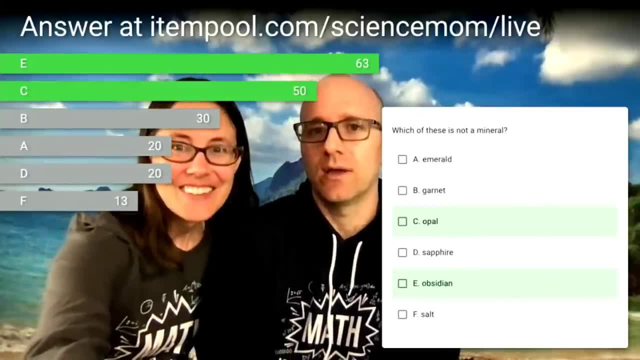 And it looks kind of purple, All right, And so the answers were obsidian and opal. So there were several that picked other things. So emeralds are minerals, garnets are minerals, sapphires are minerals and salt is a mineral. 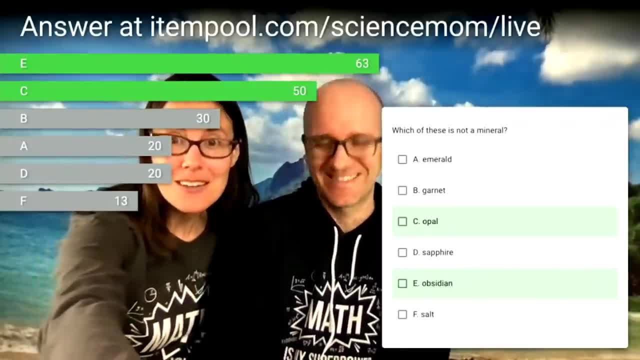 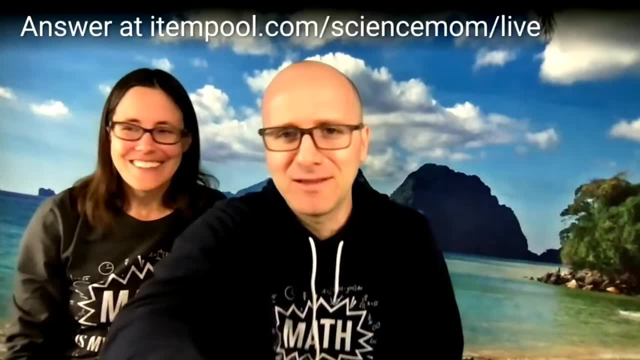 I am so happy to see that salt didn't get as many votes, because you guys were listening. salt is a mineral, That's right, okay, So I didn't stump them that time, although I did get several people to pick incorrect answers. 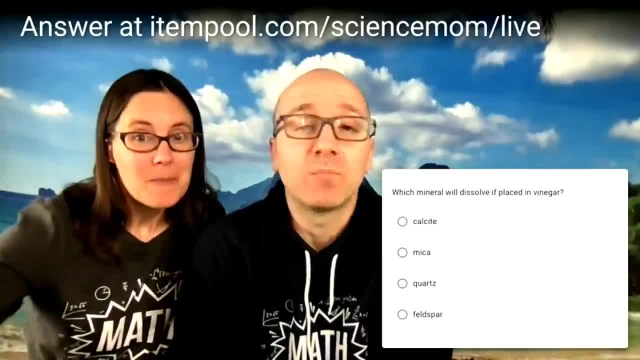 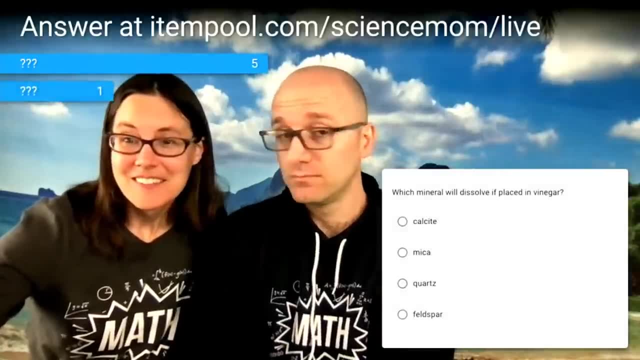 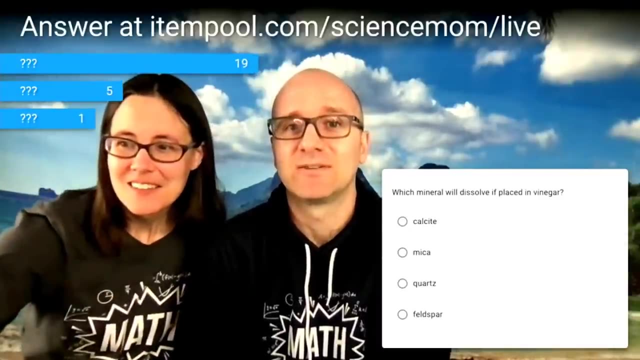 Question three: Which mineral will dissolve if placed in vinegar? We've got calcite, mica, quartz, feldspar. One of these will definitely dissolve and the others will not. Ooh oh man, Isaac had a great question about our rock salt. 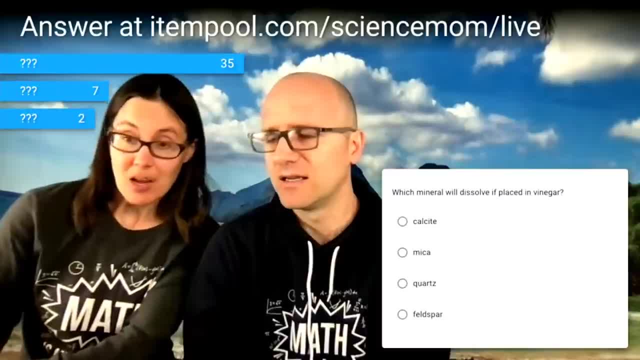 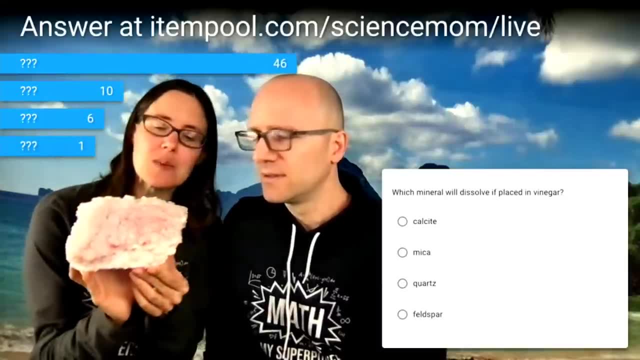 Why is it pink? And I believe it is, but I would have to double check this to be 100% sure. I believe it's because there are trace amounts of iron in the lake, And I think that's what gives it its pink color. 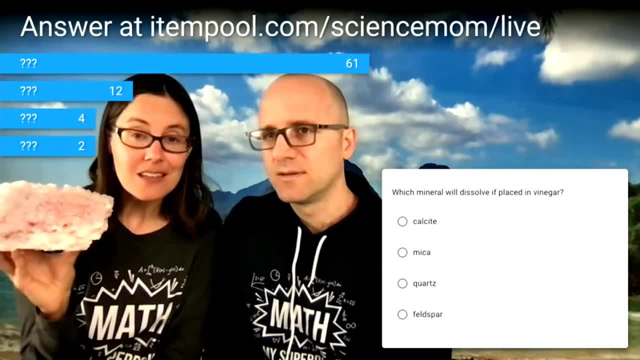 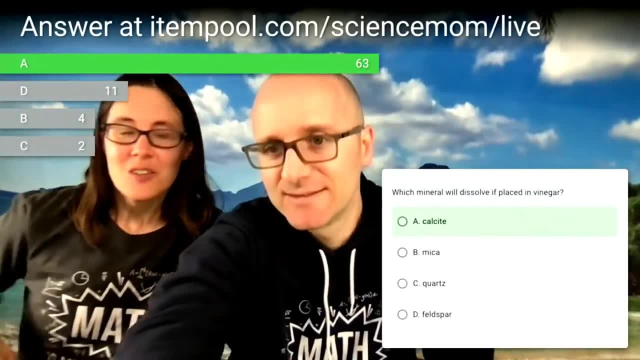 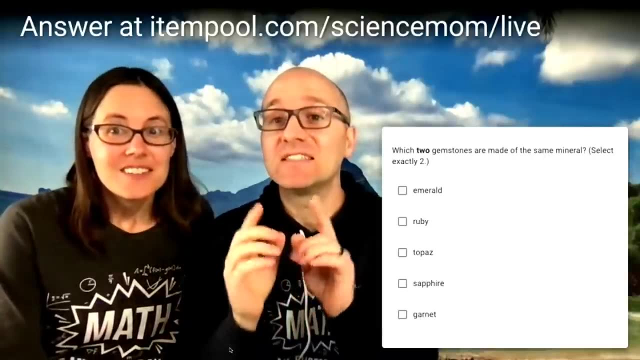 And some halite is pink and some halite is not. You'll find this in different colors depending on where it's formed. Cool, All right. the answer is calcite. Well done, well done. Okay. which two gemstones are made of the same mineral? 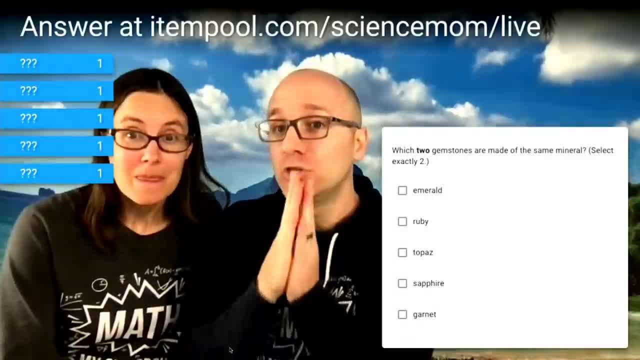 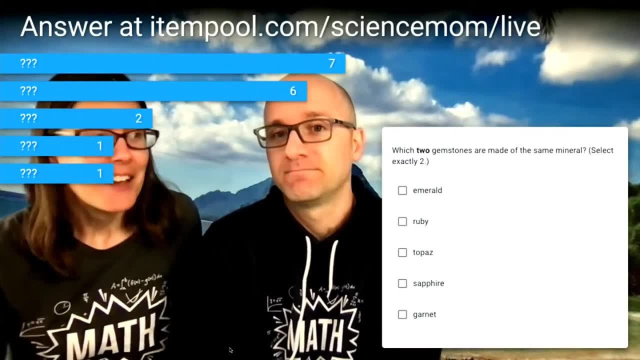 So, in particular, of the options listed below, two of them are made from the same mineral. I want you to select those two and don't select any others. The exact same mineral. I want you to select only pick two. Another great question from Pickle Obsessed. Can you make rocks at home with salt? You can definitely make salt crystals at home just by making a salt solution and then putting a string or something that the mineral can form in and letting the water evaporate and salt crystals will form And they will have the similar cubic structure as they form. 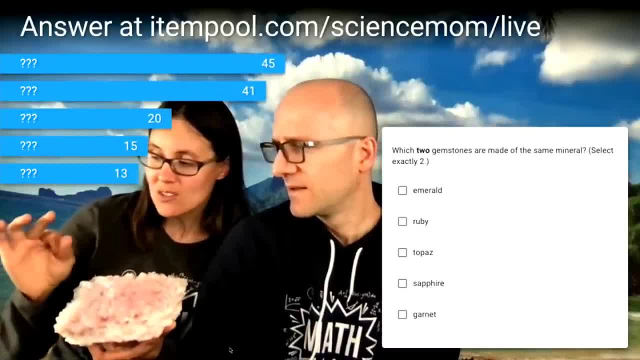 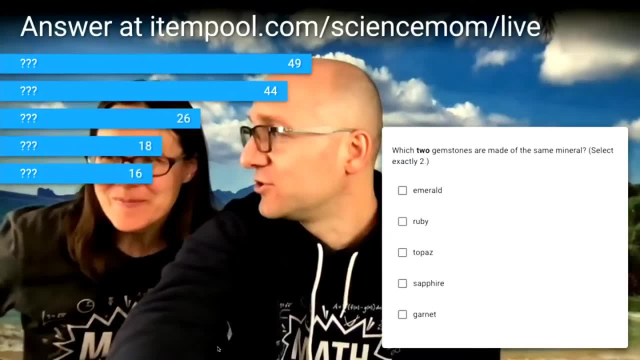 Getting them to grow as big as this, though, is challenging. The biggest salt crystal I've ever grown at home was about that big, And I was so proud of myself. We'll put it on your tombstone: Sansa Once grew a salt crystal that big. 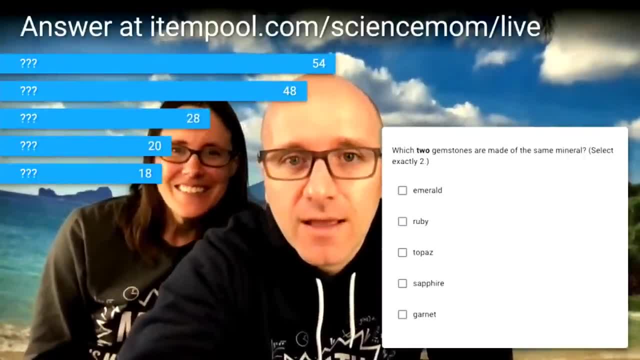 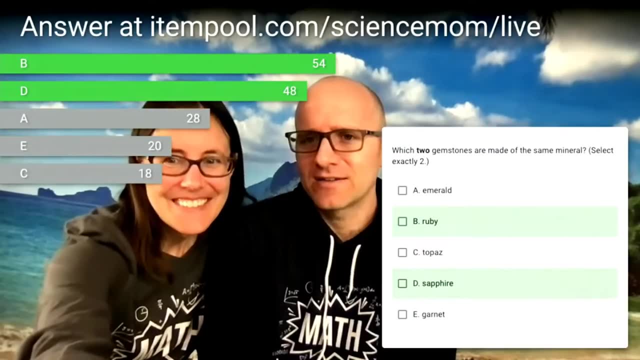 It was about the size of a large pea, All right, And Chessa's ruby and sapphire. That is correct. That's so cool that rubies and sapphires are made from the same mineral: They are Corundum. 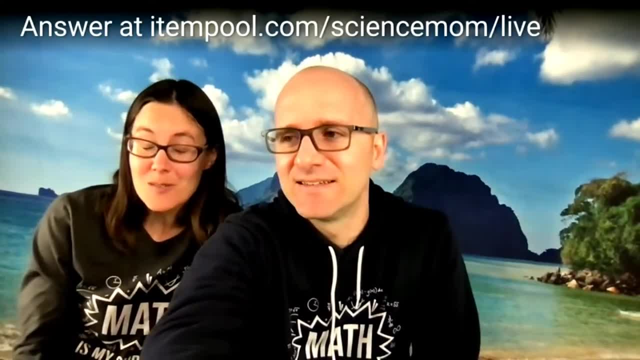 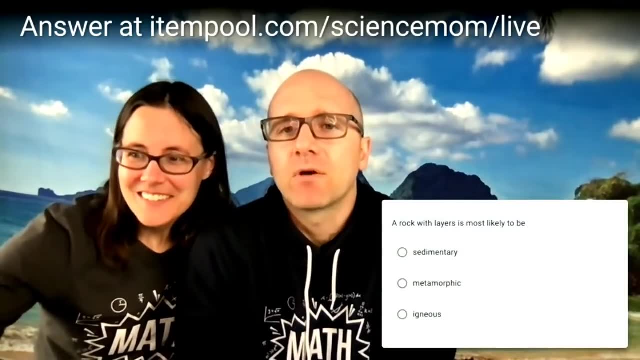 Corundum, And corundum is next down from diamond. Corundum is very hard on that mineral hardness scale. These precious gemstones are typically gonna be pretty high on that scale. All right, Question five: A rock with layers is most likely to be sedimentary. 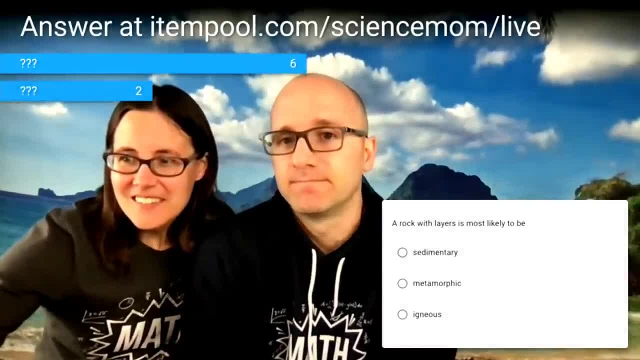 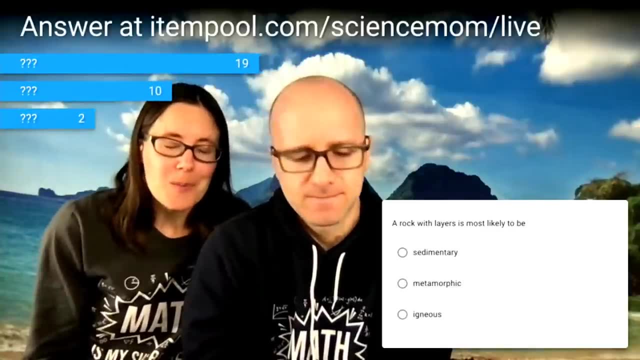 metamorphic or igneous. Which will it be? Isabel had a really great question: Can any rock be a gemstone Like? how does a rock become a gemstone? And this reminds me of the question: what's the difference between a weed and a flower? 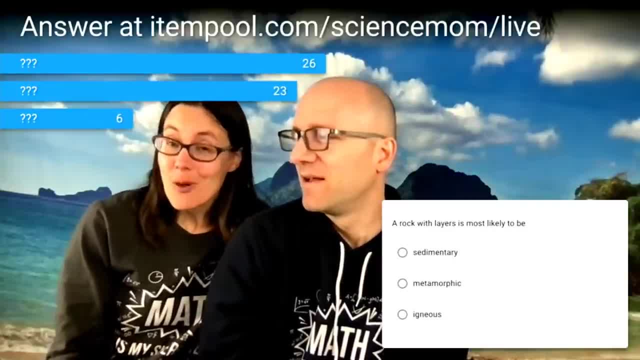 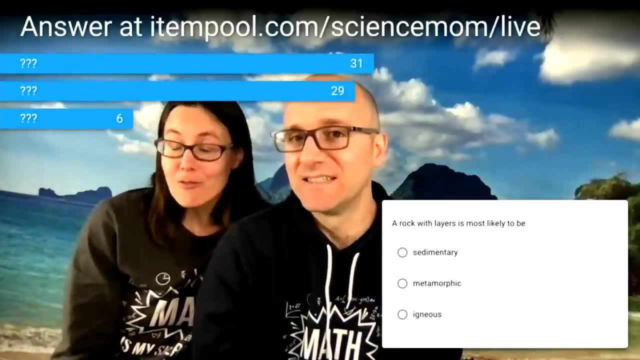 And it really all depends on like: well, what do you want in your garden? If you have a garden and you're growing carrots and then you have geraniums, get into where you want carrots to be growing. the geraniums would be a weed. But if you have a flower garden and carrots started growing in your flower garden, 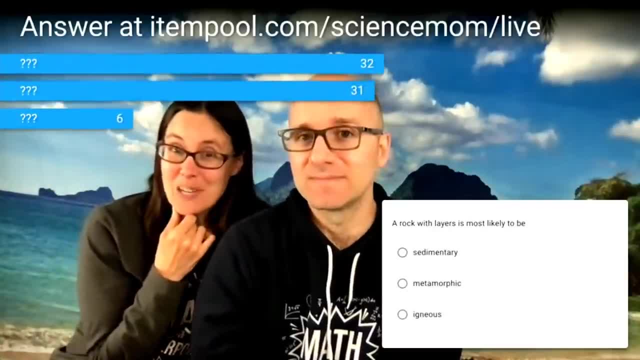 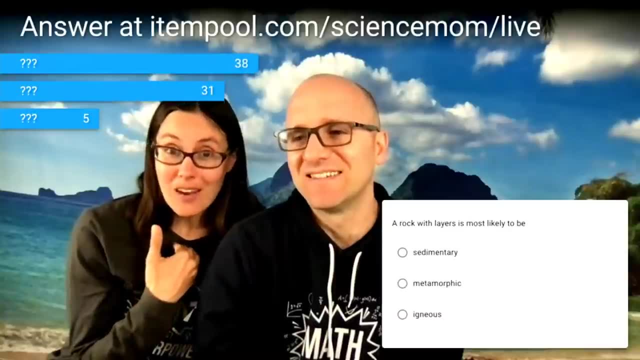 you'd pull the carrots, The carrots would be a weed. So with gemstone it's very subjective. It depends on just minerals that look pretty, that we value. And then you saw that there were some things that are not minerals, that can be called gems, like pearl and amber. So I'd say 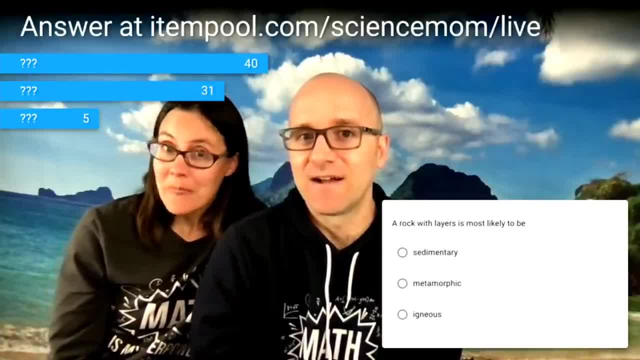 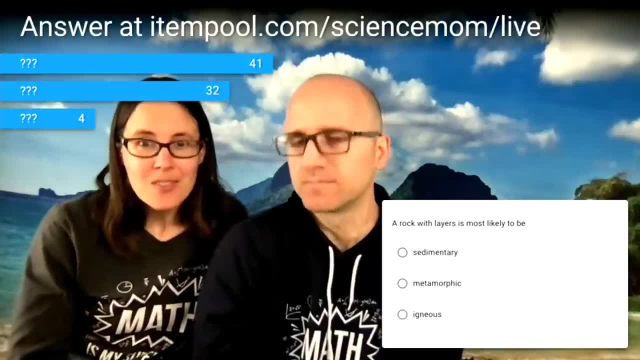 that most things that are gemstones. they are shiny, They can be cut into facets And that's like that classic diamond shape where it reflects the light. Those are the qualities that most gemstones have. Yeah, I like that question. Oh man, this was really close for a minute, but then. 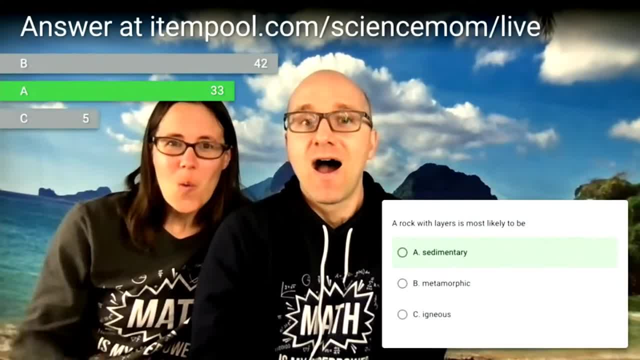 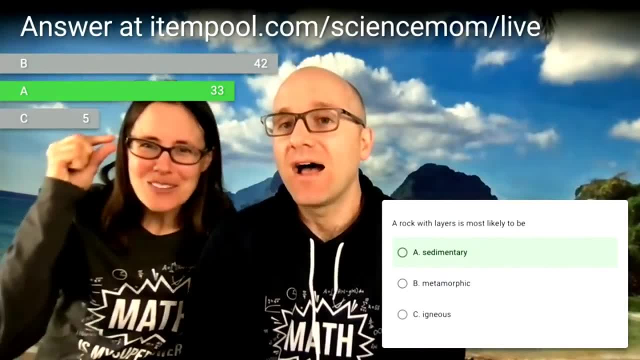 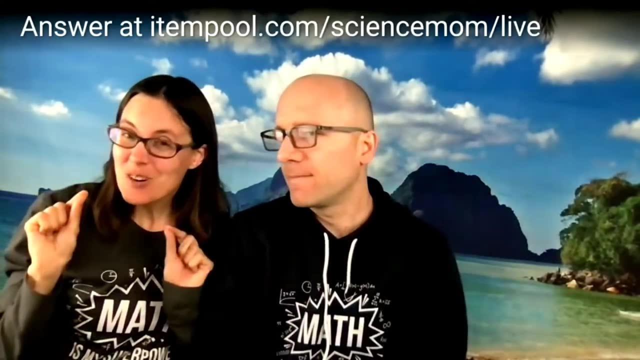 we have one. take the lead. Oh man, Math Dad, are you so excited? Oh, I stumped them Just barely. So the sedimentary rocks. you're going to be able to see these layers in better Usually, But this question comes with a bit of an asterisk. because it all depends. So usually a rock with layers will be sedimentary, but metamorphic rocks can often have layers too, And that's what we saw with our piece of nice. There were some layers in this, and this is a metamorphic rock. Okay, So that one wasn't so cut and dry. 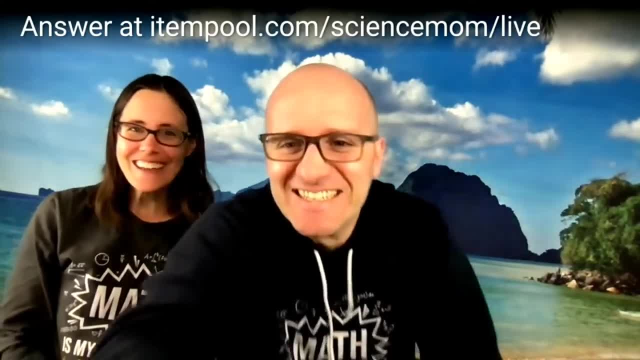 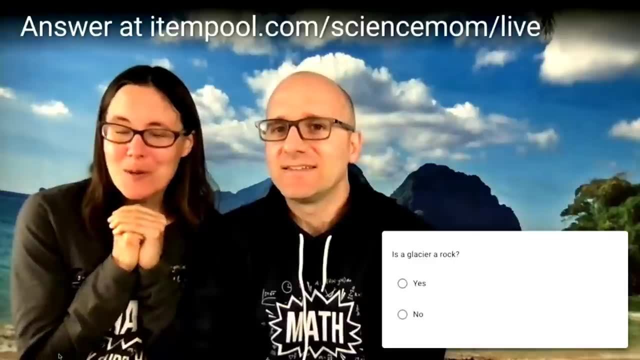 We'll still let you have your victory. Math Dad, Take that All right, And we have a bonus question here. Oh, I love this question. I'm really curious. I purposely didn't talk about this too much because I wanted to see what you guys. 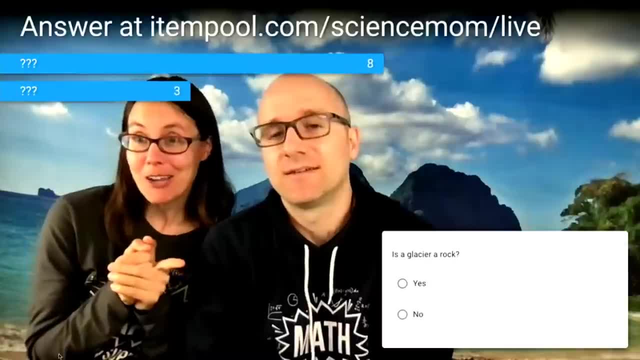 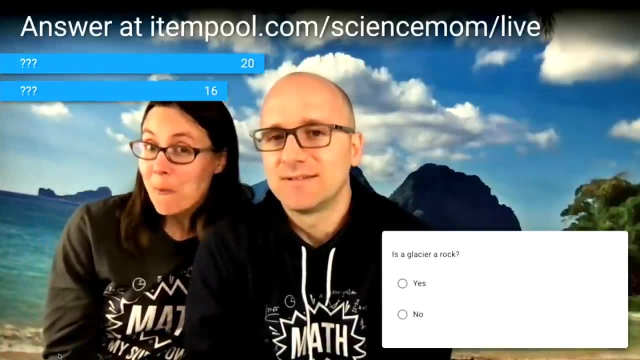 thought Is a glacier a rock, Is a glacier, a rock. And remember, a rock has to be naturally occurring, It has to be formed from minerals and it has to be solid. So is a glacier a rock. What do you think? Oh man, It's almost died. It's almost died. 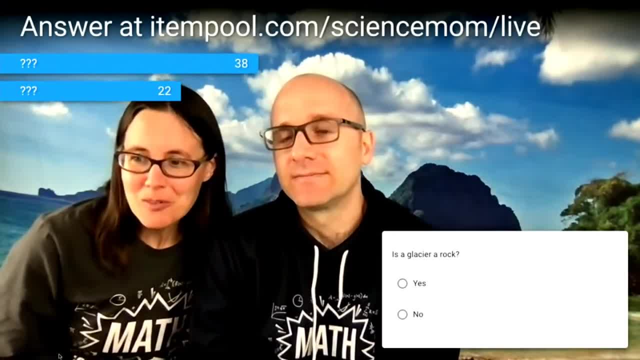 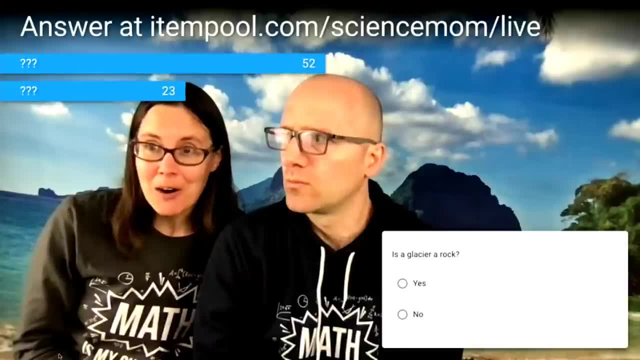 Glaciers were not on your chart. They were not. Ooh. Remington Wolf asked a good question: How hard are teeth on the Moh scale? They're hard, Harder than fingernails, but I'm not exactly sure how hard. I wouldn't want to test it by. 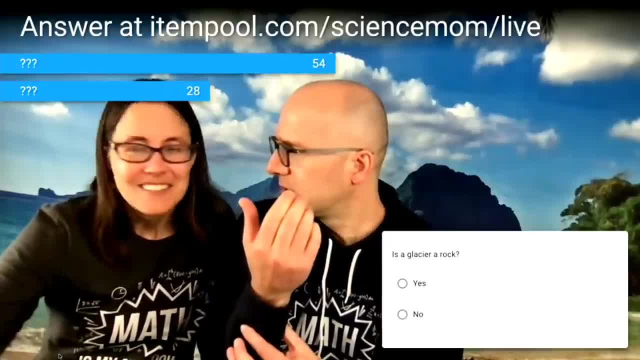 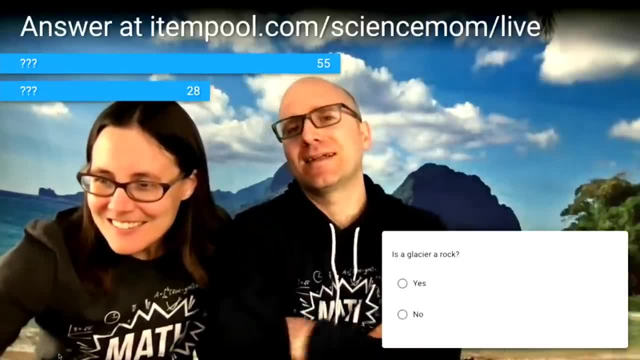 That's a really good question. I think your teeth are stronger than bone, The tooth enamel- That's my understanding. I would have to look it up, but that would be a fun one to look up. Yeah, Really good question. You guys are deep thinkers. I like this. All right, I think it's. 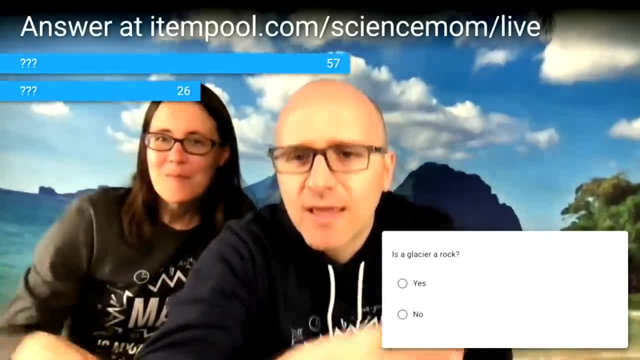 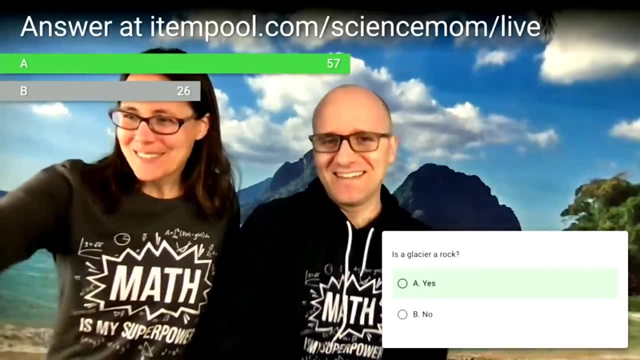 time to call it and reveal the answer. Yes, A glacier is a rock. I can't believe they got that right. So let's go, Let's go back to this view really Fast. I think that deserves, because that last question was kind of a harder one. I think that 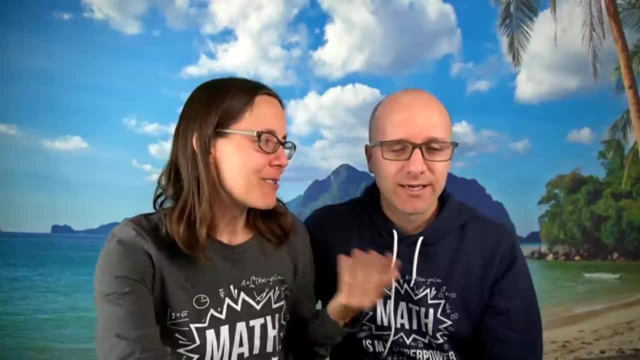 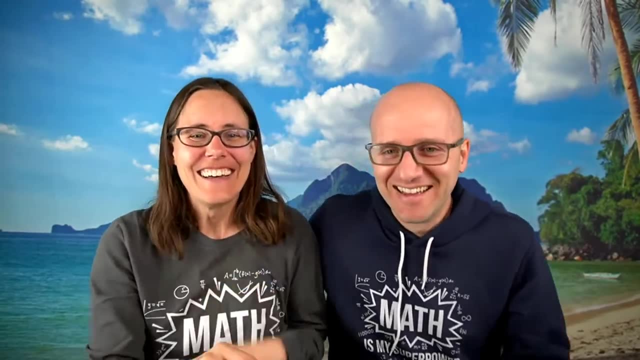 deserves a victory dance. Math Dad, what do you think? Do you want to show them the victory dance you made for yourself? So, Math Dad, One of these days I'm actually going to win, and then I'll show my victory dance. Here's the Math Dad victory dance. 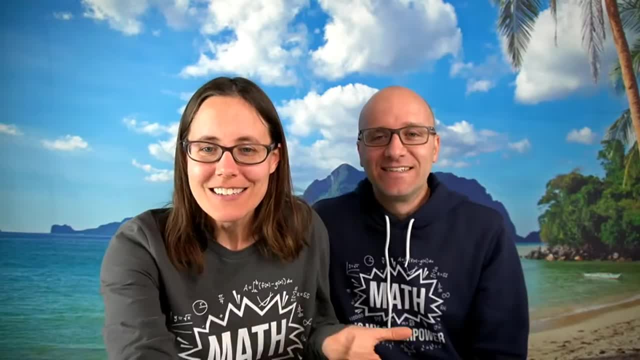 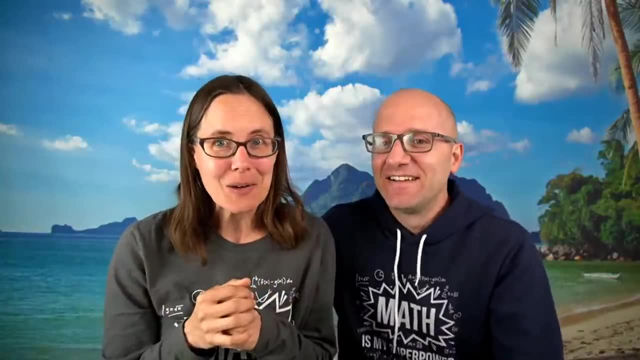 That was the one that he said he was going to play in celebration. So technically, yeah, We'll give you a victory. Math Dad, All right. Is a glacier a rock? This is a question that, if you ask a roomful of geologists, you will actually entertain some lively debate, But most geologists will take 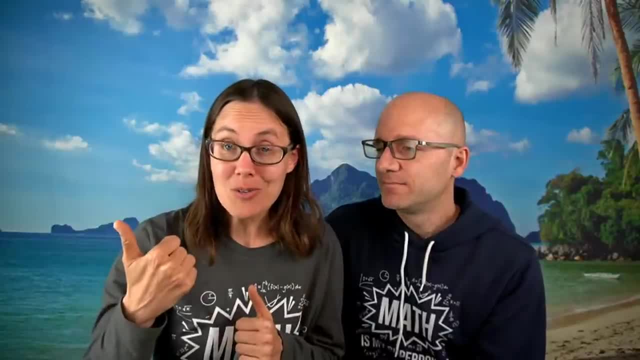 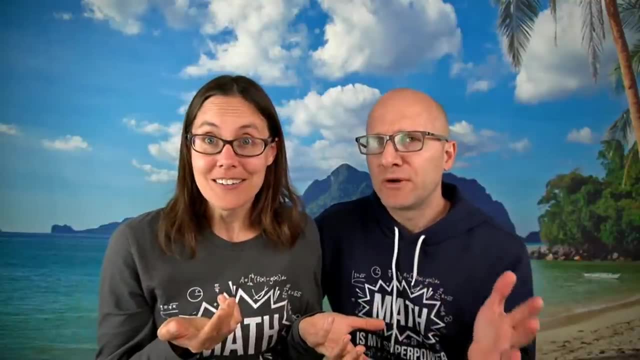 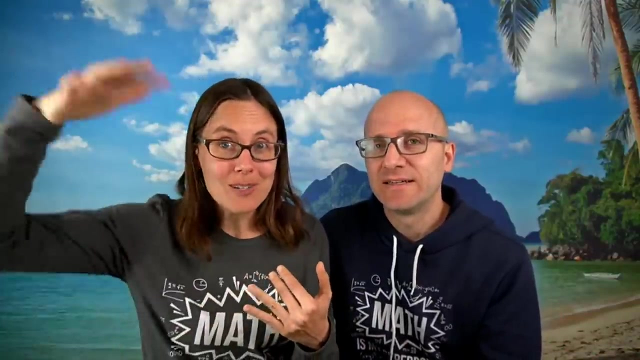 that traditional definition of a rock that we just gave you, that it's naturally occurring and it is made from minerals and it is solid. And so what type of rock is a glacier? Well, what mineral are we referring to here? Water, Yes, So it's made of the mineral ice and it's a sedimentary rock, because you have snow that. 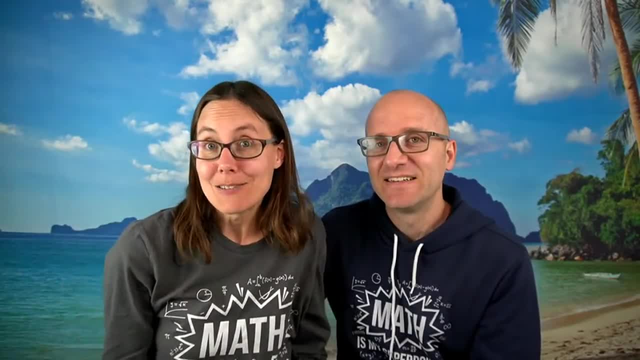 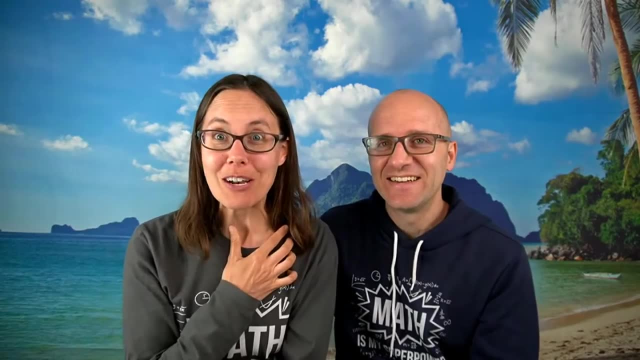 comes and layers together together and compacts the glacier. So most, most people will agree that a glacier is a rock, which means that we live on a world with an ocean of lava, Because water is like the melted form of glacier technically, 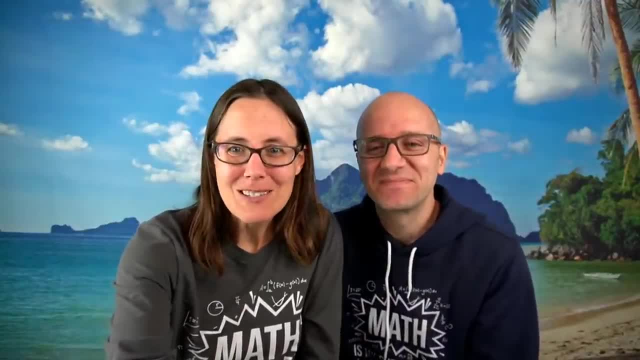 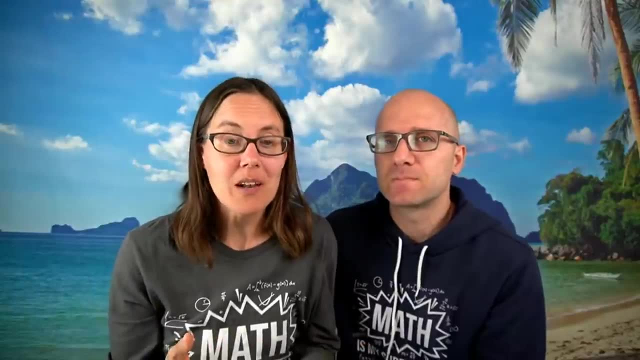 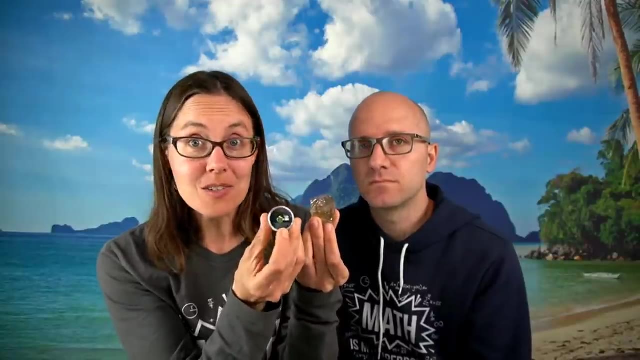 That's kind of funny, Yep. One more question I want to answer real quick before we close. Kelly asked: why would a cut and polished gemstone be so much more money than just a plain gemstone? So, for example, this piece, piece of citrine here when it's cut and polished into a faceted gemstone. 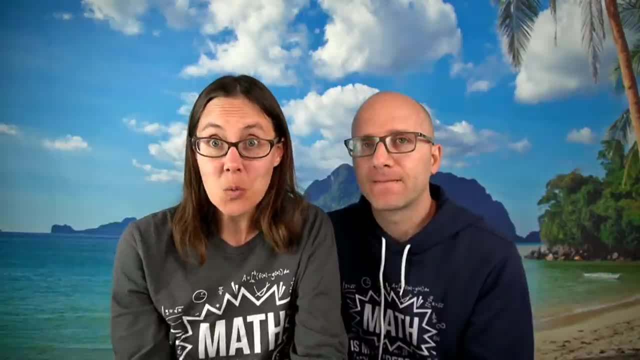 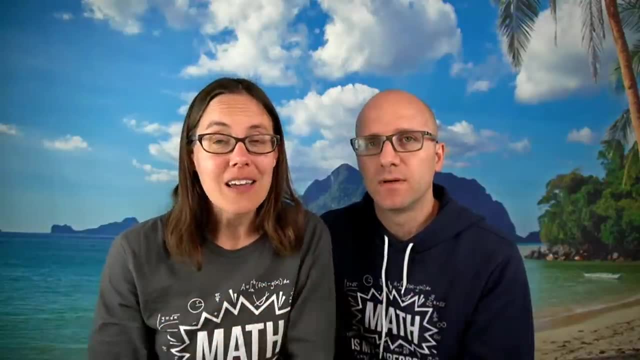 it's much more valuable. Part of that is because it's it takes work to cut and polish a gemstone, And if you do it wrong then you've got to throw that piece of rock away and get another one, And it's it's. it takes a lot of work and skill to be able to cut it. I think a lot of the value of gemstones is just: it's been inflated by jewelers who want to sell them and, like the diamonds, are actually a way more common than you would expect, based off of the fact that diamond rings cost so much, but the prices have. 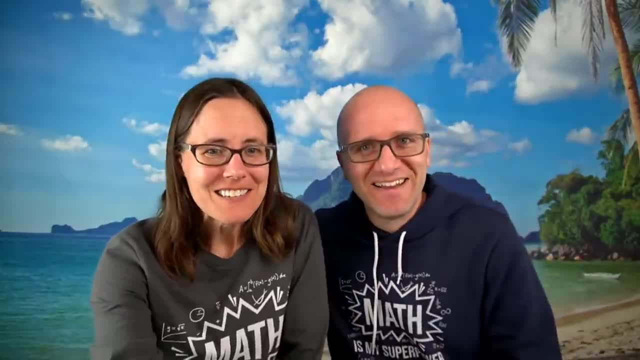 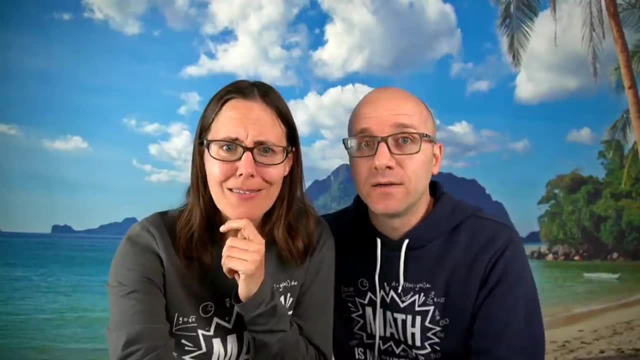 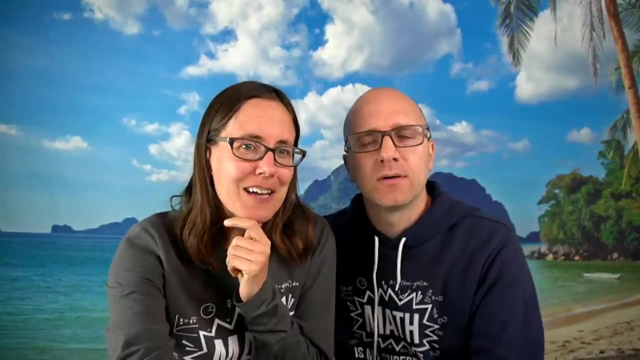 been artificially, somewhat artificially inflated. yes, and two really great questions. i'm going to research and i'll have answers for you on friday. what's the oldest mineral in the solar system? love that question, rosalita. and then, um, what's the rarest rock that someone could get? i would